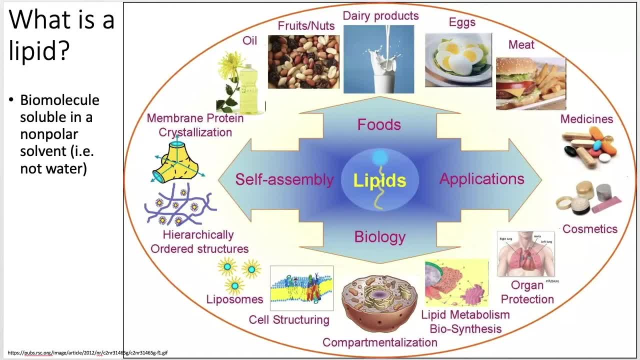 usually we say like to the layperson: which if you start googling this stuff or do google images, you're going to get all these crazy nutritional things and it just gets complicated by the non-scientific community. But a lipid is really just a biomolecule. that 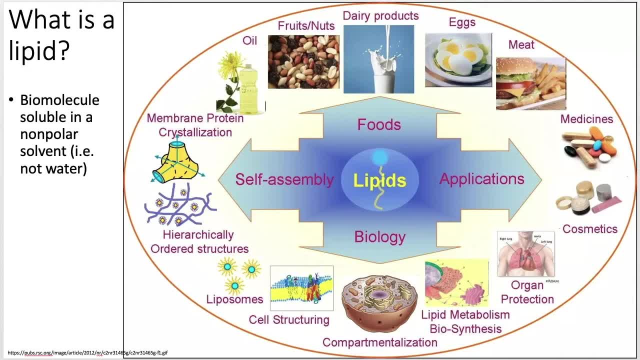 is soluble in a non-polar solvent, ie not water, So they're generally hydrophobic, or at least have a hydrophobic region. Now, of course, when you think lipids, basically what you're thinking of are fats, And so I mean that's foods. they have different abilities and stuff. 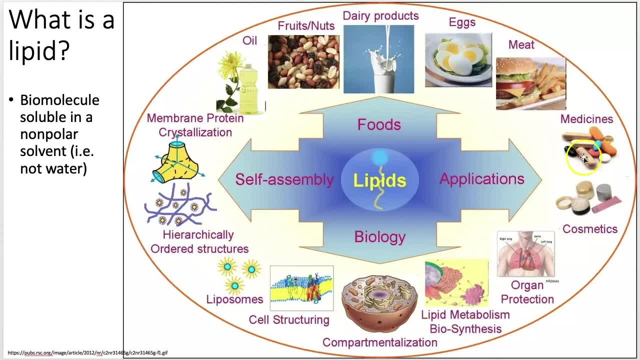 and we're going to talk about mostly this stuff. But they do have a lot of functionalities in like larger scale things like medicines and things. But of course you know, we all know what fats are and stuff like oils and fats And so 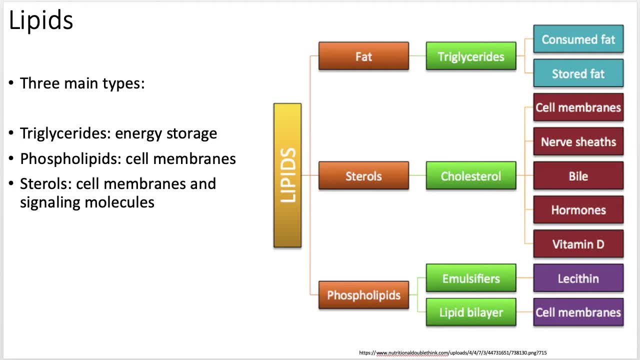 we're going to talk about those today. So there are three main types of lipids that we're going to talk about. So there are triglycerides and in general, that's our energy storage molecule. So we're going to talk about that, And then we're going to talk about phospholipids. 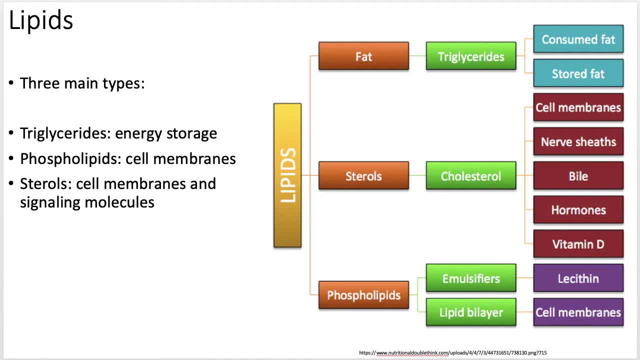 for cell membranes, Just that general structure. we're going to talk about that. There's a ton of variety in there. And then we'll talk a little bit about sterols, which are like your cholesterols or your ergosterols, And those are in cell membranes, but they're also part of signaling. 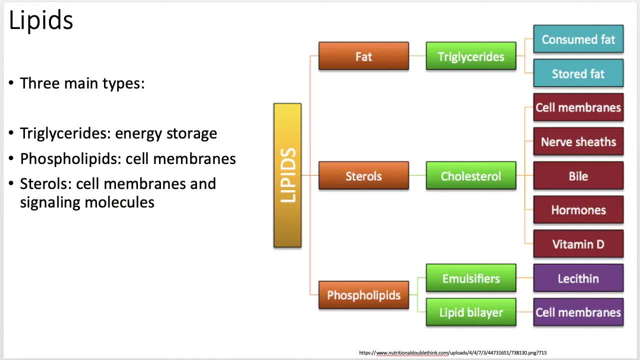 molecules, And it's going to get a little complicated. might be the wrong term, but there's just going to be a lot, because a lot of these things are tied to each other and there's a lot of pathways that cross over, And so I'll try and keep things pretty clear. but let's get in. 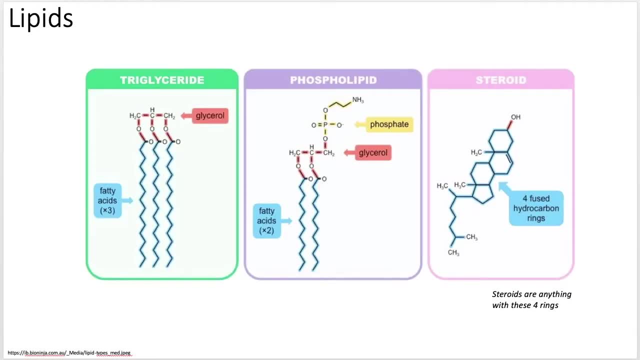 Now, in general, these are our structures that we're dealing with, And why am I showing you this? Because I want you to see the consistencies. So one of the keys to learning fats and lipids and their structures is to look for the consistencies. okay, I say this as somebody who struggled with 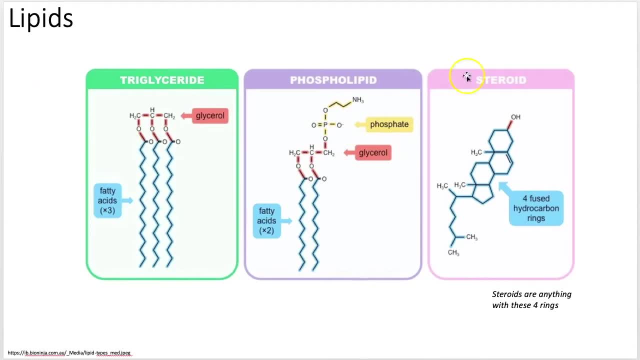 this. So here we've got our three groups again: our triglycerides, our phospholipids and our steroids. okay, So in general, most of the time, cursory examinations of lipids. we'll generally just have these three groups And I want you to see these nice long fatty acid. 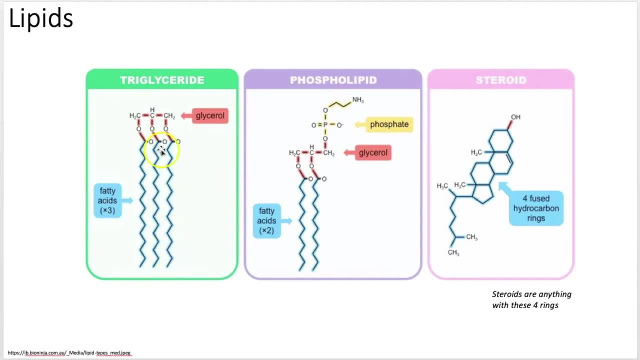 chains, So these are long carbon hydrogen chains. okay. And fatty acids: we're going to spend a lot of time talking about these in a minute, And fatty acids comprise most of your triglycerides and a huge portion of your phospholipids. okay, And so once we understand a lot about fatty acids. 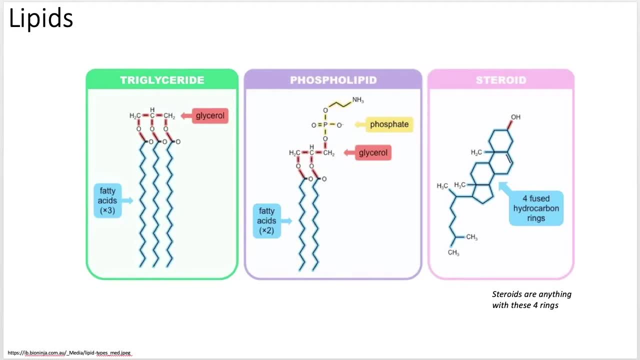 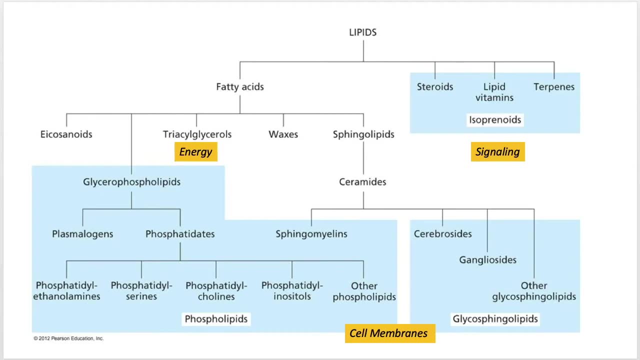 then we can understand a little bit better about triglycerides and phospholipids, hence why we're going to spend a lot of time talking about fatty acids. All right, so just to reiterate, here's another. So, basically, I'm going to slowly expose you to the massive amounts. 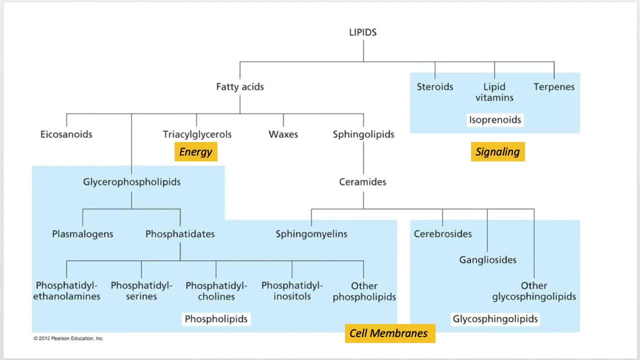 of lipids that exist on this planet. It can be super overwhelming, especially if you're trying to teach people about it. So let's try and break this down a little bit. I mean lipids. I mean everything is encompassed under lipids, Things with fatty acids in them. so I just mentioned 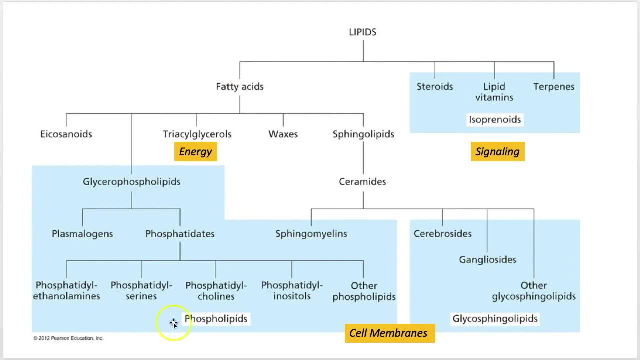 this, okay. So basically we're all of these things down here. we're going to encompass in our phospholipids or our sphingolipids, but we're going to kind of just lump those together in all the things associated with the cell membrane. okay, Now there are other things associated. 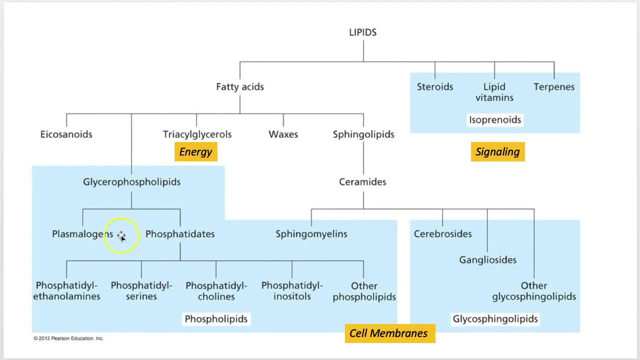 with the cell membrane, of course, but these are going to be the big components. okay, Now triacylglycerols up here. so there's your energy. okay, Now, all of these things can be used energetically, and that's where it gets a little confusing. but what's their primary? 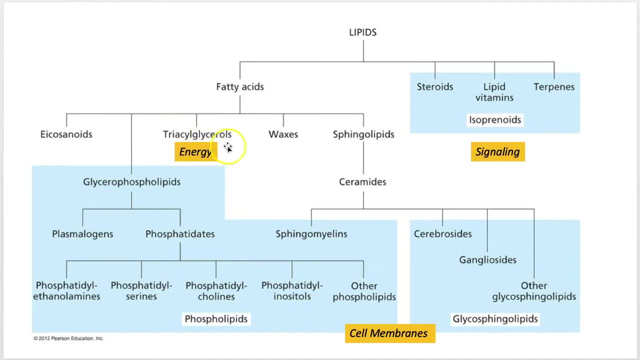 function is what you have to think about, And the primary function of triacylglycerols, or, you know, your triglycerides, is energy, energy storage. okay, Now you do also have some weird ones, your isoprenoids. I think I said that right. Generally, those are going to be: 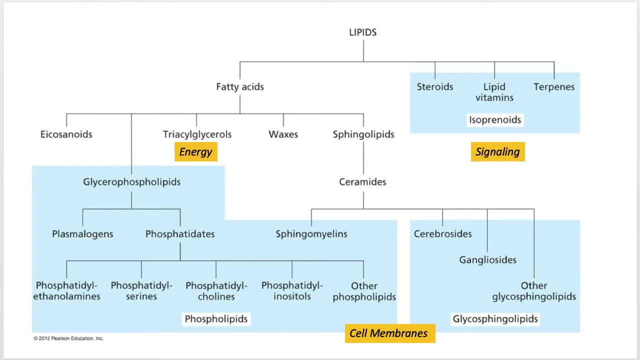 your signaling molecules, though they can have other functions as well. I mean, that's your steroids, your hormones. you can have lipid-based vitamins like vitamin D. I think vitamin A is as well Terpenes, that's like in plants. they'll be like plant-defensive molecules, I mean. 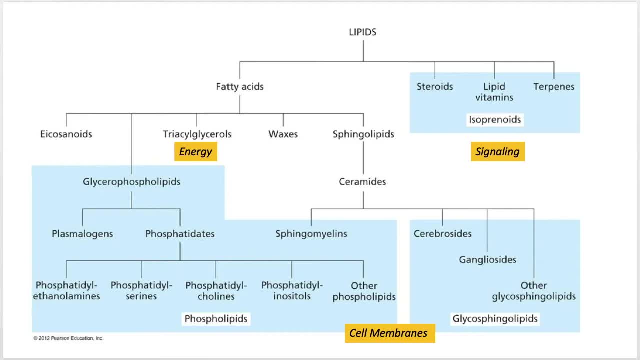 if it's insoluble in water. that's like so many things, and so you can see why it's so many things. So let's kind of break it down and try and just dig a little bit deeper into the specifics and just make it a little simpler. We need to talk about fatty acids. 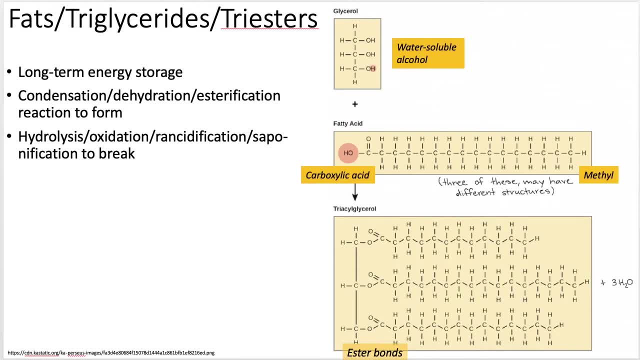 okay, And to get us into fatty acids, we're going to focus on this first structure, our triglycerides, and there's those fatty acids right there. So triglycerides are generally a long-term energy storage molecule. okay, They can have a huge variety, and that variety typically. 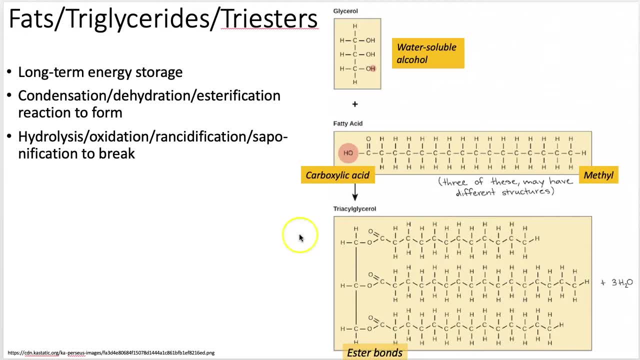 just comes from the length of the fat. So if you have a lot of fat in your body and you're going to have a lot of fat in your body, you're going to have a lot of fat in your body, okay. So 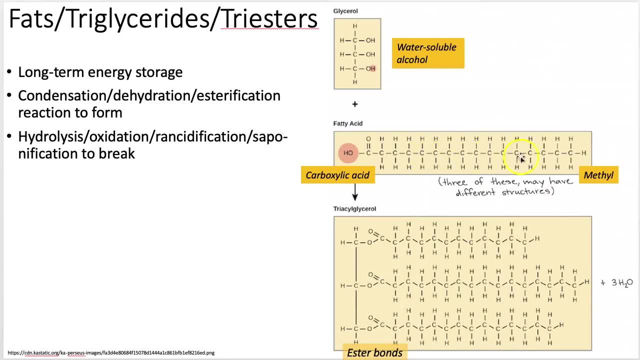 here is your typical fatty acid long carbon chain. This one is a fully hydrogenated, so this would be called a saturated fatty acid. okay, These are actually all saturated fatty acids. We're going to talk about what that means, And what you're going to do is you're going to 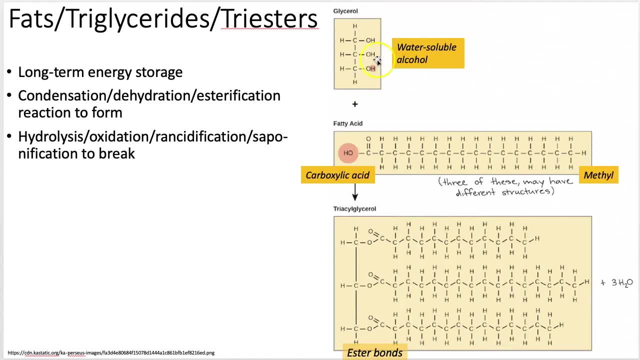 take a glycerol molecule, which is a water-soluble alcohol- okay, lots of alcohol groups- and you're going to have a condensation reaction, which is a dehydration reaction- Hence you can call it a glycerol reaction. And you're going to take a glycerol molecule which is a 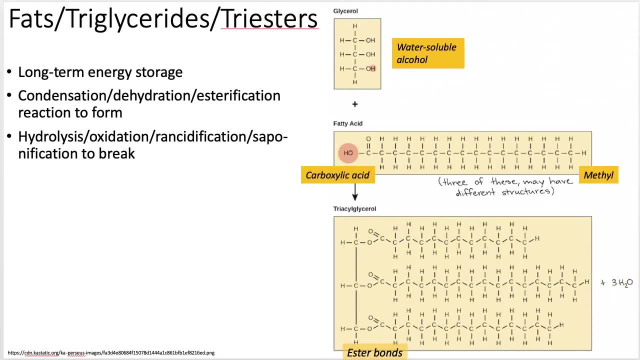 get water out with one, two or three fatty acids. Now in general we refer to three of them. okay, It's a triglyceride. It's also called a triester. That would be a more generic term for. 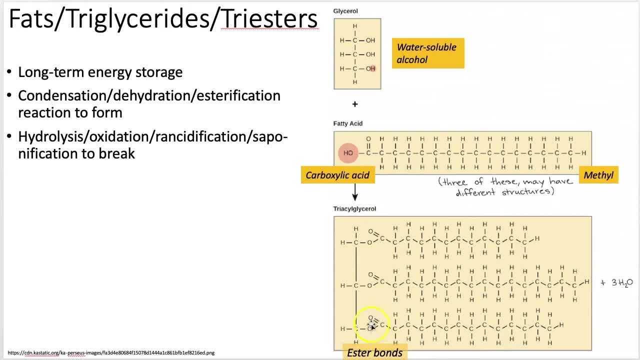 it because there are three ester bonds. okay, So we've got our ester bonding here. We've got our carbon with a carboxylic acid, and then we've got another carbon chain going this way, and then oxygen, and then another carbon chain, And so that's an ester, And so you have three ester bonds. 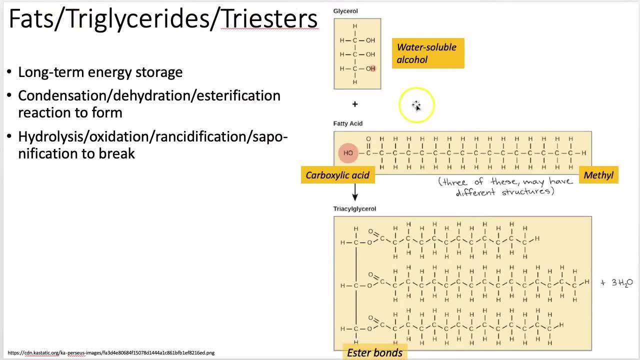 hence triester Triglyceride, meaning that we have our glycerol group with three fatty acids sticking off of it. Important to note: your fatty acid will always have a carboxylic acid on one end and a methyl group terminating it on the other end. Now, yes, it's a bunch of carbons, okay, But 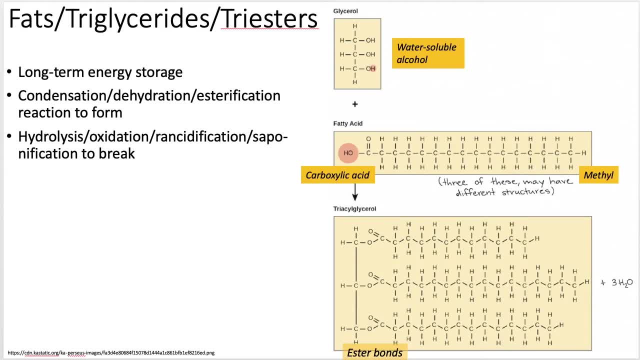 at the very end. it's technically a methyl group And so that's your typical fatty acid. Length obviously can change. We're going to talk a little bit about structure- and I'm second- and the presence of bonds, double bonds, Sorry, I was going to say dibonds. What? 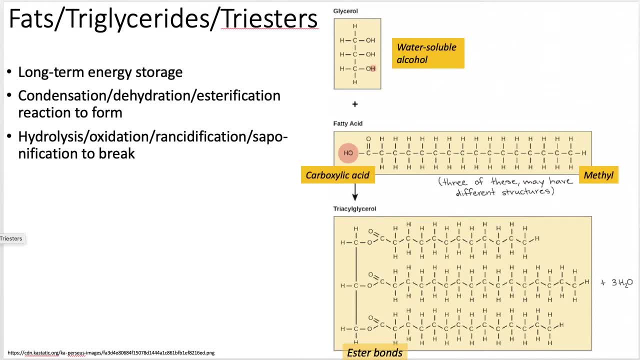 Now, if you want to go backwards- which of course you can go backwards- If you need to build these, then you need to break them down, too, right? So if you're going to get the energy back out- And that's hydrolysis or it's also oxidation- Oxidation is generally what we call it when we're 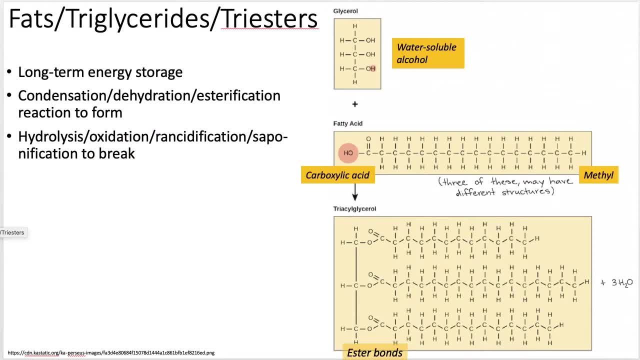 breaking things down. right, We're pulling electrons away, okay, So we're oxidized, We're making a compound and then reducing another compound, okay, And so if we're making it as condensation, dehydration, I guess you could say a reduction as well, An esterification, right, Because 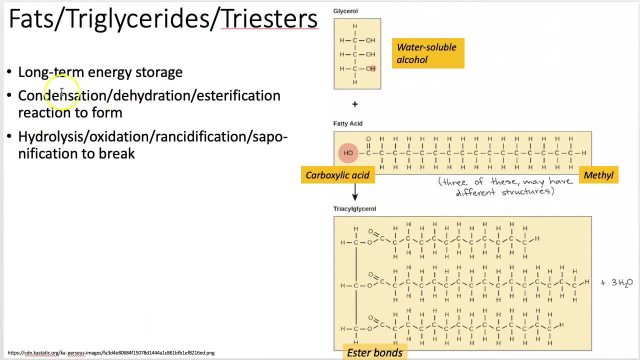 we're forming an ester, But for the most part we usually call these condensation reactions. If we're going the other way, it's an oxidation, It's a hydrolysis, because we're going to use water, because that's generally what our solute, not our solute, our solvent- sorry, Even though. 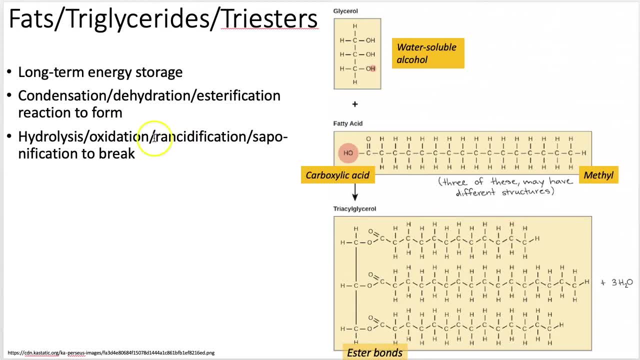 obviously these are insoluble in water. But there are a couple other terms. I just want to hit: Rancidification, So that's when you have spontaneous oxidation of your bonds, And so that's when, like, if you leave. I'm trying to think of a good example, Like: 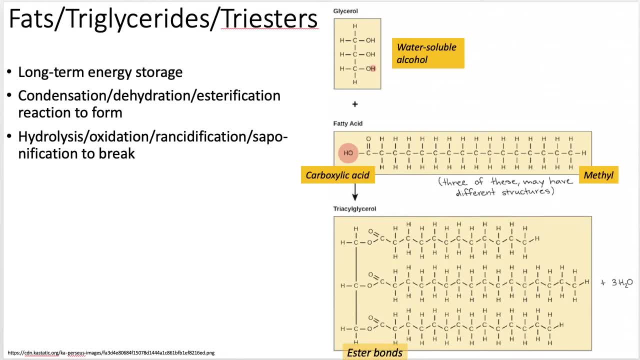 if you leave butter sitting out and it starts to stink, it's gone rancid, right, And that's actually a technical term, I guess, arguably technical. Aren't these all technical terms For a oxidation reaction right? Spontaneous oxidation or partial oxidation of these fatty? 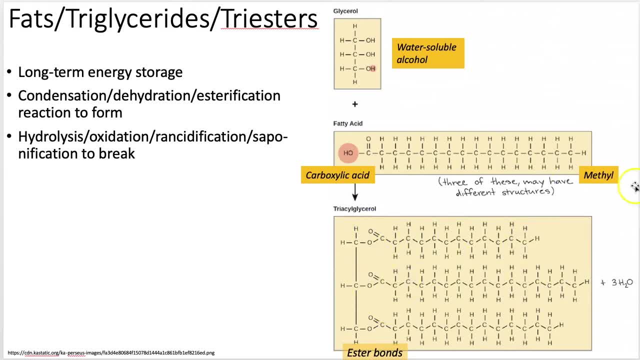 acids, So you can have one of these or two of these. And fatty acids can have really complex structures. Let me rephrase that They can have really long twisty structures. Sometimes they can be complex. I guess it depends on how you define complexity. But, and some of those molecules 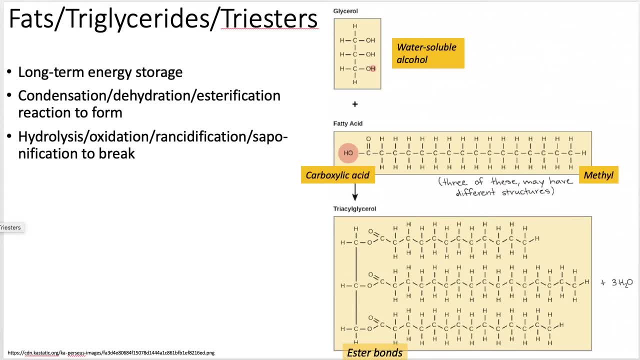 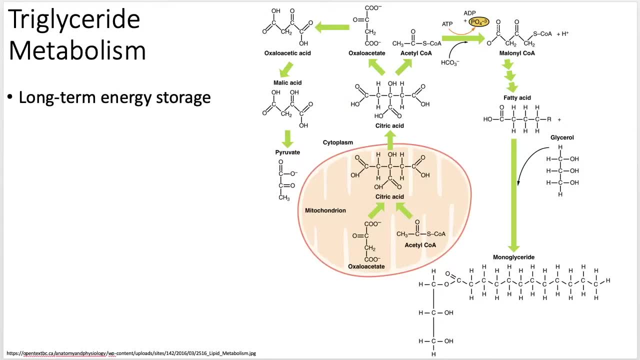 that fall off can smell bad. So yeah, And then we're going to talk about saponification in a second. That's how we make soap, which seemed kind of cool, So I thought we could talk about that Now to actually metabolize. So either, this one's talking about how to make it. 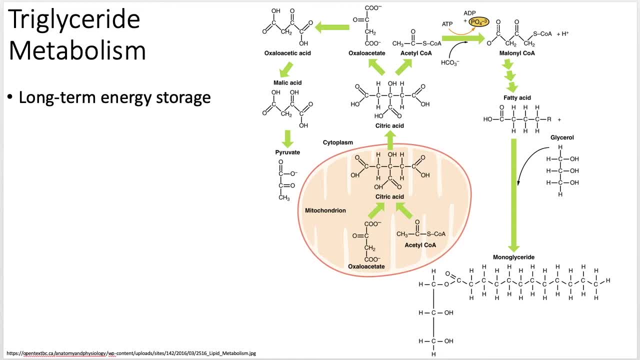 But to break it down would be similar like reverse pathways, But basically if you're going to generate triglycerides or monoglycerides, in this case the actual pathways are really, really similar. So we're going to see a lot of these consistent between either glycolysis, Okay, 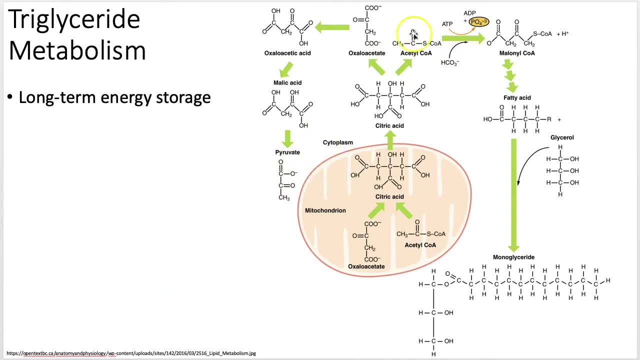 So there's pyruvate, which would come from glycolysis. You could argue that acetyl-CoA could come out of glycolysis. It's sort of the intermediate step between glycolysis and citric acid cycle, And then a lot of these, So there's acetyl-CoA again. 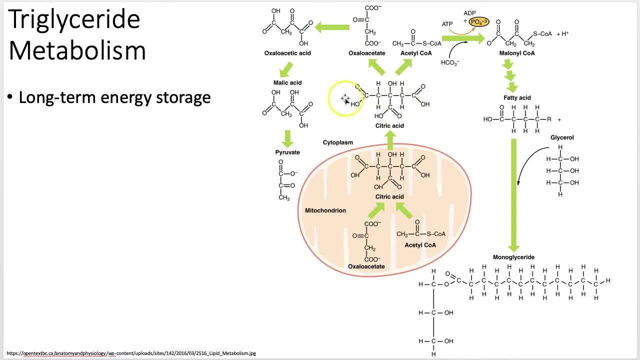 Then oxaloacetate and citric acid. These come from the citric acid cycle themselves. They're intermediates And so- something important, as we actually start digging into these deeper pathways, ie glycolysis or citric acid cycle, we're going to follow those cycles, So we'll learn all the 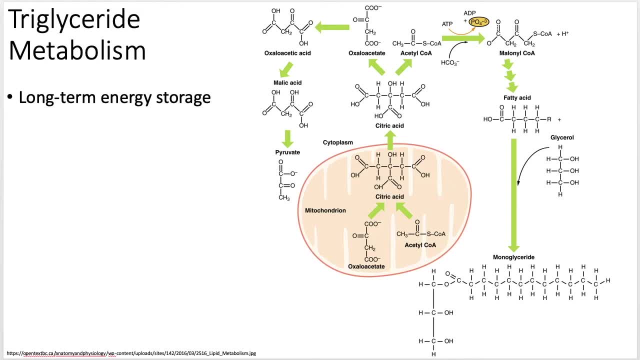 steps of the citric acid cycle. But you can pull intermediates of the citric acid cycle out of that cycle and use them to do other things, And that's a really important idea to understand, But it's pretty straightforward. Honestly, you're going to take your glycerol here. There's your glycerol. 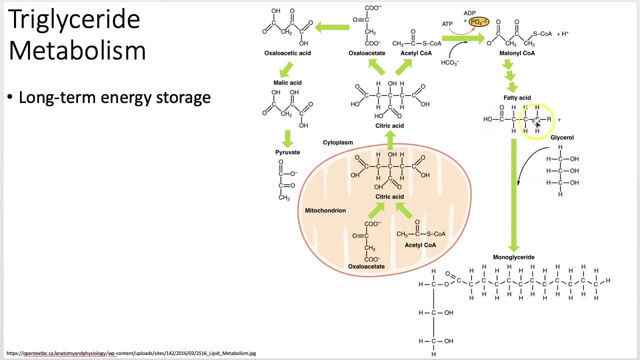 And we're going to mash it together with a fatty acid. So they're implying that you have to have at least three carbons, but whatever. And then you're going to go down. You can have less than three, But you're going to then perform an esterification and generate, in this case, 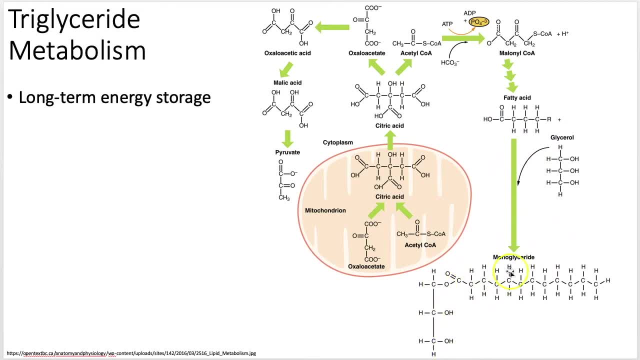 a monoglyceride. But then you've got these two nice open groups. Now they're showing it this way, because you could actually generate a phospholipid this way, by only having one fatty acid or maybe just two fatty acid chains, And then you're going to have a monoglyceride And then you're. 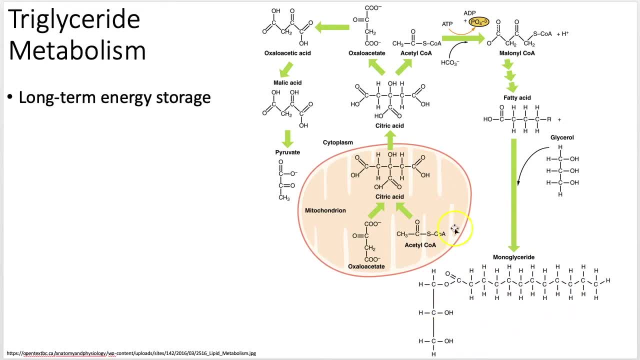 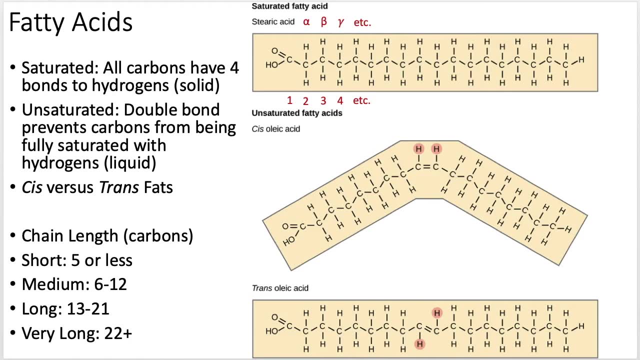 leaving the other one open to bond with other things. So that's why this picture itself is called just showing monoglycerides. So let's talk a little bit about fatty acids. So big, long carbon chains, Pretty straightforward structure. honestly, I mean, you have your. 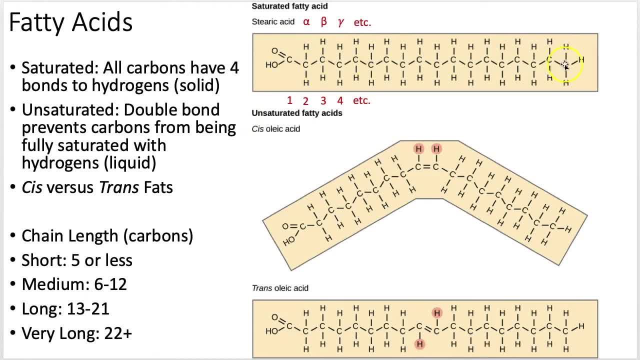 carboxylic acid on the end here and just a bunch of carbons. But you could do other stuff, Like you could have a double bond in there, You could have a couple double bonds, And so let's talk a little bit about that. So saturation is probably something that you've heard of. 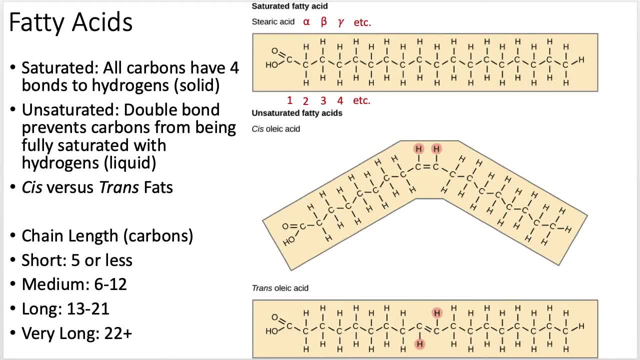 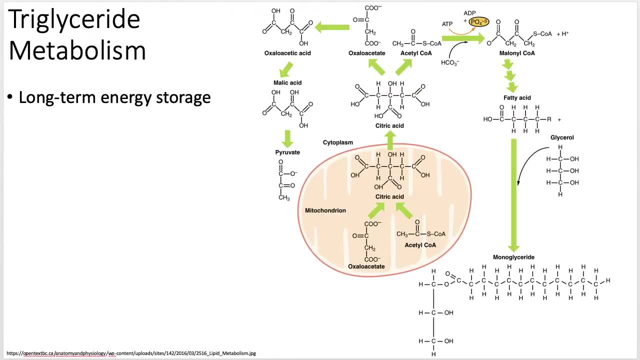 Hydrogenation, or like partially hydrogenated soybean oil, or saturated fats versus unsaturated fats. Those are all just different versions of fatty acids, And so it's always referring to this fatty acid chain, which, of course, you can have your triglycerides, which are made of fatty. 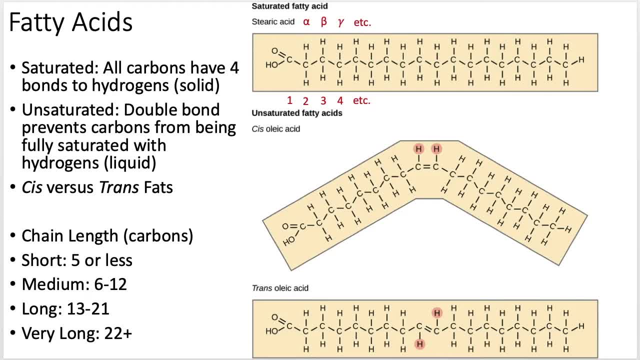 acid chains, And so you can have a variety of fatty acids in your triglycerides. And so when we say saturated, that just means that all your carbons are full up with hydrogens. okay, Now to actually do that we 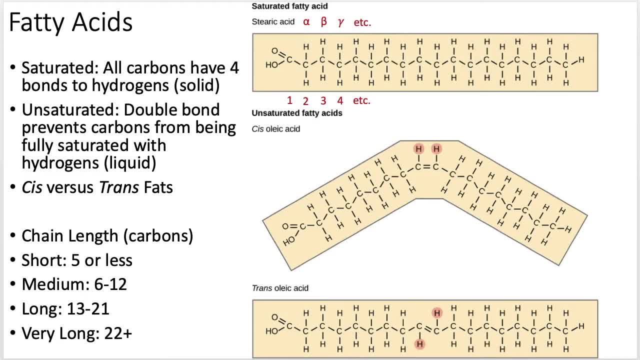 use a process called hydrogenation And I'm going to have a little video in a second that talks a little bit about that as well as a slide. Unsaturated is when you get double bonds And so naturally occurring double bonds. well, double bonds can exist either in a cis configuration. 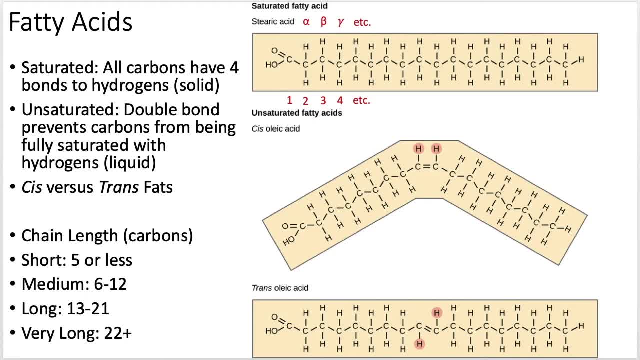 or a trans configuration. So are they on the same side of the? are the hydrogens on the same side or are they on opposite sides? So cis versus trans. So in this case this would be a cis version of a fatty acid, Now in general, not in general trans fats. okay, So trans fats down. 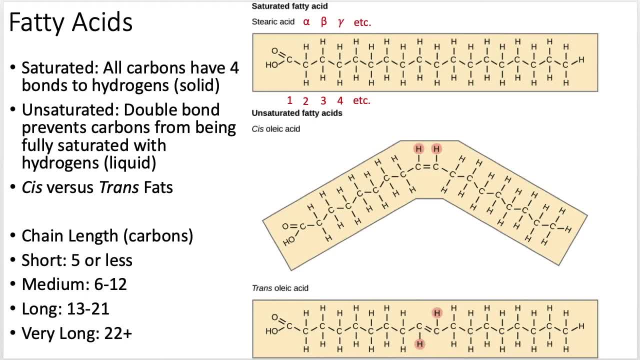 here. those are unnatural, Those are man-made fats. Now you can eat them and you can break them down. However, cis fats are generally what get created in living systems. okay, Now you can. you can get some trans fats in, like certain animal fats that occur naturally, But for the 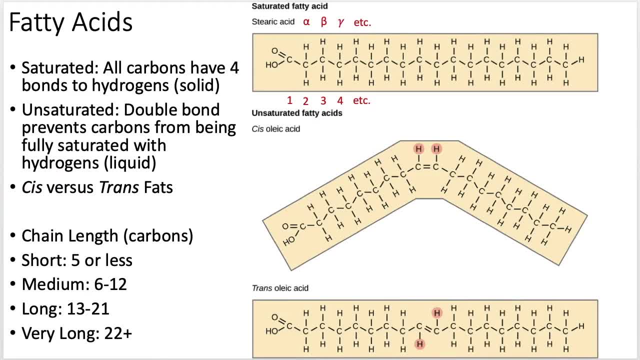 most part, cis fats are what occur naturally. As a nice generalization, I'm going to say that, like so many times, enzymes for all kinds of creatures tend to like cis fats better, hence why trans fats last longer on the shelf, So they have extended shelf life. Now the chain length is important, So 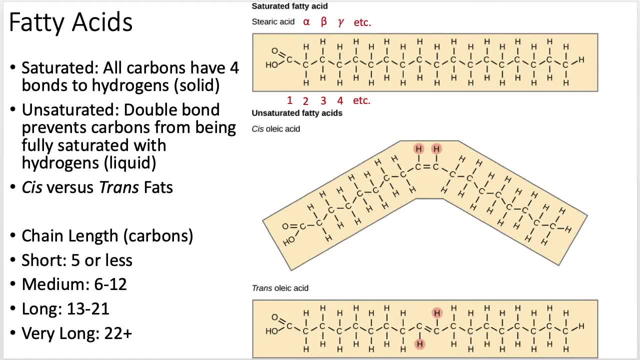 there are really five classifications. Some people don't include very long ones, but you might as well, So they can be short, which is five or less. You'd have medium and long chain ones. Those are generally most of your fatty acids are going to be. 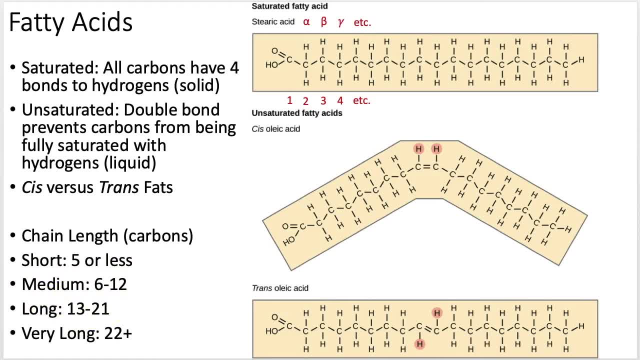 typically medium to long, So are the ones that we encounter. most of the time. You can have very long, but those are much more rare, as are short ones, But the medium to longs are when most of these actually fall in there. Now, one important idea too: if you have this saturated, okay, it's a lot. 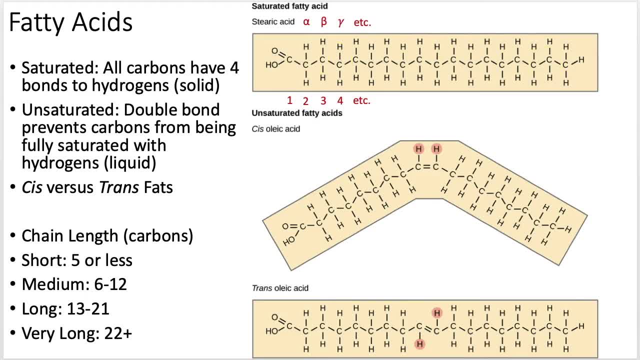 easier to fit a bunch of them close together, And so you can really squish them and stack them. And, in general, trans fats are going to be more saturated, And so you can really squish them and stack them And, in general, 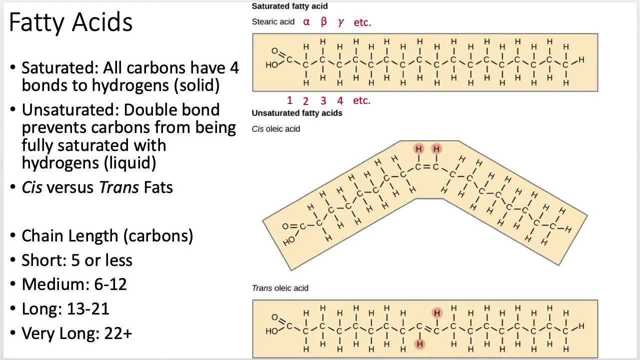 fats that are comprised of saturated fatty acids are solid at room temperature, okay, as opposed to unsaturated fats, which tend to be liquid at room temperature. Now, that doesn't necessarily mean they're healthier either which way. It just has to do with their saturation levels, And I mean 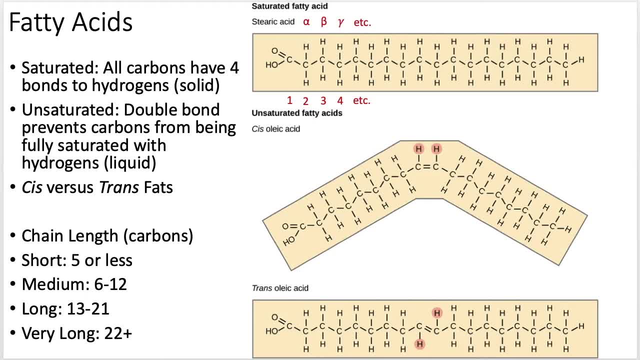 it depends on what you mean by room temperature. I mean, if it's really hot, then, like I remember, we had coconut like cooking oil, fat stuff, and it would be solid in the way that it would be saturated, And then in like summertime apparently, our house got warmer and it was like right at room temperature. 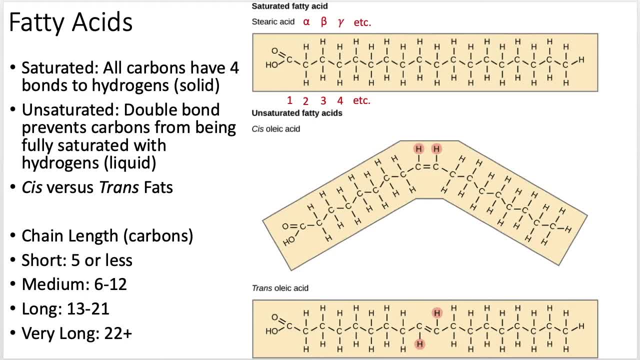 and it would turn into a liquid. So I wanted to show a little video from the osmosis people- I forget what they're called- like osmosisorg, And they're just going to quickly talk a little bit about. they're just going to show you some visuals that talk about this and the process of hydrogenation. 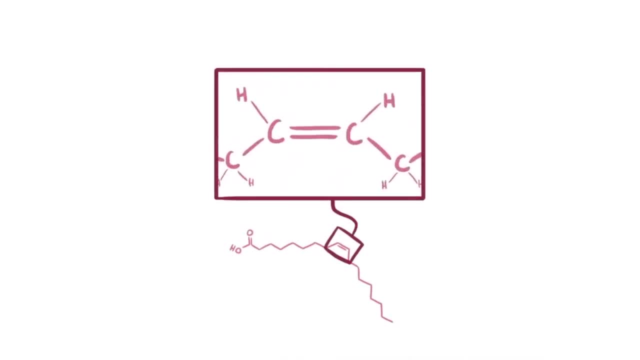 Now looking at the double bond of this unsaturated fatty acid, like most unsaturated fats, it's got a cis configuration. In a cis configuration, the two functional groups are on the same side of the double bonded carbons. Now, when this happens, the fatty acid chain naturally bends. A molecule that 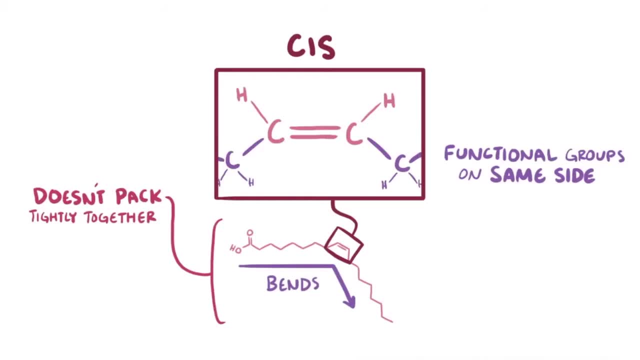 bends does not pack tightly together, so it's a lot more fluid. Think about cooking oils, which are liquid at room temperature. Some fats are in a trans configuration, though In a trans configuration, the functional groups are on opposite sides of the double bonded carbons. 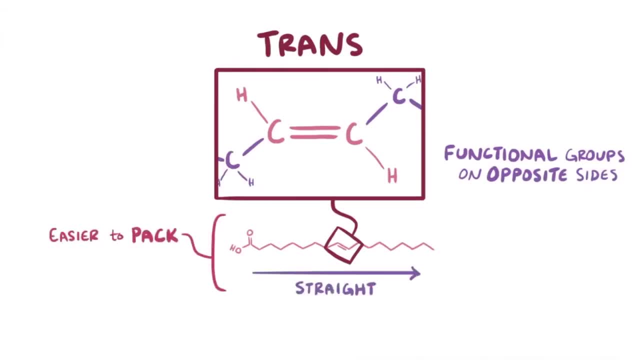 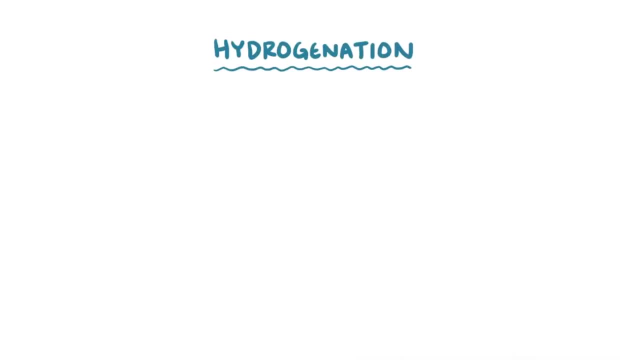 And this keeps the chain more straight and easier to pack. Trans fats result from a process called partial hydrogenation. In just plain old hydrogenation, hydrogens are added to cis fats to get rid of all of the double bonds. So let's say that you've got. 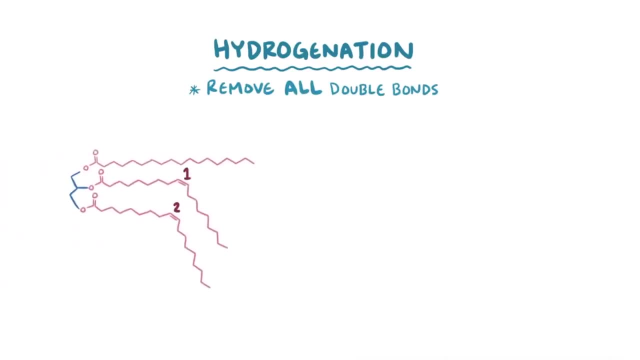 this triglyceride and it has a total of two double bonds. So in this case we'd add four hydrogens, two for each double bond. That turns the unsaturated fatty acids with cis double bonds into saturated fatty acids. Partial hydrogenation, on the other hand, refers to adding hydrogens to most, but not all, double. 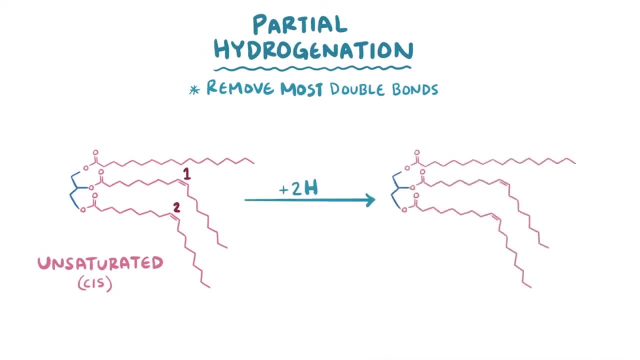 bonds. So let's say now that we add just two hydrogens. When this happens, some double bonds can be turned into single bonds by the hydrogens, but then they might reform And what you end up with is an unsaturated fat. but some of those fats have trans double bonds. 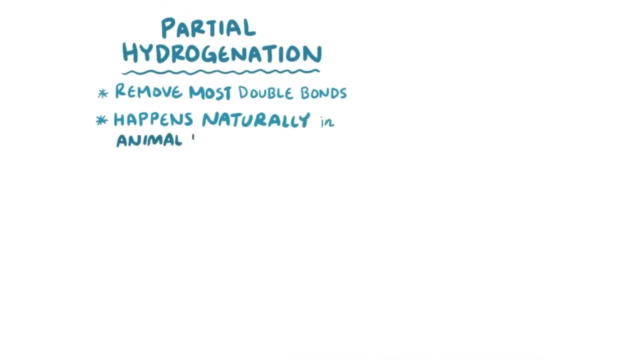 Partial hydrogenation is a process that happens naturally in the digestive tract of some animals like cows and pigs, which is why trans fats can be found naturally in meat and dairy products. Trans fats are also created through the partial hydrogenation of liquid oils, a process that 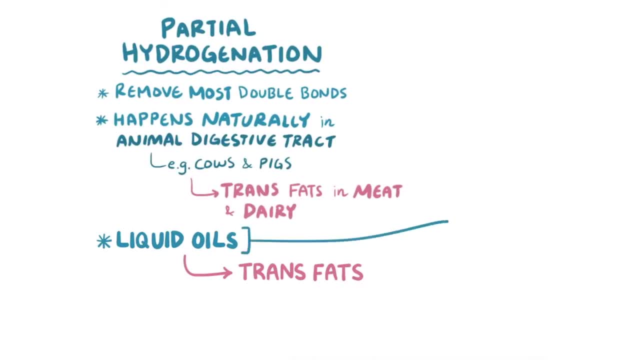 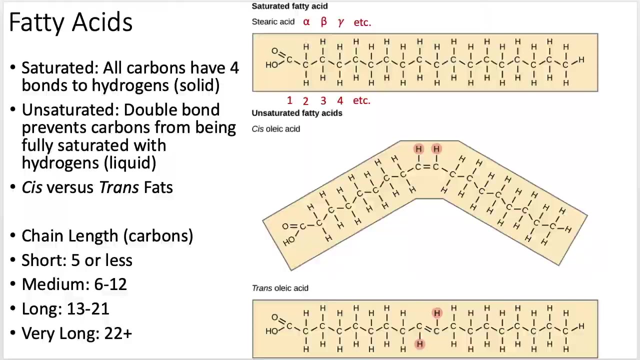 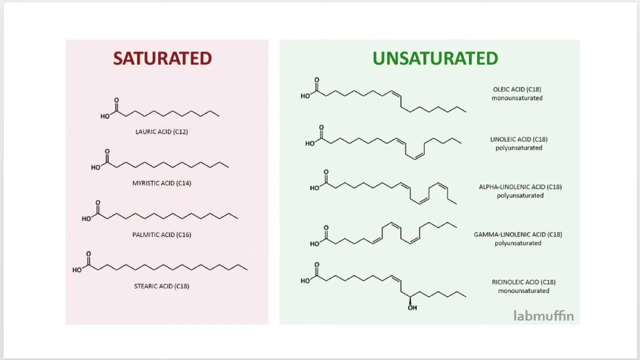 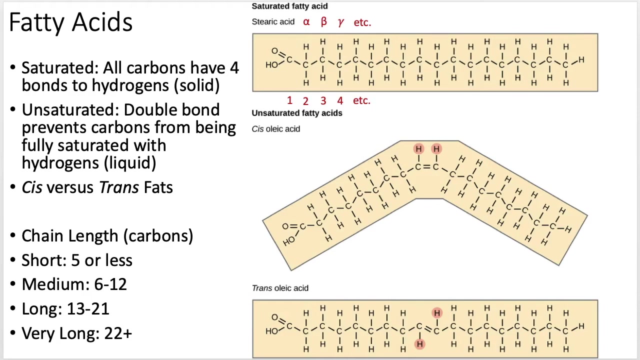 makes them solid. Partially hydrogenated oils have been largely removed from foods in North America and Europe because trans fats have been associated with coronary heart disease. Trans fats have also been associated with carboxylic acid, which is the first carbon that will go into the body. 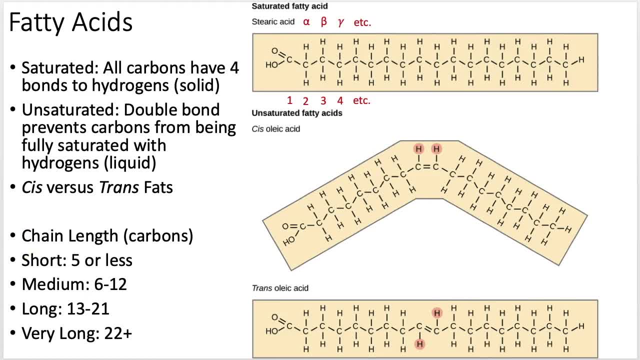 And so the carbon that is now in the body is the second carbon that will be added to the body. This is where you get the first carbon that's going to be in the body And then you go out. But there are some other alternative numbering schedules or naming schedules for the carbons. 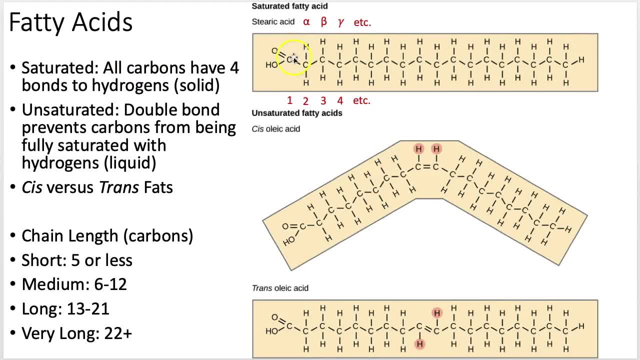 I'm not including one of them because it's really complicated. But if you skip that first carbon, then the number two carbon would be the alpha, and then the beta, and then the gamma, and so on. if you want to use Greek letters, Usually that is just referring to—eventually- you can say like: oh, it's a gamma double. 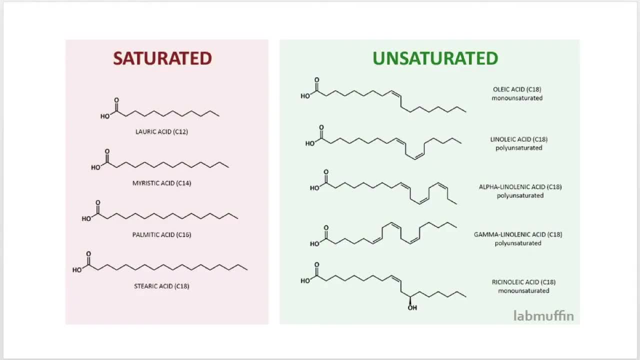 bonds at the sixth, carbon or whatever. So that's where that comes from. Now, the next thing that comes to mind is the difference between carbon and carbon. you can have multiple double bonds in your fatty acid chain, and we call those polyunsaturated, okay. 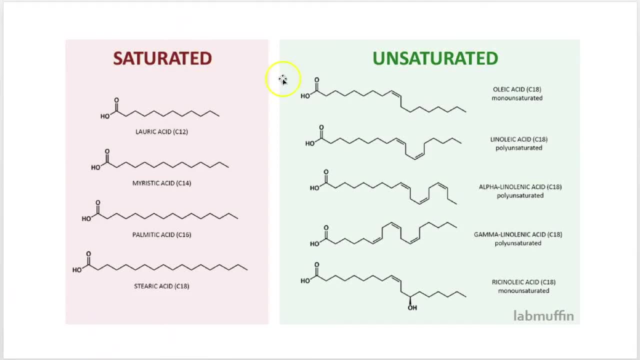 so we can have saturated. you can't have polysaturated, that doesn't make sense. but you can have either monounsaturated or polyunsaturated fatty acids and, uh yeah, they're just very. on carbons now i want you to see this chart. i know the quality. 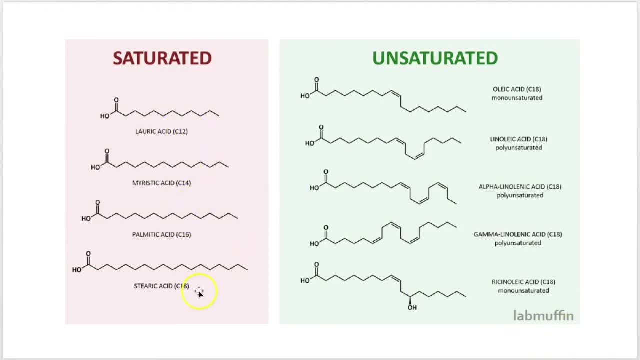 isn't great. but uh notice, uh, 12 carbons, 14 carbons, 16 carbon, 18 carbons. uh, in general we tend to see more of the even numbered carbon chains than the odd numbers. you can have odd numbers, especially 13, 15 and 17, as odd numbers, but a lot of times they're actually even numbered for. 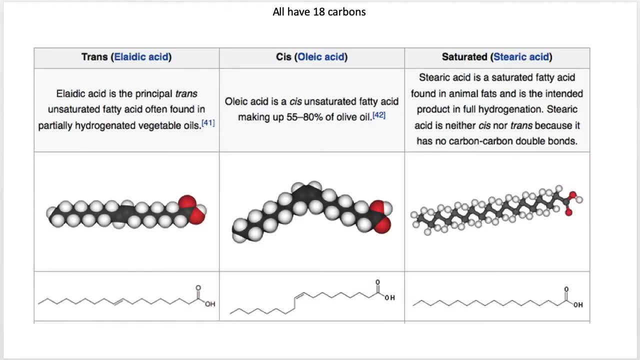 a variety of reasons. now i just wanted to show you this. so here's an example of these are all 18 carbon chains and they all have different names and it all just depends on where that different carbon chain is, and it all just depends on where that different carbon chain is, and it all just depends on where that. 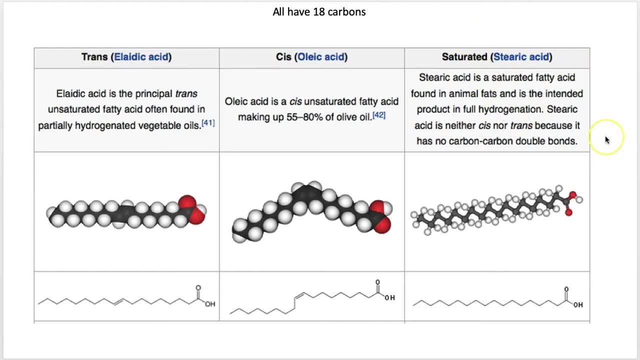 double bond is. so if you're saturated, it's stearic acid. okay, uh, it's found in animal fats. you can make it artificially using hydrogenation. now you have can have oleic acid, which is also a really common one. so most of your olive oil is actually in made of oleic acid, which is really 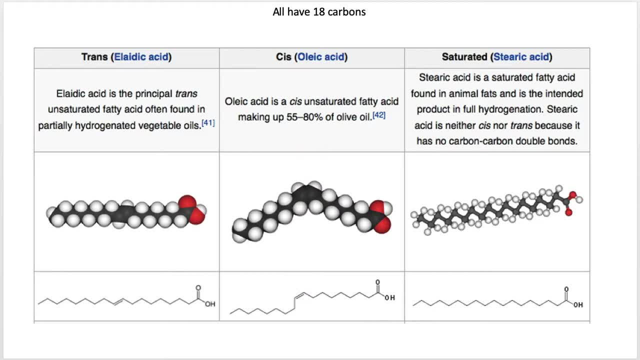 really cool, um. but if you do a partial hydrogenation of maybe like a double cis or a polyunsaturated fat that has 18 carbons and you end up with maybe one trans double bond here we call that- i'm not gonna say that right- eladic, eladic acid. i don't remember, um, but that's one. 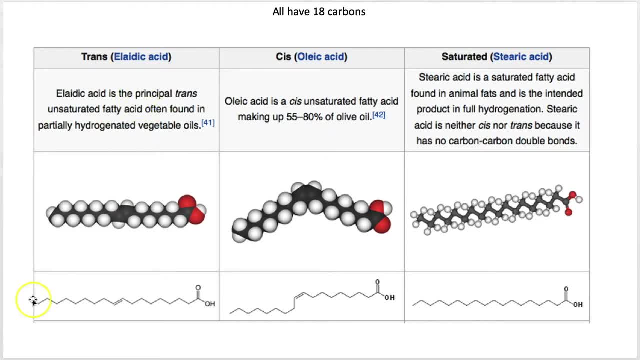 that can show up because it's it's artificially made, right it's? it's a trans fat, because most of the time your trans fats are artificial and there you've got it from partially hydrogenated vegetable oil so you could take a polyunsaturated, so multiple double bonds and if you end up with a 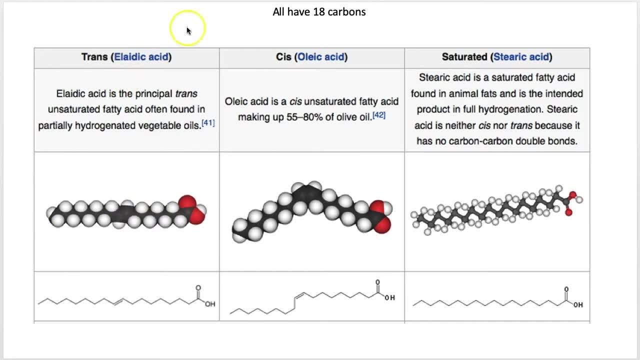 double bond here. that's trans. uh, that's what we call that eladic acid. it's a trans unsaturated fatty acid, so that's important. so that's where you get either hydrogenated soybean oil or partially hydrogenated soybean oil. that's where that's coming from, and this is much harder for enzymes. 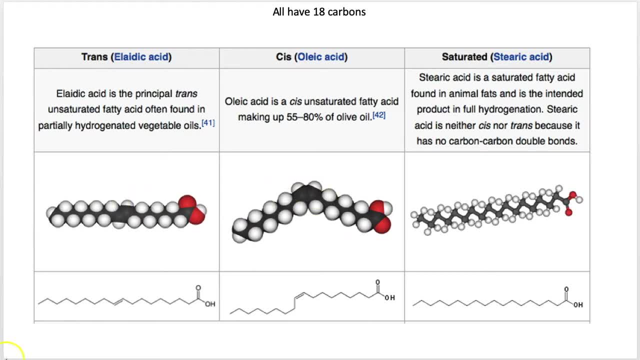 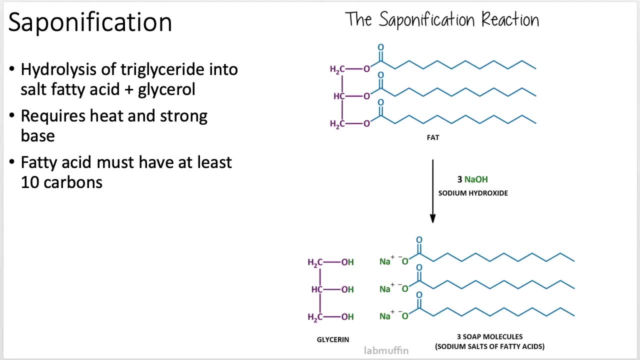 to cleave than like a cis one, and so it lasts longer. last couple things i wanted to hit: uh, a couple of- uh, you could call them industrial processes. uh, saponification, that's making soap, so that's just what we call it. uh, you're gonna take some kind of triglyceride. 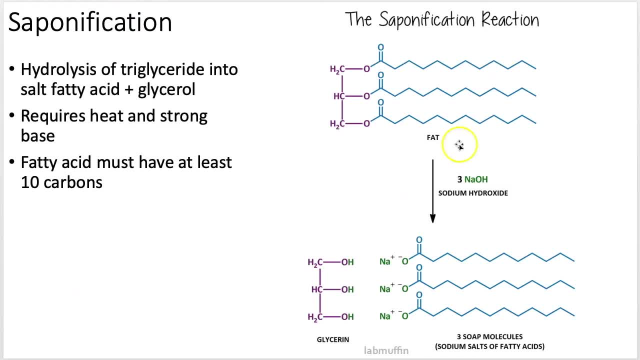 it doesn't have to be all the same length. so that's just common to, if you're just talking about triglycerides in general, to just have them all the same length. but there's nothing that says they have to be all the same length. um, but when you saponify you use heat plus a. 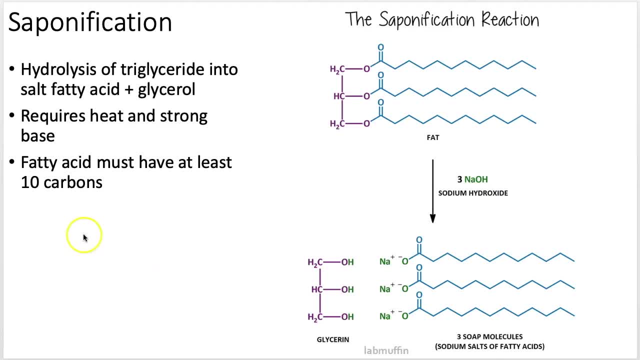 really strong base. so often we'll say sodium hydroxide, and then you will be able to just cleave this off, de-esterify. we call it saponification, but you're going to end up with these soap molecules. so this is, it's salt of fatty acid. so it's fatty acid plus this salt. 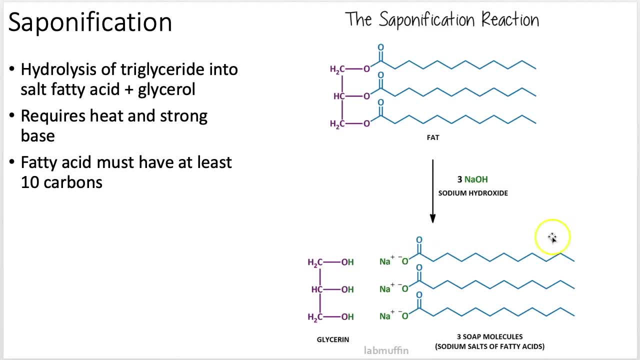 because you have this nice negative charge and the sodium is going to balance it out and then so this can then go on to form like micelles or basically act as the functionality of soap, which is sort of a single phospholipid layer. it's not a bilayer, but it's like a single. 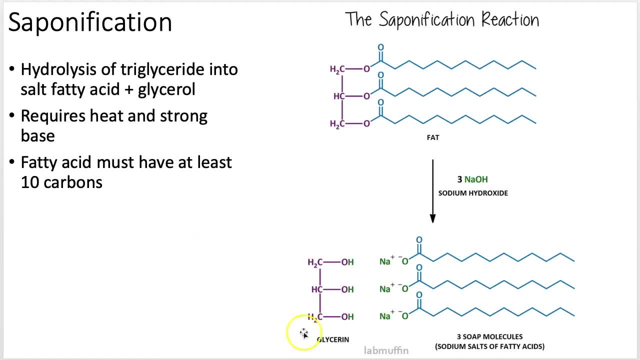 layer. now that is also going to generate glycerin, or you're going to regenerate your glycerol, basically, and this is how you make glycerol, which is a really, really common chemical that's used for all kinds of processes. glycerin, glycerol- same thing. 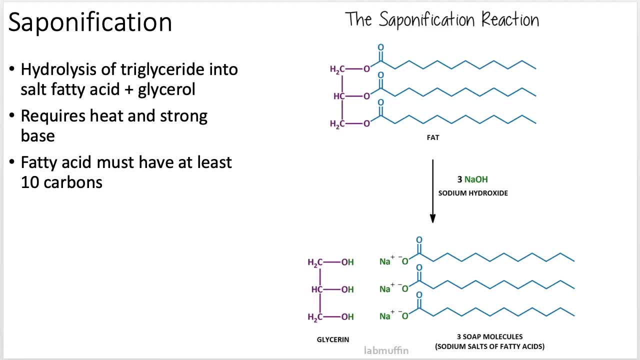 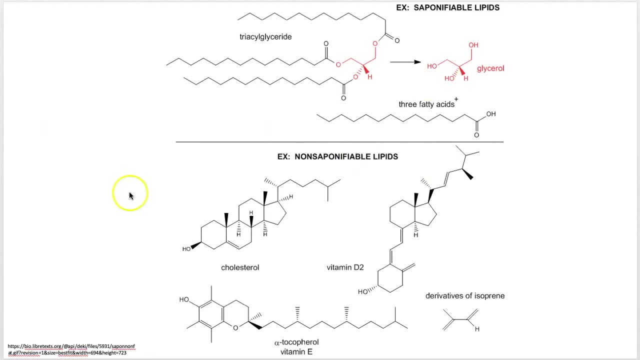 and so, yeah, this is the- i think, the number one way to actually make glycerin too. now i included the next slide. just, you gotta have a fatty acid to do it. so, like i don't know, i just thought this was funny, i guess- uh, because you gotta have a, there's your triglyceride, uh, or? 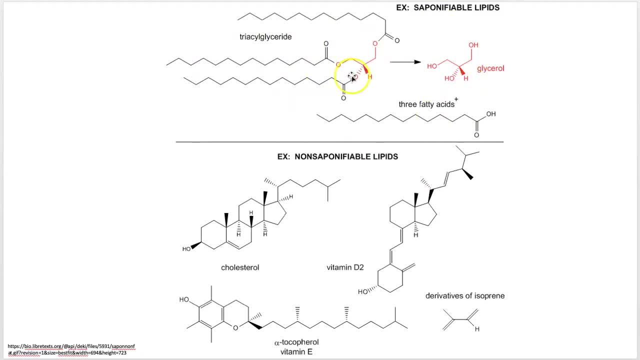 your triacyl glyceride? sure, fine, whatever, same difference, uh, and then you're generating glycerol from glycerol, so it's just a very simple way of doing it, and so i don't know, it's kind of a crazy thing to do, um, but you have to because you can't saponify every kind of lipid, i guess. 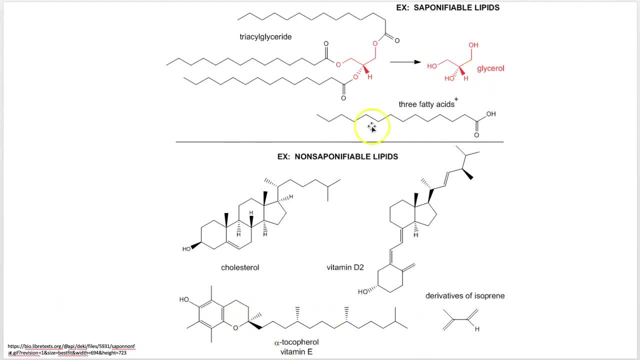 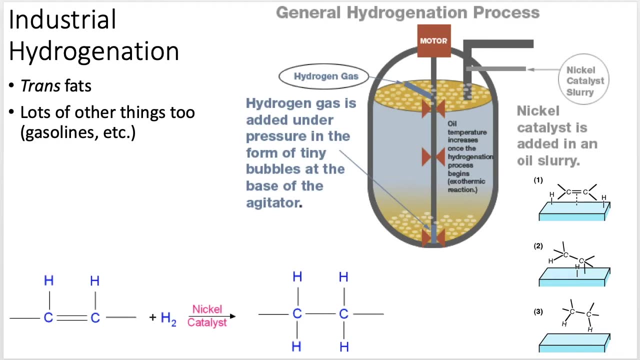 that's the whole point of this. it came from like a textbook, um, i mean, if it's a goofy looking sterol or whatever like or a tocopherol that's like got all this crazy stuff on it, yeah, you can't get it to react, so i don't know. it seems pretty straightforward. another really common: 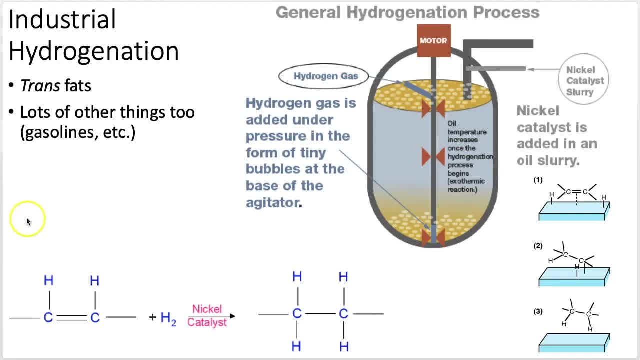 fatty acid, fat just associated thing is how we actually hydrogenate things. now the process of It could be anything, So any kind of long chain carbon molecule that has like a double bond in it, then you can add hydrogens to it, of course. 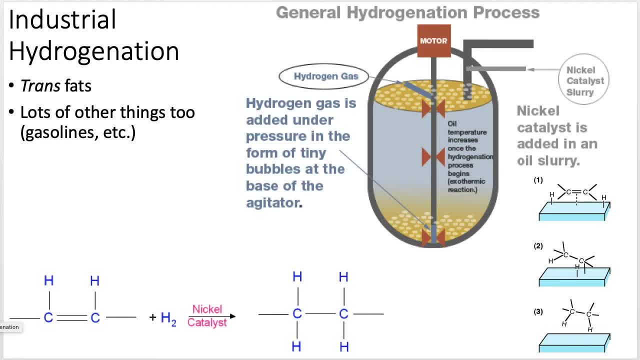 Now you need to apply heat, usually, and you need to supply extra hydrogen. Okay, so hence this is just the process, how you would typically use a nickel based catalyst, So you would throw the catalyst in and then you add hydrogen gas, of course. 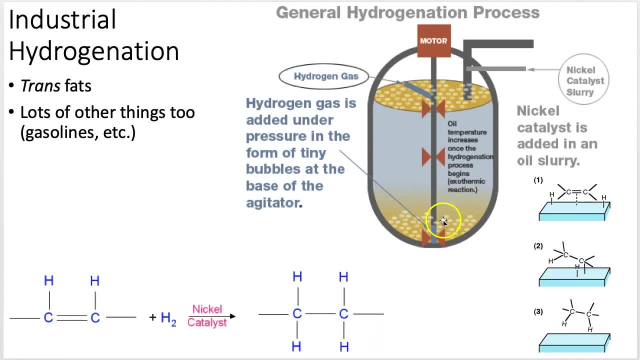 So this is super dangerous because you have gasoline or some kind of fuel with hydrogen gas, which is incredibly flammable, as well as a nickel catalyst. Things are happening. It's really dangerous. But hey, you got to make some food, You got to make your trans fats or you got to make your partially hydrogenated soybean. 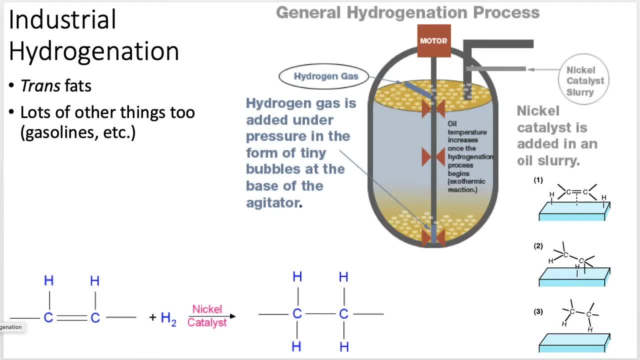 oil so that people can eat it, because people like to pay for food, And I mean, that sounds like I'm judging that I like to eat too. So you often will use a nickel based catalyst for this. Why, Well, the catalysts? 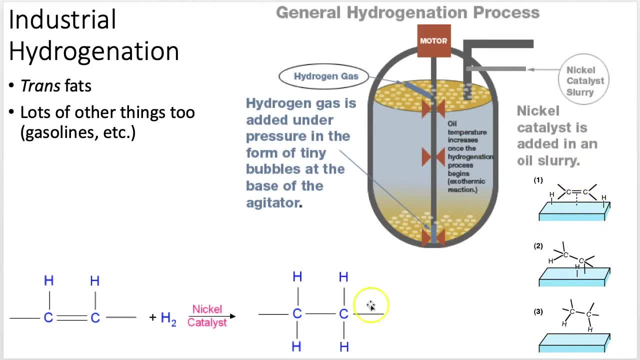 The catalyst is actually this blue block here, And then it lets you, So the nickel will hold on to the double bond as well as the hydrogens, And then it's just bringing everything together. It's just like how enzymes sort of bring things together and let them happen. 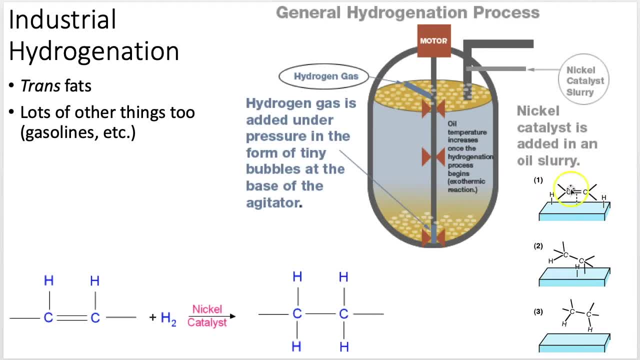 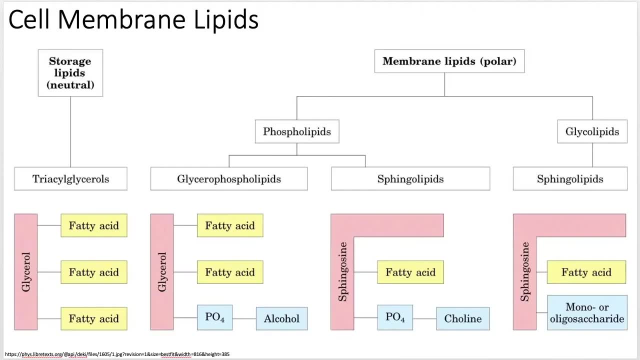 Well, that's what they're doing here. They're bringing the double bonded carbon with the hydrogens close together and allowing the reaction to occur, which is kind of cool. So we're going to start moving on into the cell membrane. So I'm going to try and keep it relatively organized. 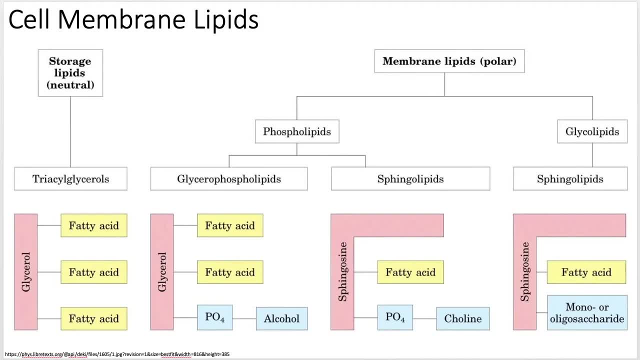 But there's going To be. it's going to get a little chaotic when we start talking about sterols, because we do see our phospholipids and our other lipids that have a charged head and a fatty acid tail. Yes, those make up our membranes. 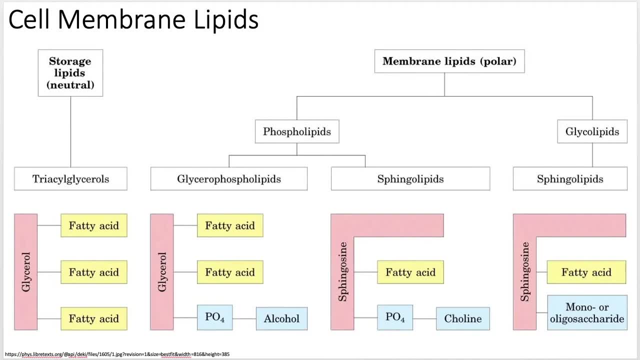 That's basically their job. But we also do see a lot of sterols like cholesterol in the membranes. But there are other sterols that are used for other things, And so we'll try and stay organized here. So if we're going to store stuff, there's your triacylglycerol. 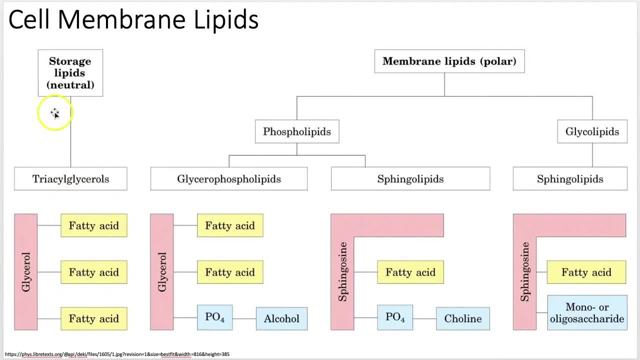 There's your triacylglycerol, There's your, your triglycerides, your triglycerides- over here. Now, our membrane lipids kind of fall into two big categories. You got your glycol lipids, So that's where you're going to throw on a sugar. 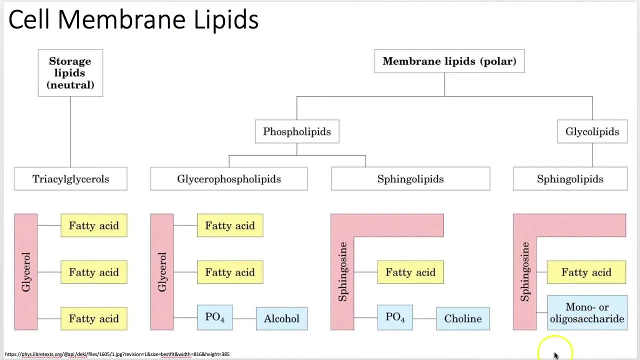 So we talked about that last time, where you have some kind of saccharide, either a mono or oligosaccharide- I suppose it could be a polysaccharide, but you'd probably call it an oligosaccharide- Or you can tack on some kind of phosphate, either with an alcohol or 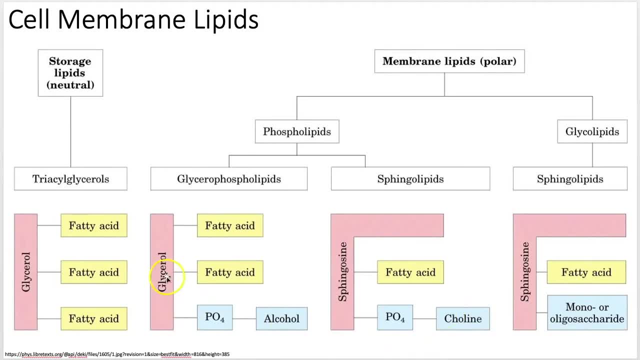 choline, And those can either fall under. They can either have a glycerol or a polysaccharide. So you can either have a glycerol or a polysaccharide. You can either have a glycerol, just like triacylglycerols do, or you can have a sphingosine. 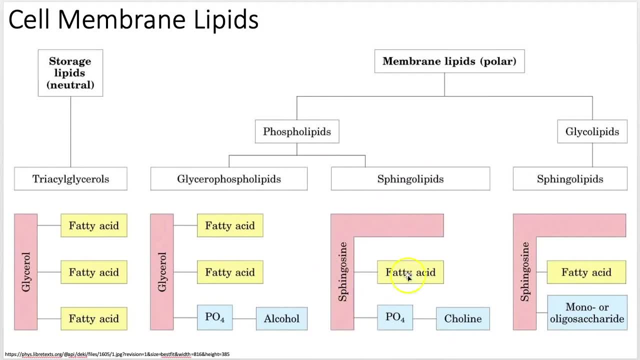 But basically you just have another carbon based structure with a fatty acid, So you have a nice charged area, So this is kind of where the charge comes from, And then you have those fatty acids that stick down, And so this is a classic look of what it looks like. 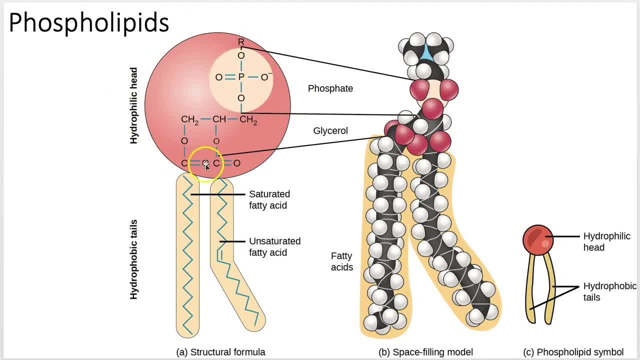 What? And so you have your nice charged head. So instead of just being completely hydrophobic, like our fatty acids are, then we can have a nice hydrophobic, Now that hydrophilic region does not have to have a phosphate. 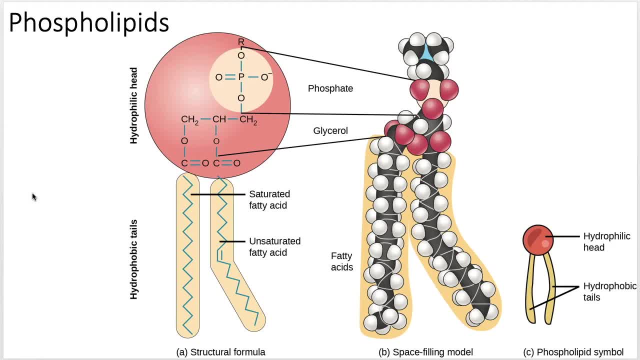 OK, a lot of times they do. We generally say phospholipid bilayer, because I don't know that's just what a lot of them are. They don't have to be, of course not. it's biology or biochemistry. 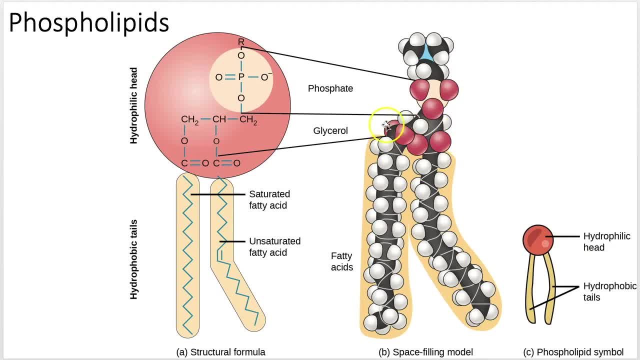 So like. of course there's exceptions always, But notice you also, you have that glycerol and you have your fatty acid, So it's really not that different from a triglyceride, except you have this other little head group here, But generally you just have those two. 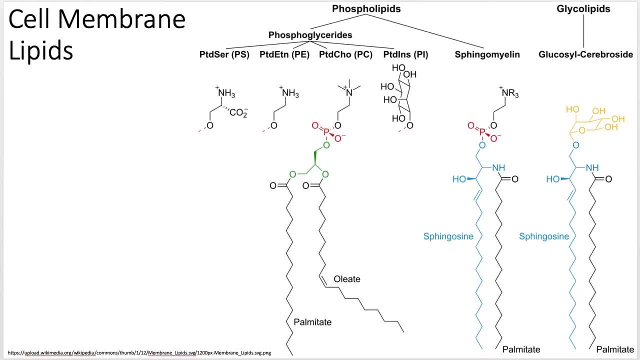 Two sides, hydrophobic and hydrophilic region. Now you can get some variety in there. There is so much information out there about the different kinds of phospholipids that you can generate, or just the different kind of cell membrane lipids. 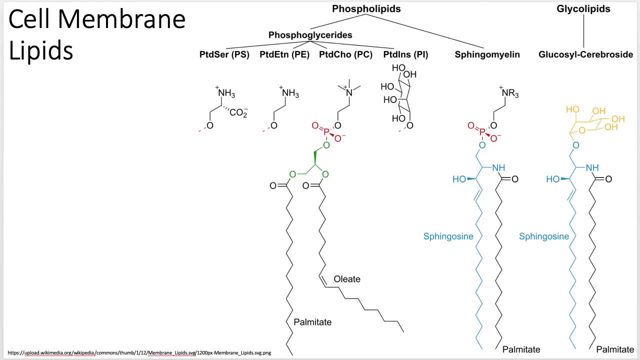 There's huge charts, There's entire research groups whose job is to do this, And so you can just find all kinds of different things, But basically you're going to have a charged region with some kind of long chain and something I want to. 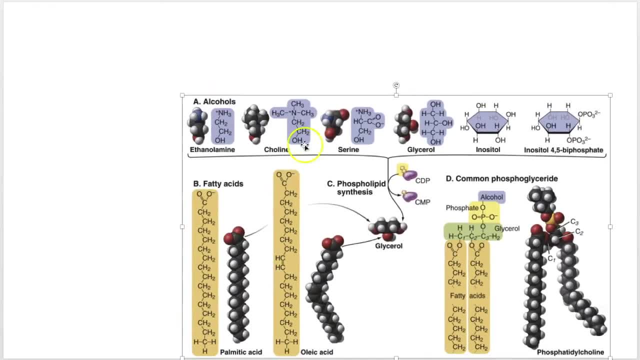 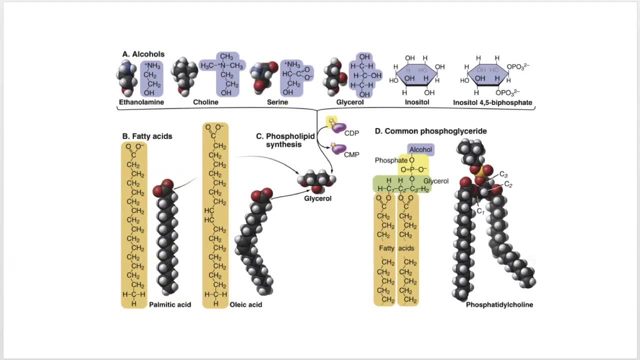 keep in your brains is man. I swear I have like better quality pictures. When you have a nice long straight chain like this, you can stack them really tight. OK, but that might not necessarily be what you want, because you're going to get a lot of hydrophobic. 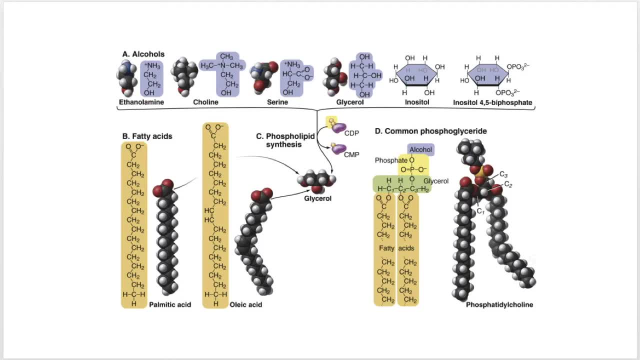 interactions between each phospholipid, and that can really kind of stifle things. It can hold things a little too tight. So sometimes you actually want some kinks in there, And so that's where you're going to add in your double bonds. 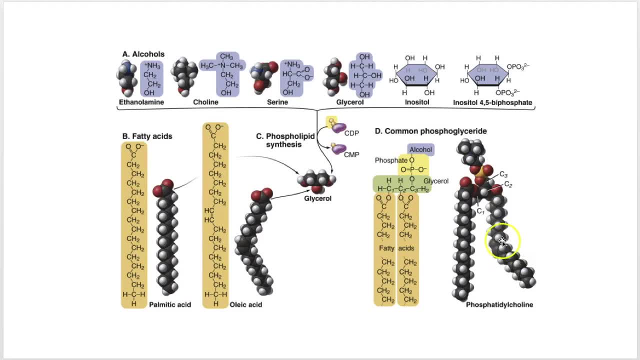 You can get some cis fatty acids going and then that gives a little kick So it looks like he's like walking, but that's going to put some extra space in between the nearby phospholipids And so that can really kind of open up your lipid bilayer. 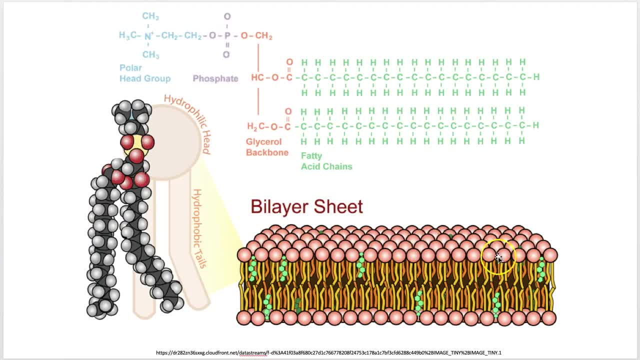 So here's just a classic image of what our lipid bilayer looks like, And you can see you're going to want some kinks in there. That's really, really important. And what are these? Oh, what are those? Those look like sterols to me. 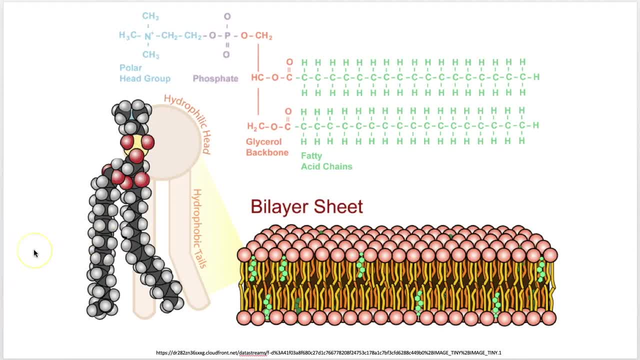 Interesting. Well, we should probably talk about those. But phospholipids And general membrane lipids form naturally form these kinds of sheets, So you can have a monolayer sheets. of course, that's like what soap kind of forms. 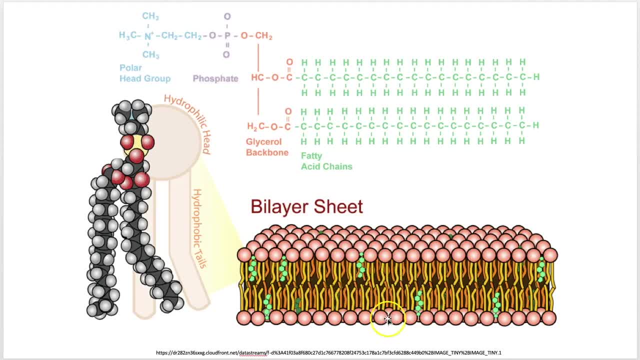 But you can also have these bilayers where your hydrophobic regions line up and then your hydrophilic regions line up on the outside where there's actual water, because we're basically always dealing in water as our solvent, as opposed to in some industrial processes. 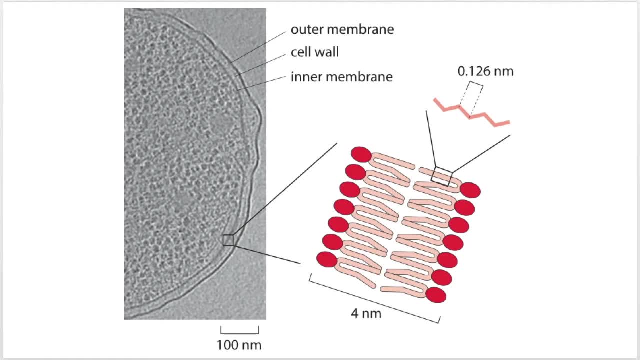 I mean, water might not be your solvent, but hey, it's biochemistry, Not chemistry. Just to show, like, the size of these 0.126 nanometers, Okay, Wow, Okay, It's just kind of interesting, I thought. 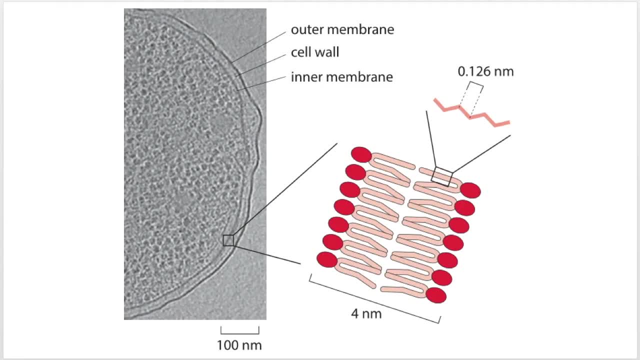 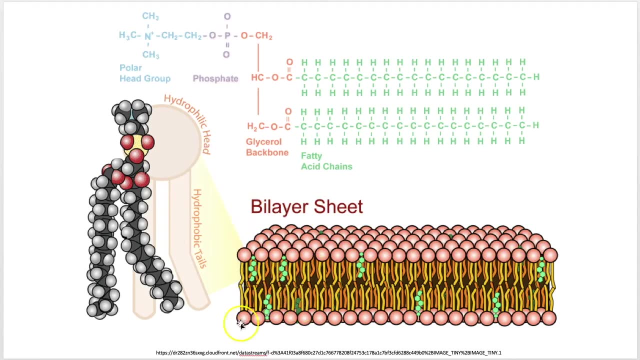 But this is where we're at. We're inside a cell, We're looking at it, We're trying to see what's going on now. This is interesting. So what we actually learn is that phospholipid bilayers are not just made of phospholipids. 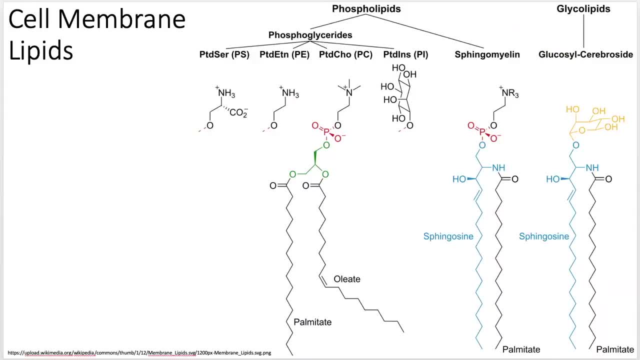 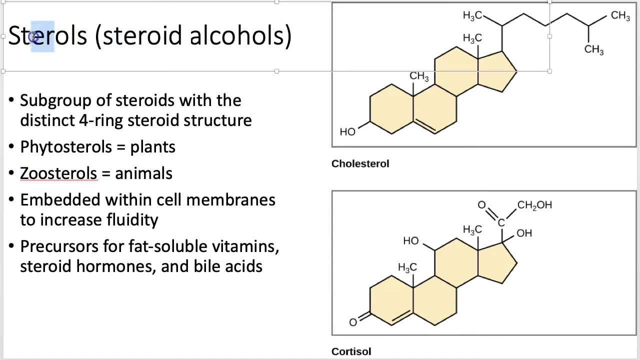 They're made of all kinds of crazy lipids that have charged heads, as well as sterols. So we need to talk about sterols, which comes from steroid, hence ster, and then alcohol. So all So steroid alcohols. 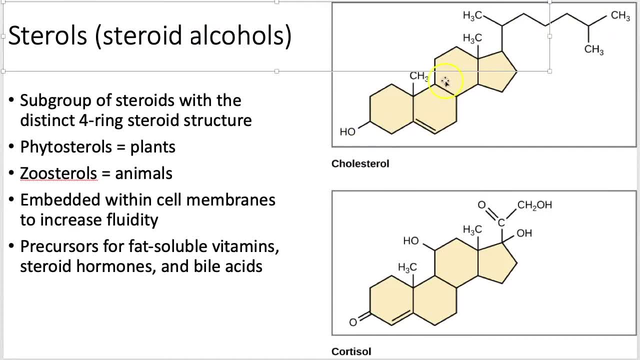 Okay, So there's your alcohol right there and this is your steroid, and then there's your alcohol and there's the rest of your steroid structure. Now they have this consistent four-ring structure. Okay, This is a subgroup, So steroids don't all have to be sterols. 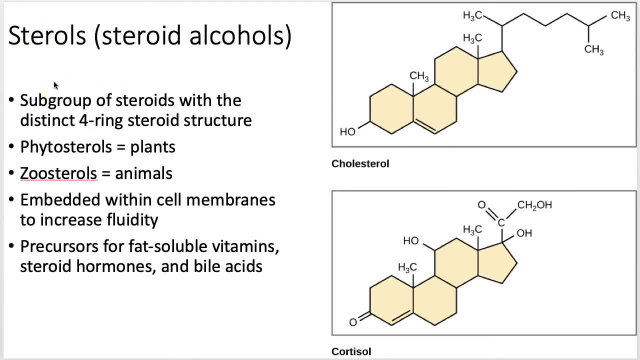 Okay. So it's like not a All steroids. Okay, All sterols are steroids. They're steroid alcohols, but not all steroids are sterols. That's why I'm even talking about this. It's a subgroup of steroids. 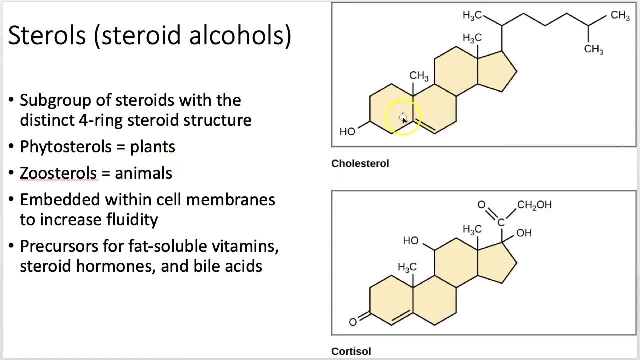 Oh man, I'm getting myself mixed up, because this is this ring structure. oh my gosh, This ring structure is the steroid portion. If they're in plants, they're phytosterols, because plants, and then, if they're animals, 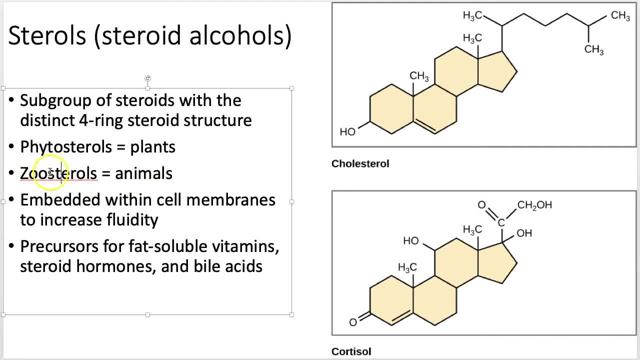 they're zo, I would say zoosterols, but you could probably say zoosterols Whatever. It's fine. They increase fluidity and we need to talk about that a little bit. We're going to get into that in a little bit. 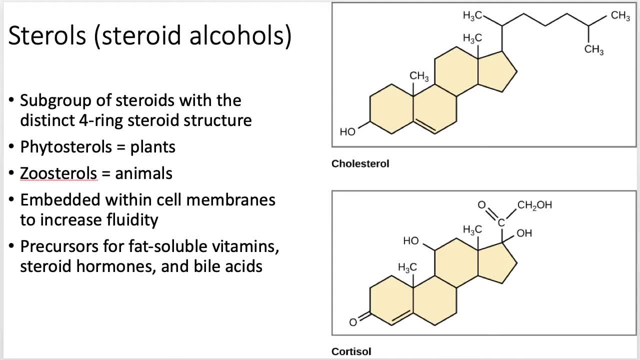 We're actually going to wait a little bit, So I'm looking ahead and realizing that I want to talk about some other stuff, like where we actually make these, But they're in the cell membranes and they're precursors as well, So it's not just for cell membranes. 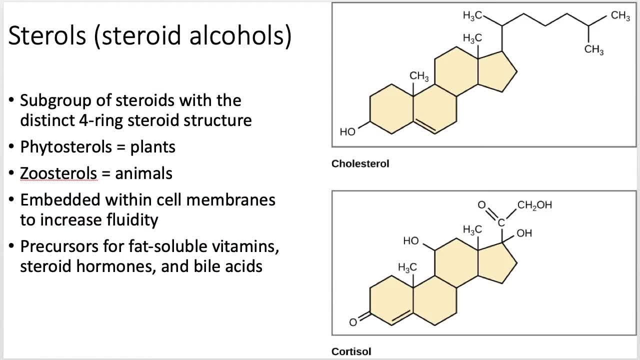 They're super-duper important- Arguably just as important as your phospholipids or your sterols, but they're also really important for the cell membrane. Okay, They're also really important for steroid hormones, bile acids and some vitamins. 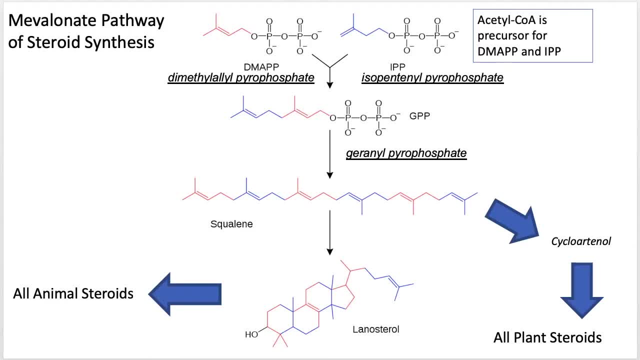 Not all vitamins, but some vitamins. A little bit about where they come from. The main pathway is the mevalonate pathway, mevalonate pathway, however you want to say it, And you have all these precursor molecules. Okay. 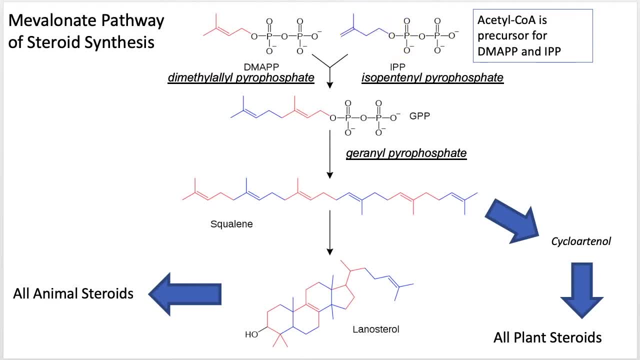 So we've got these long-chain carbons and we just are going to basically combine a bunch of small carbon chains to build these nice ring structures. So it's organic chemistry basically, But I mean you could argue it's biochemistry. 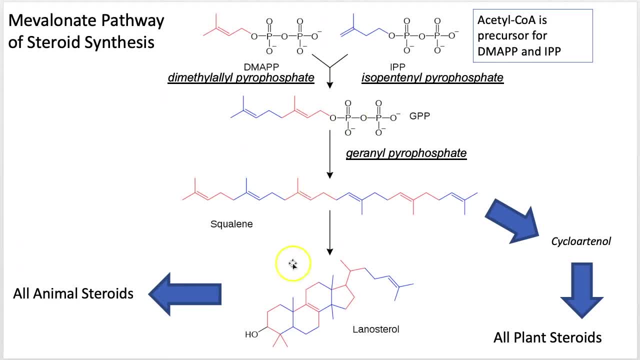 But it's a classic. This makes me think of doing like organic chemistry lab and when you would have to do, you know, like each reaction and then build a bigger molecule, and then you combine those and you get them to fold over and eventually you can get some of them to come out like this: 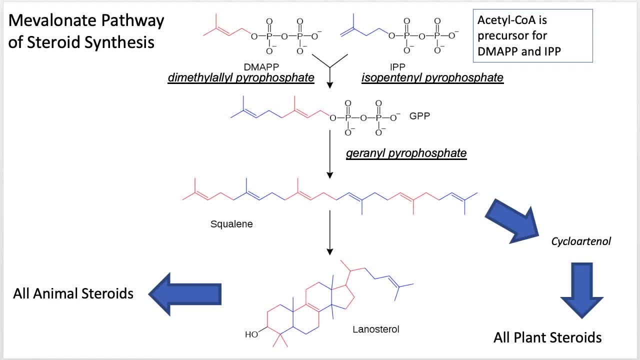 Now, squalene is a really common molecule. It's used a lot in like all kinds of processes. It came up when I was in grad school in vaccines. It just it's really, really common And it's common in like every organism ever. 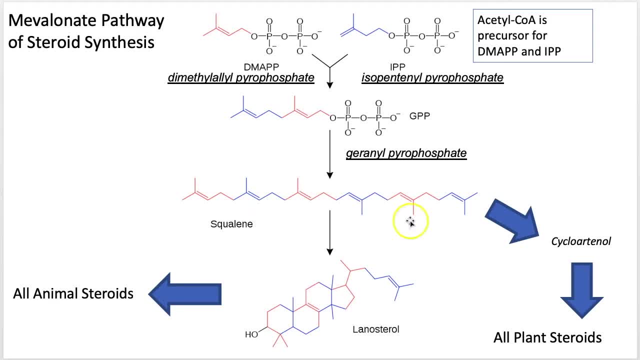 And you make squalene if you're a plant, if you're an animal, a fish- I know sharks have a bunch of squalene in them And you can get that to fold over. You're basically like folding this onto this and this onto this and this onto this. 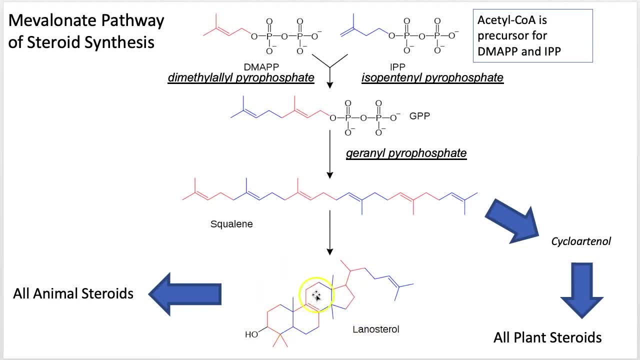 And you can form that sterol basic structure. So you've got that nice steroid in here, And then you add, like an alcohol group, onto various spots to actually generate your actual sterols. And so plant steroids start with squalene, as do animals. 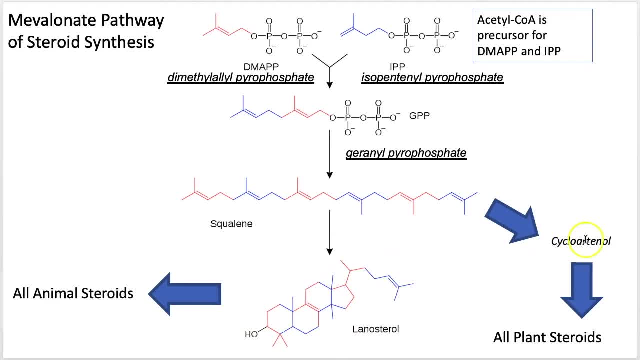 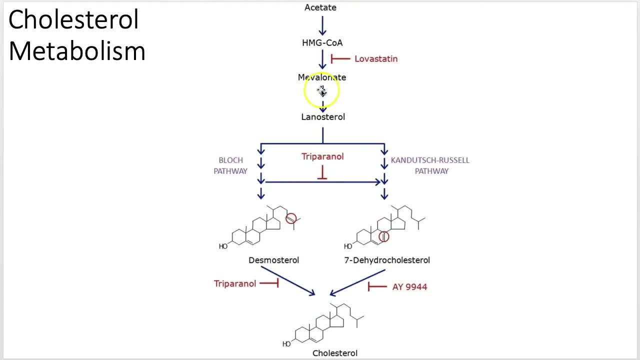 But animals have a lanosterol And plants use cyclartanol. So fun fact. Now, why am I showing you that? Well, it becomes medically relevant. So I wanted you to see mevalonate. So mevalonate, there's mevalonate. 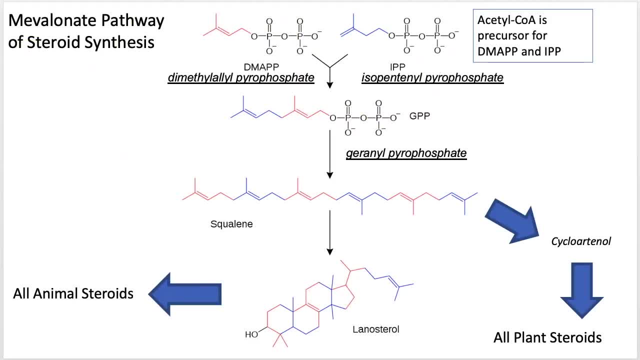 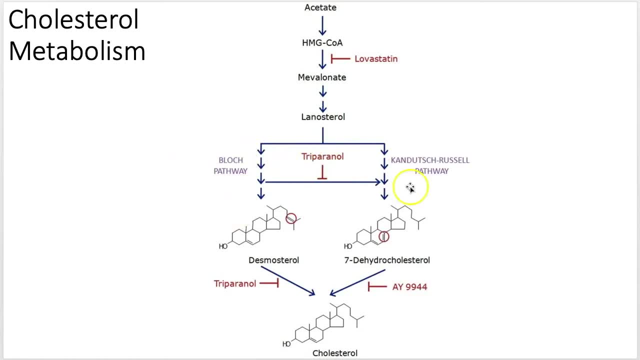 So this is the mevalonate pathway, because you end up with, you start with mevalonate And then you end up going down. You end up all these. there's a couple different pathways and how to actually build these crazy-looking things. 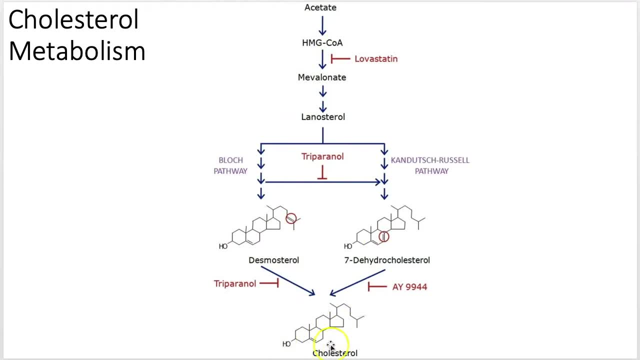 And look the whole point here. there's a lot going on. okay, I understand that You're ending up with cholesterol. Everybody's heard of cholesterol, right? What's your level of cholesterol? What's your LDL? What's your HGL? 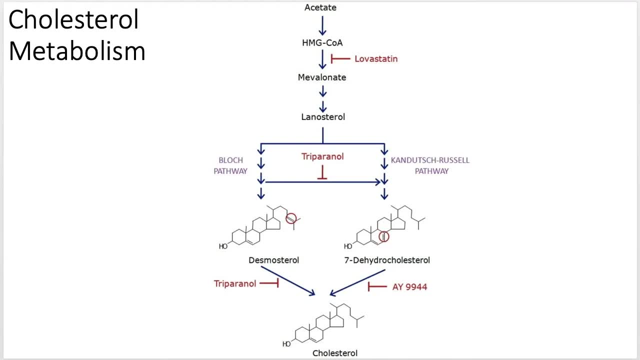 Most of you watching this are probably younger, so you may have never had a cholesterol examination or level check. I have mine in two weeks because I'm in my mid-30s and that's something they like to look at, Though mine's always pretty good. 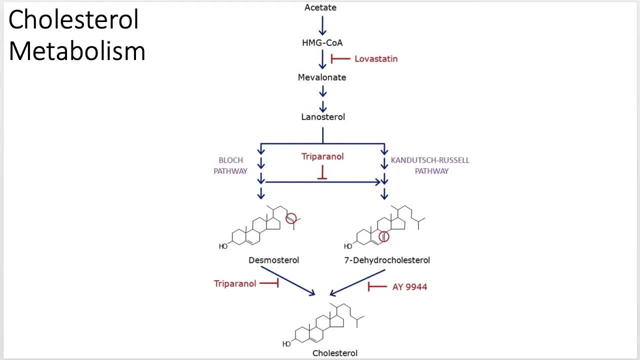 But they're going to measure your LDL, your low-density lipids, your high-density lipids, And we're going to talk about that in a minute. But basically I just want to show you. You can ask your dad or maybe your grandpa- I have no idea how old you are- if they're on a statin. 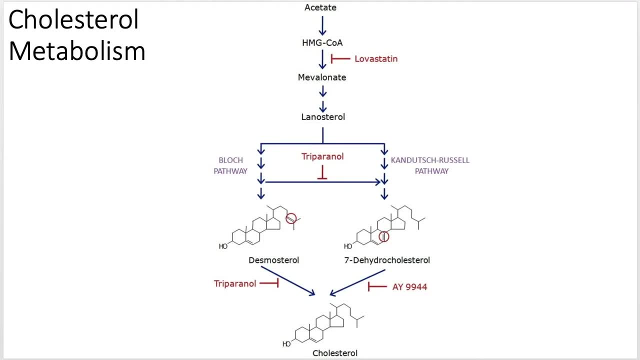 So my dad is on statins. So statin drugs drop your cholesterol. Now there's some debate about how important your cholesterol levels actually are to your health. But arguably you could say: I mean, if you have high cholesterol levels in your blood, that is going to technically allow for the formation of cholesterol. 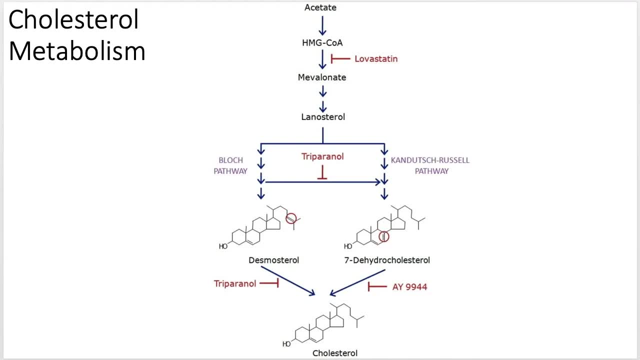 It's going to allow for the formation of more like bad things, basically plaque formation in your vessel walls, along the endothelials, And so generally you want to keep it lower. Now it turns out that's an oversimplification, but hey, whatever. 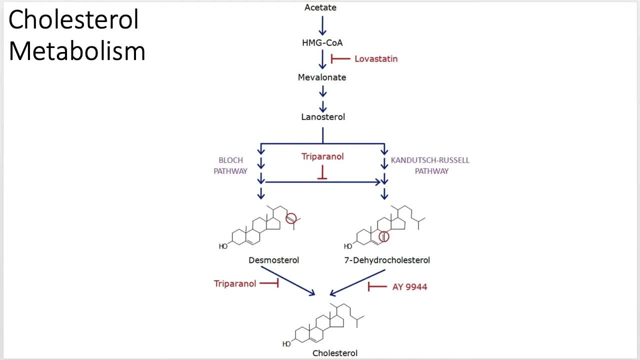 So if you want to drop your cholesterol levels- because it's, I don't know, the mid-90s and they think that's the most important thing in the world- instead of diet they can just put you on a statin drug or one of these other drugs that are going to block these specific pathways. 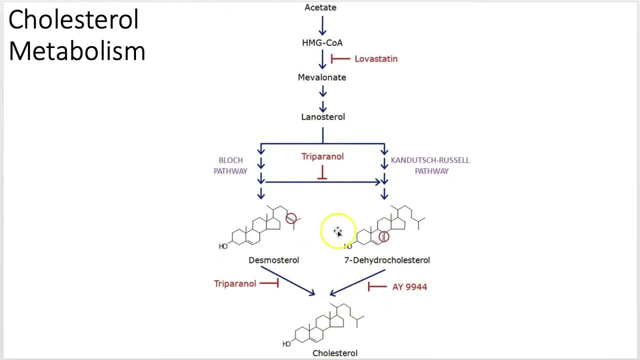 And they're all just these pathways that lead to cholesterol. But look at, if you take a statin drug, that's blocking it really early on And that's why statins are really, really common. Now. they do have some other problems, though not that we need to get into statin drug metabolisms and side effects. 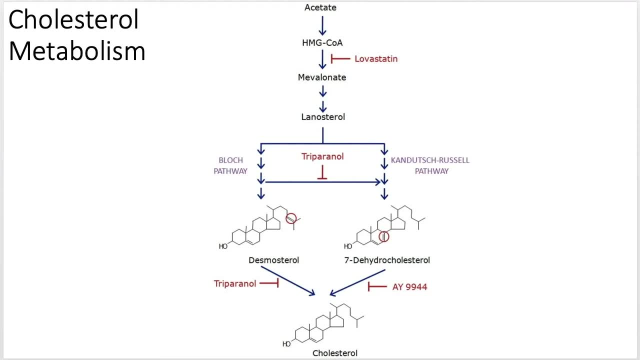 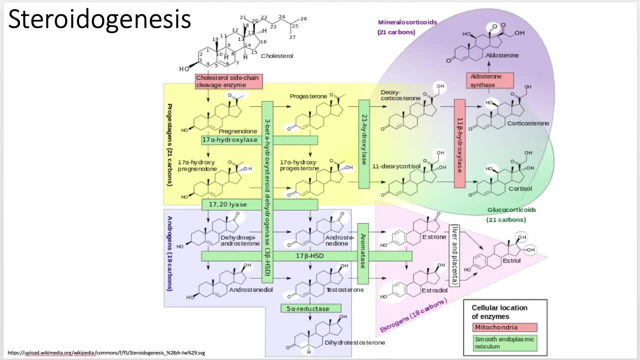 But there are a lot of side effects to statins. My dad always had joint issues when he was on statins, So let's keep on going So. talking sterols, steroids, So your sterols can be nice precursors for a lot of things. 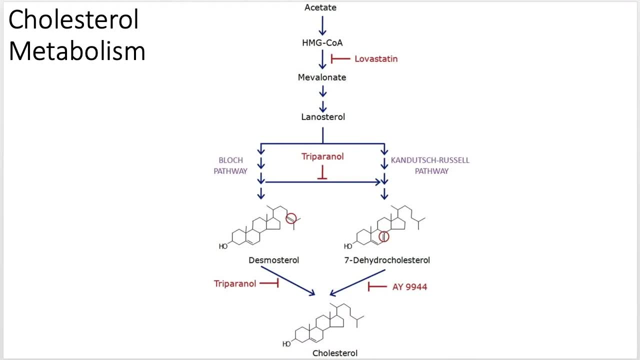 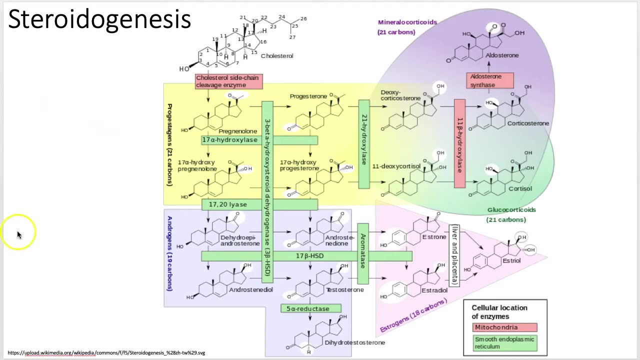 So cholesterol? Cholesterol is basically one of those things that you're going to use a lot in your cell membranes, But that's not the only function for sterols or steroid-based molecules. A lot of them are signaling molecules: Your progesterones, your androgens, your estrogens. 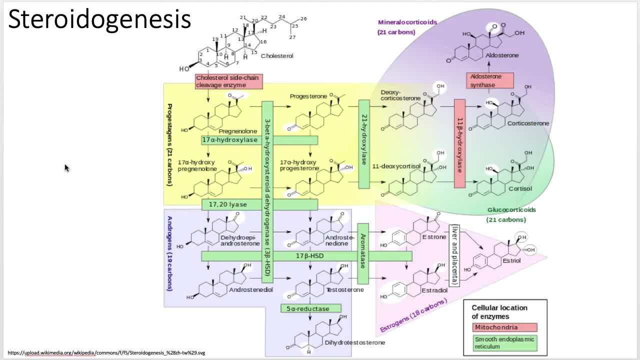 I don't think I'm looking on here. I don't think testosterone is one of these. Oh no, there it is. Yes, testosterone is. So we've heard of all of those things. right, Your estrogens, your testosterone. 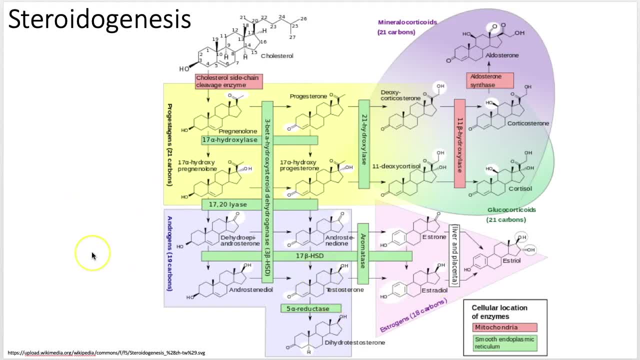 All your sex steroids that are sending cell signals, right, And so the colors here just kind of indicate, like where they are, like what kind of compartment they are or what kind of like. is it a prostagoid? Then it's in the yellow. 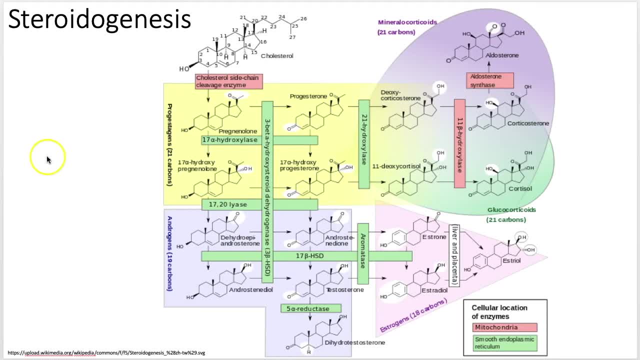 Does it kind of bridge the gap between those? And where is it made? Is it made in the mitochondria? Is it made in the ER? It all depends on the cells and what kind of cells they actually are, But it's really really interesting. 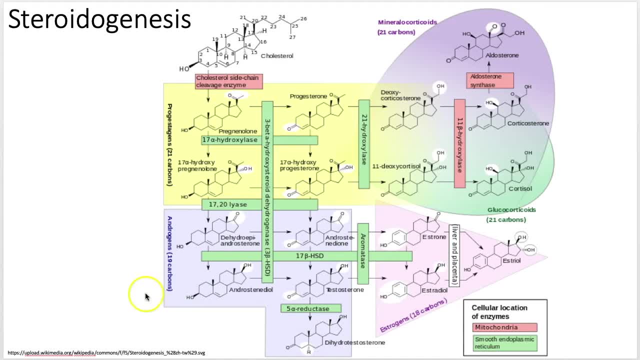 And notice the carbon amounts. You got actually odd numbers of carbon, Interesting, Anyway, so really really cool stuff. We call that steroidogenesis, But you can start with cholesterol to actually build all of these, So this is really important. This is why you need to actually consume fats. 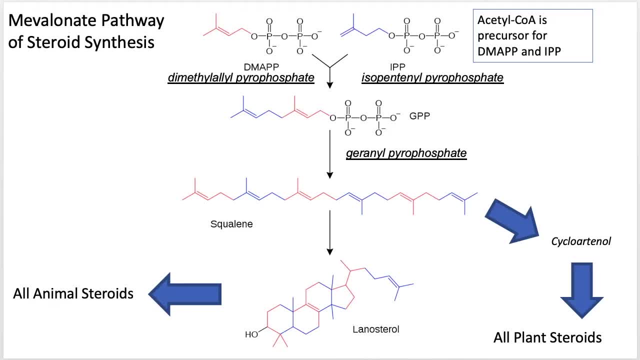 Fats are really, really important because we can break fats down into these precursors and then build them back into sterols. okay, Among other things, You can get these precursors from pretty much anything that you eat, But fats it's easy. 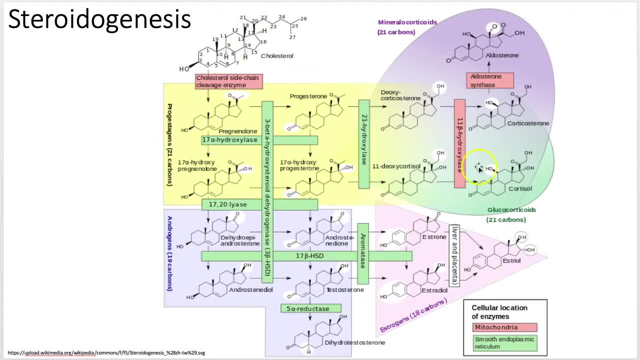 And so you can get those things to make these cholesterols, in order to make these hormones to actually make your body do stuff. So that's really interesting. That's why this stuff is actually important. So, speaking of important things, vitamin D is something that we need to talk about. 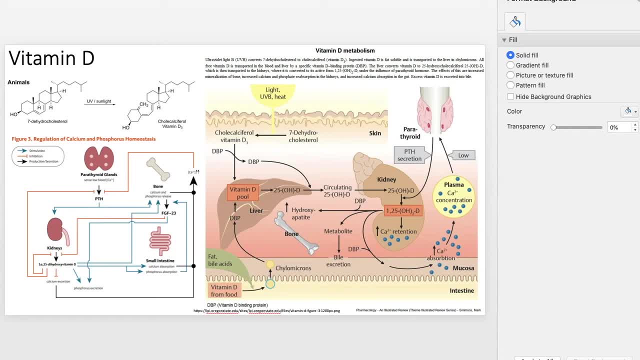 So this is kind of the quintessential vitamin that we talk about when we talk about sterols and steroids And when you get UV light. now you can eat vitamin D and consume it from your foods, But you can also generate it from UV light. 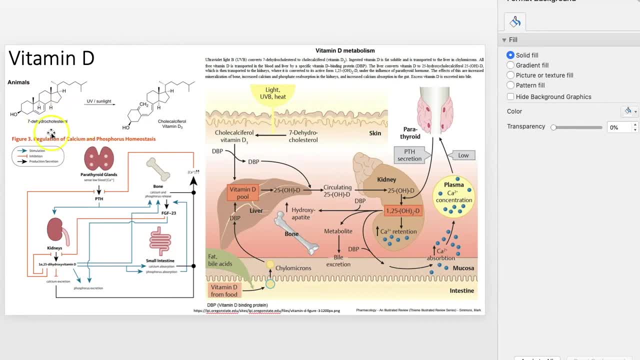 So you can take your precursor of it. It's cholesterol 7-dehydrocholesterol, So it's lost a water molecule And you can have sunlight. actually, You're basically breaking this bond right here, part of that ring structure, and opening it up. 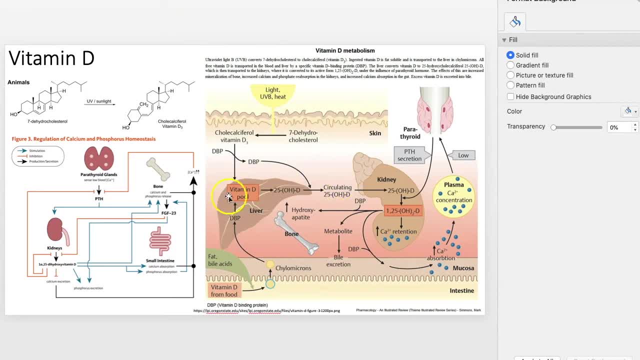 And that lets you just kind of do some things to it and store it long-term inside the liver, And so you have that nice vitamin D pool And we can use vitamin D in part of our stimulation and inhibitory pathways for our body, And we can use it in part of our metabolism pathways for controlling calcium and phosphate levels in the blood. 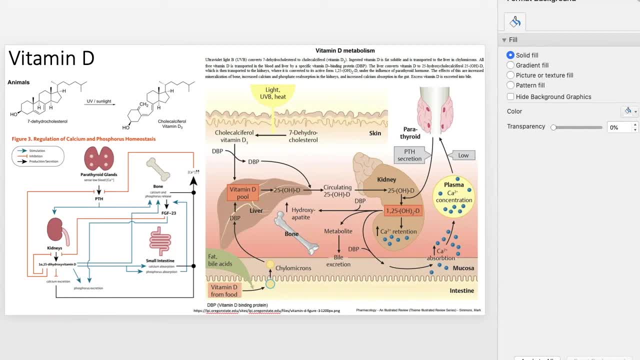 Well, calcium is not just for building bones And phosphate is actually So like calcium. phosphate is one of the main ways that we actually build bone, But it's actually used not just structurally, but also those two molecules. So calcium and phosphate are super important signaling molecules. 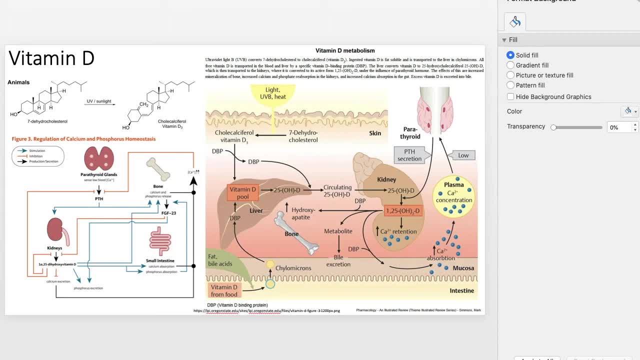 I mean we use phosphate for ATP and ADP and AMP- right, We use phosphates all the time. Your RNA backbones your RNA backgrounds. You phosphorylate things all the time, So you need lots of phosphate in your blood And you also need a ton of calcium, especially for muscles to have them do things. 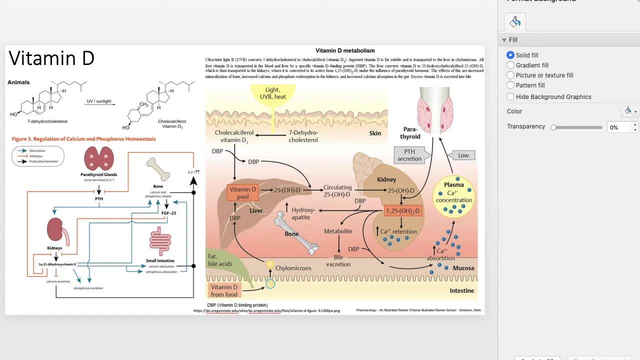 And you need to have neurons. Your neurons need calcium all the time, And so you need to maintain your blood calcium levels at a pretty narrow range as far as molecules go, And so to maintain that range we have hormones, Parathyroid hormone being one of the main ones. 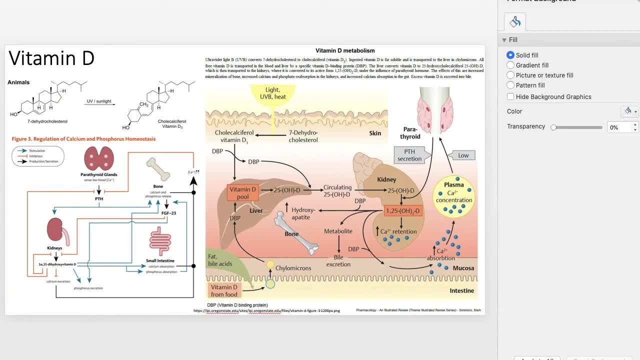 That can then drive either. So let's say, your calcium levels start dropping. Well, then your parathyroid hormone goes up, It gets secreted by your parathyroid Duh And then it goes to your kidneys and causes your kidneys to not excrete calcium. 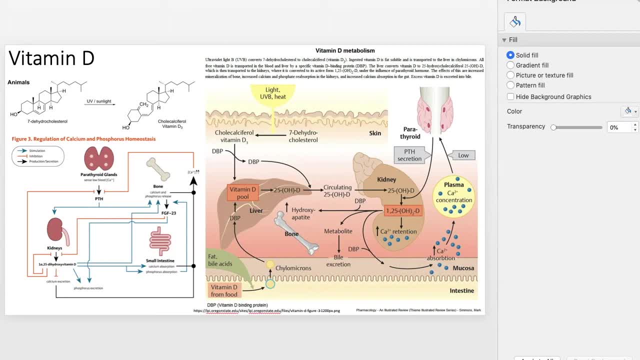 So they kind of hold on to it. They do get rid of some phosphorus, But in this case we're dealing with calcium, And then you are going to also. You don't want to get rid of calcium, So you want it to stay in your blood. 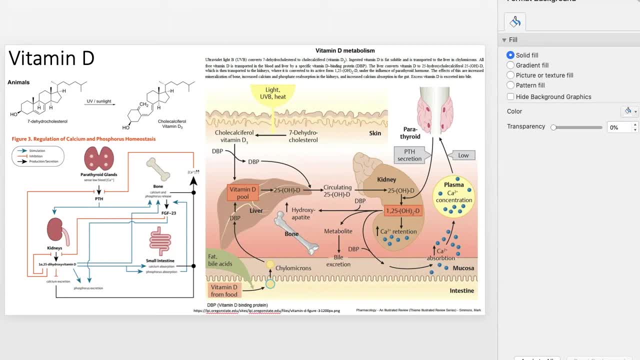 And you want to be absorbing as much as you can. So your small intestine begins It's able to better absorb calcium as well as phosphate- Really interesting stuff. So you can kind of read all about that. Yeah, I like both these charts. 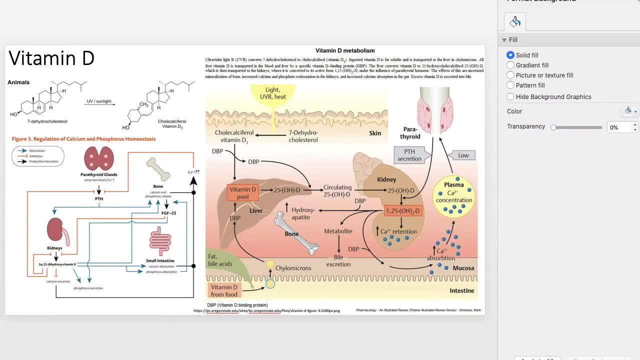 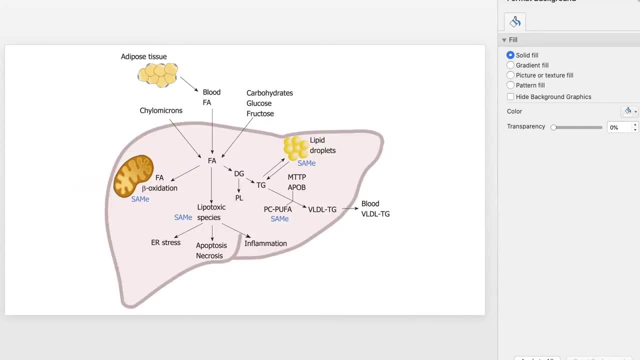 They're pretty cool. I'm basically reading it this way: Fucking sterols and cholesterol. I wanted to briefly talk about this, But I mean, we've got to talk about your liver and your fatty acids And we've got to talk a little bit more about your LDL and your HDL and all that good stuff. 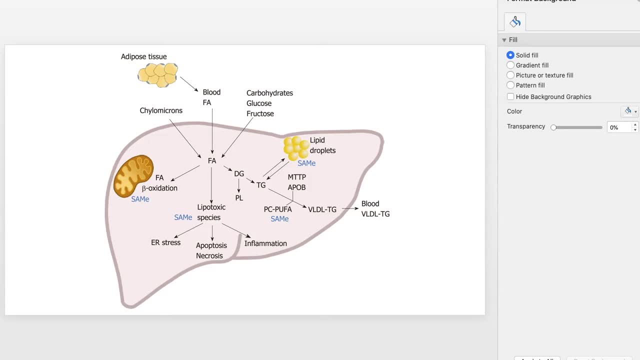 Because a lot of people take this class, actually want to be doctors, So we should probably talk about it. So here we've got FA, Fatty acids And where they're going to go. Okay, So basically we're going to follow these over here. 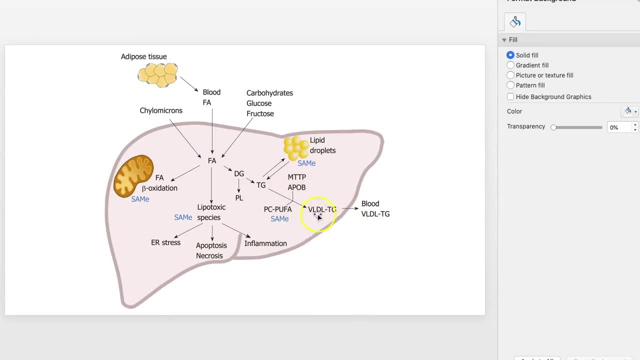 And we're going to generate some low-density lipoprotein. Sorry, I had a brain fart, But there's a lot of variety going on here And it's really Imagine, if you have, The way, that I help understand my brain. 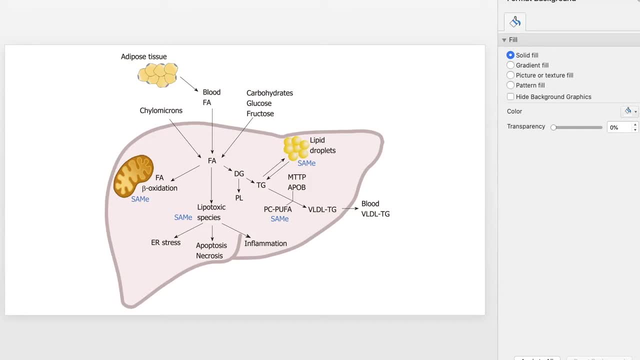 What The way I can get my brain to understand this better is to think about if I had, like, a high-fat diet, Okay, So somebody who All they do is go to McDonald's And they just eat Super fatty stuff all the time. 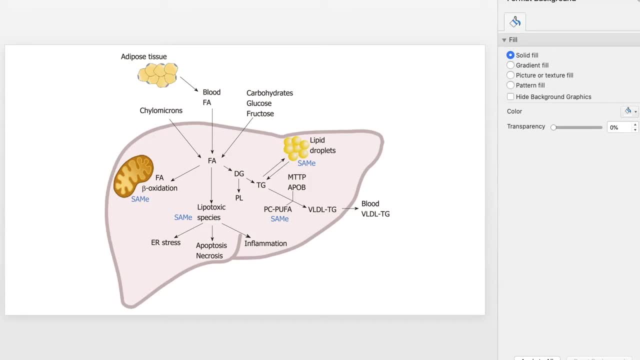 So I'm not really worried about caloric intake. I'm interested more in the actual content of the nutrition they're taking in, And the content is a lot of fats And a lot of fatty acids, Not as many carbs, So there are always some. 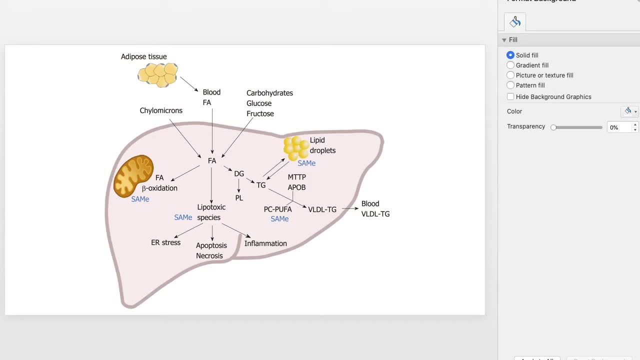 Not a lot of protein, Not a lot of other nutrients. So you're just getting a lot of fat. And what is your body going to do with it? Well, it needs to store it somehow, Right? You can't just have fatty acids floating around willy-nilly. 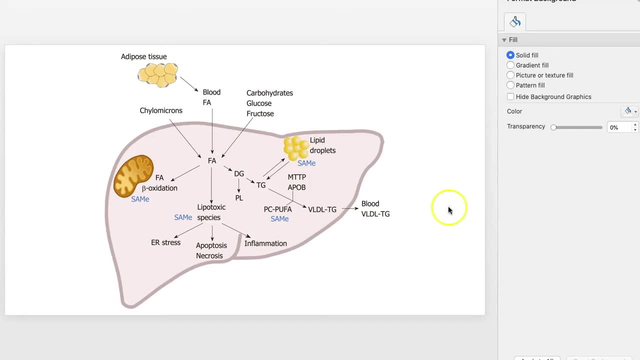 So you're going to send it to your liver, Because your liver does all kinds of stuff And it's going to do something with it. It needs to store it somehow, And so it's going to start storing it in the. It's going to start storing it in these chunks. 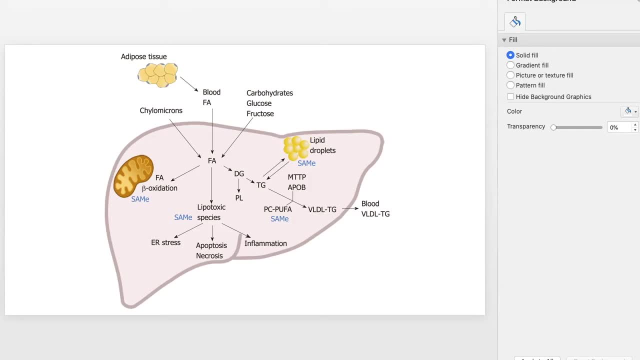 These big spheres- basically It's different sizes But different sized spheres- of lipoproteins. Okay So, lipoprotein being It has protein components, But it's also a bunch of lipids, And that's what we're talking about. 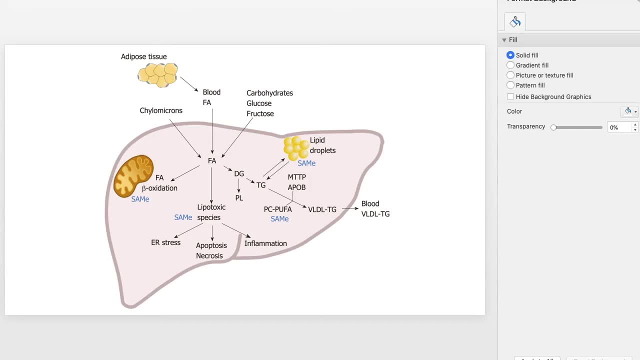 Lipids, Right, And so we're going to take our fatty acids, Take those big long carbon chains, And then we're going to store them, And so we need to talk about that. There is more than just LDL and HDL. 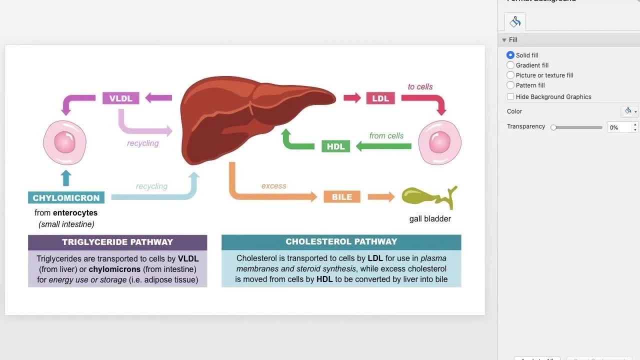 Okay, There is very low density lipoproteins, There's the chylomicrons And There's actually a variety. I used to talk about this a little bit more. There's in-betweens of all of these. 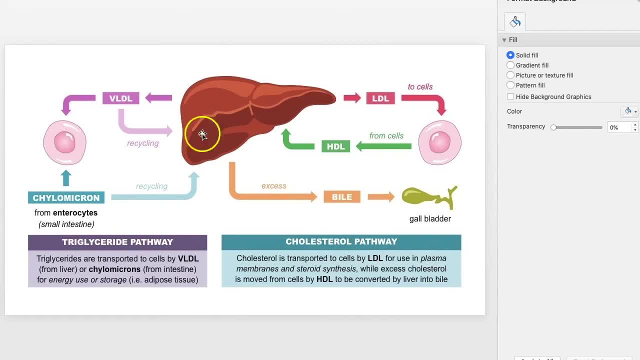 But basically I just wanted to cover the function of these lipoproteins. Okay, So you've got your cells. Okay, So this is like the rest of your body, So focus on here. So imagine this is a muscle cell or basically any kind of cell in the body. 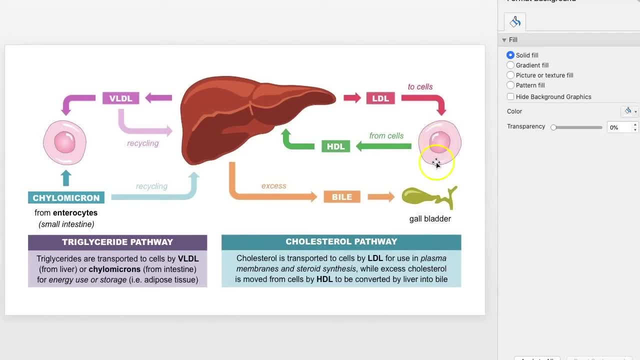 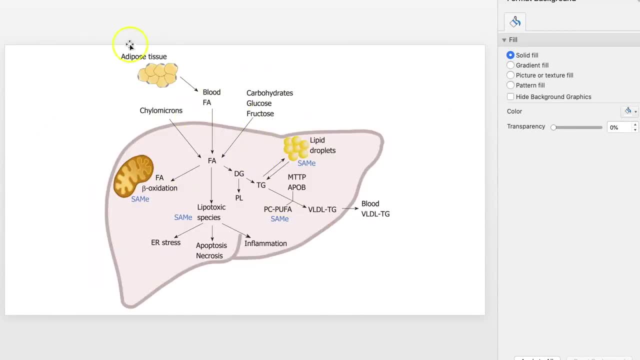 And if they have excess lipoprotein, they're going to make high density lipoproteins, They're going to send it out And it's going to head into the liver to be processed or whatever. Okay, So it can come from the liver. 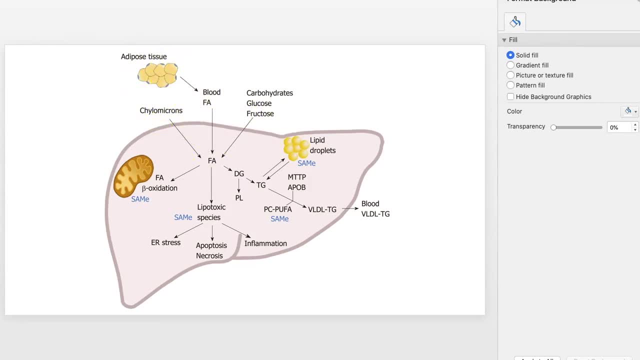 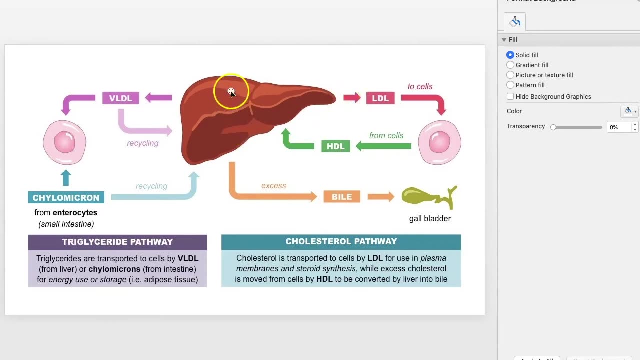 Either in chylomicron form or tissue is just going to come in there, And then your low densities is how you actually send it out to the cells. So there's a nice little pathway there. Now, if you actually want to go store it in a different way, you can make it very low. 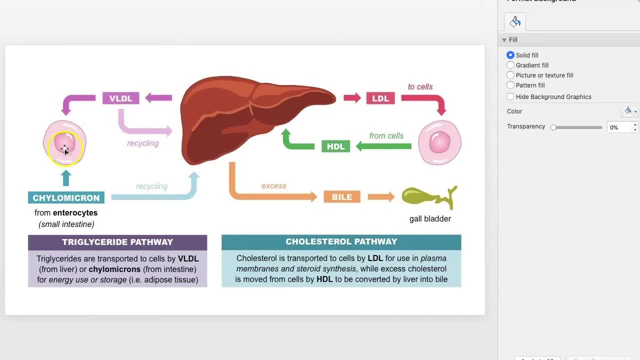 density lipoprotein and then send that out And that can either form chylomicrons or you can get chylomicrons So you can actually eat stuff, And that's where the chylomicrons come from, And they all just kind of end up in the liver. 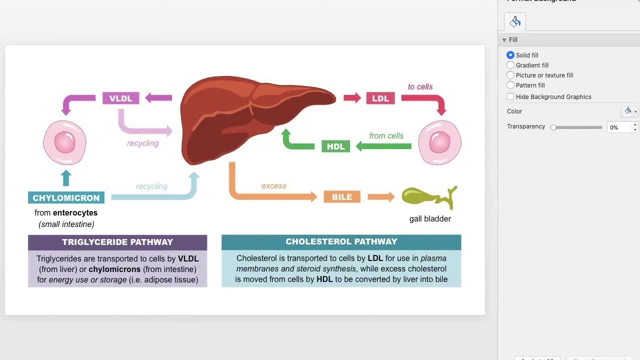 And if you have excess ones you can send it out. So if your liver is getting all fat and gross and full of gross stuff, your cells don't need it anymore. They're sending all this HDL in there. The rest of your body doesn't want anymore chylomicrons. 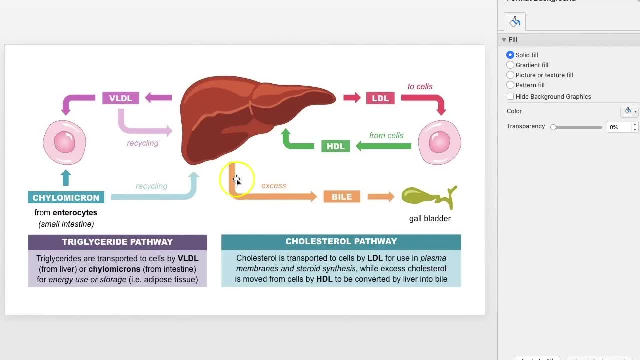 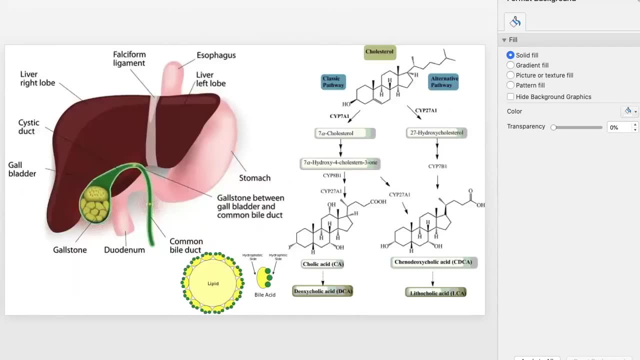 They're sort of sick of it And so you say, all right, let's get rid of it, So you can get rid of the excess in your bile And we need to talk about what bile is and what bile salts are. Too much McDonald's and you need to get rid of all that fat. 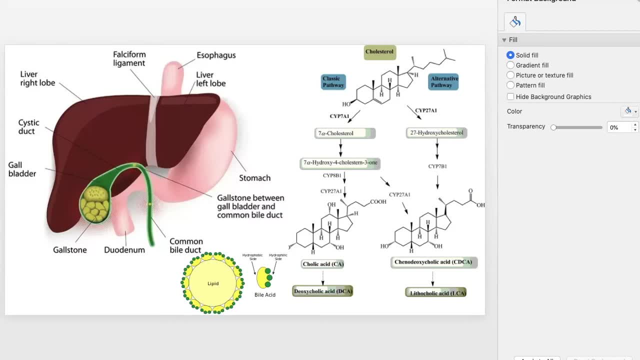 Okay, All right, Fine, Let's head to the liver. We're going to take all that excess cholesterol. Okay, So it doesn't have to be cholesterol per se, but we're going to stick with this. It comes from a different – it can head a couple different directions. 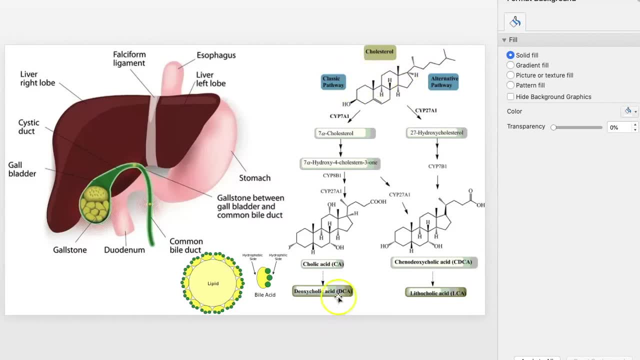 Okay, But basically you're going to end up with these colic acids. So either deoxycholic acid, DCA, or lithocoic acid – lithocolic acid Man. some of these terms are so hard to say. 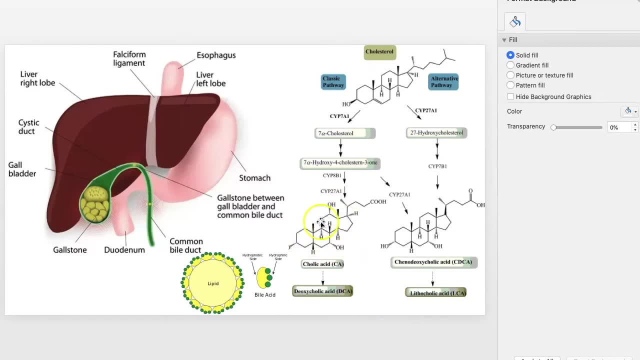 But notice, you still have that nice ring structure, You still have that steroid structure here, And what you can do is you're going to then take those things And you're going to basically smash them together with some proteins to kind of keep them together. 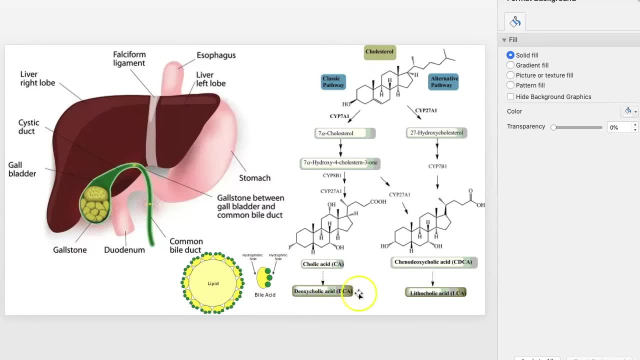 And that's what's going to form your bile acids, And so the DCA and the LCA that is going to form your bile acids. So I have this little picture here of what a bile acid looks like, And then what you can do is you can either get rid of it that way, send it out through your intestines. 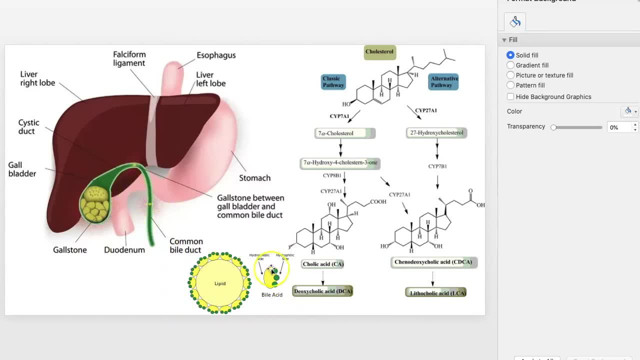 You poop it out. But also, what's really nice is bile acids have – they are amphipathic, So they have a water-loving side And a hydrophobic side And you can use them to sort of form almost like soaps or lipid layers. 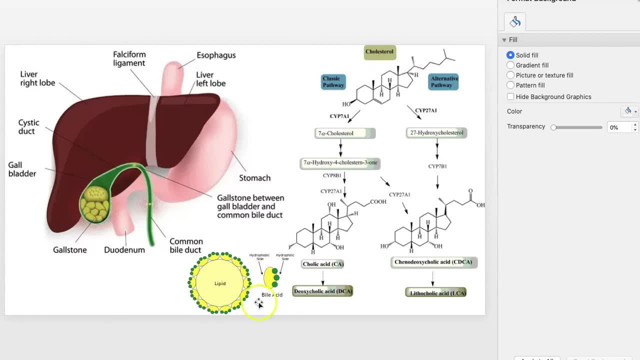 And you could take larger chunks of fat and actually use bile acids to kind of grab onto those and sort of deal with them And you kind of wrap it around there And then you can get rid of large fat chunks or other lipids that you just have access of. 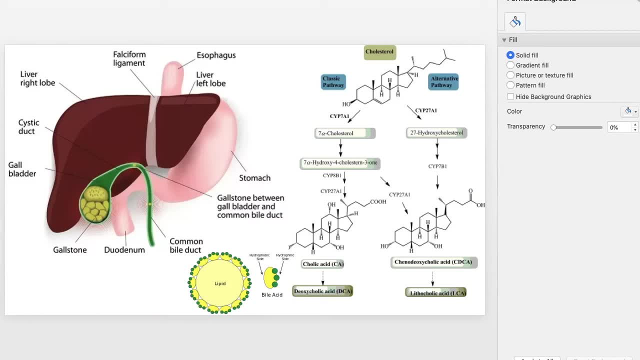 So it's really, really nice. Now I would like to cut to a video that sort of talks a little bit more. It's the rest of the osmosis video that I showed earlier. It talks a little bit more about fatty acids and lipids and just how these things are actually stored in chylomicrons. 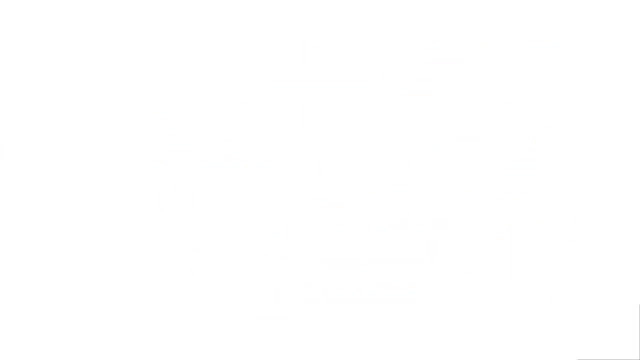 It's really, really good. Let's cut to that. Fats have a three-carbon backbone called glycerol, as well as fatty acid chains. The fatty acid chain is basically a string of carbon and hydrogen atoms. When an OH group from the glycerol molecule binds to a hydrogen from the fatty acid, an H2O or water molecule gets released. 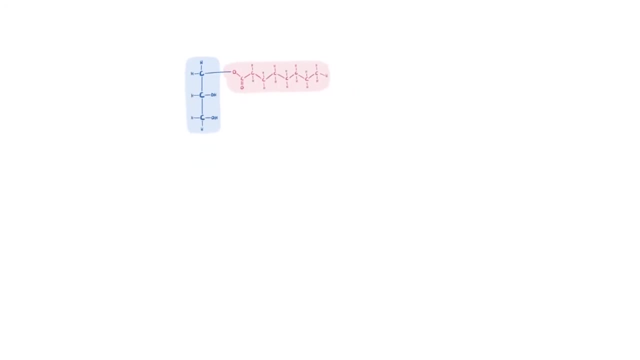 And the two molecules link up. If this happens once, the result is a monoglyceride. If it happens twice, it's a diglyceride And three times makes a triglyceride. Now there are various types of fatty acid chains. And one way to categorize them is by their length, In other words, how many carbons they have. Short-chain fatty acids have 2 to 5 carbons, Medium-chain fatty acids have 6 to 12 carbons, And long-chain fatty acids have 13 or more carbons. 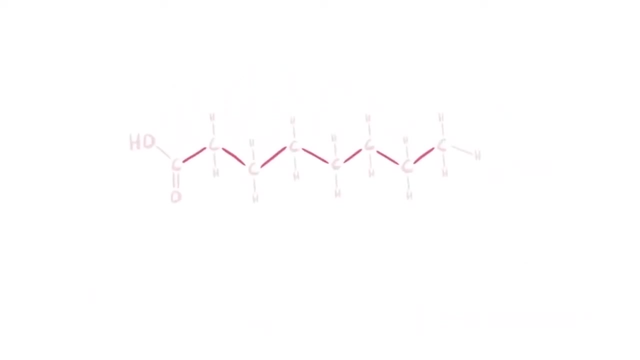 Fatty acid chains are also categorized by the bonds connecting the carbons in the chain. A single bond is just one bond between the carbon atoms, And when a fatty acid chain has only single bonds, it's called a saturated fatty acid, Because it has as many hydrogen atoms as possible. 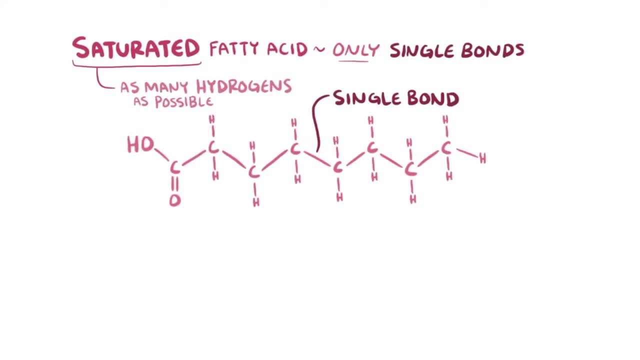 Or it's saturated with them. Triglycerides with saturated fatty acids are nice and straight, so they pack together really well And as a result, they're usually solid at room temperature. And the longer the saturated fatty acid chain, the more likely it'll be solid at room temperature. 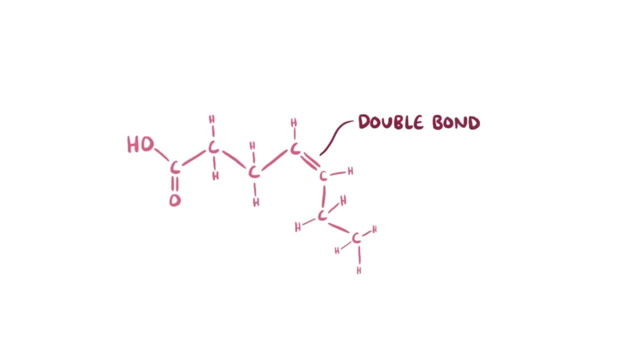 Carbons can also have double bonds between them, though, And when a fatty acid has one or more double bonds, it's called an unsaturated fatty acid, Because it's not saturated with hydrogen atoms. For every double bond, there are two fewer hydrogen atoms. 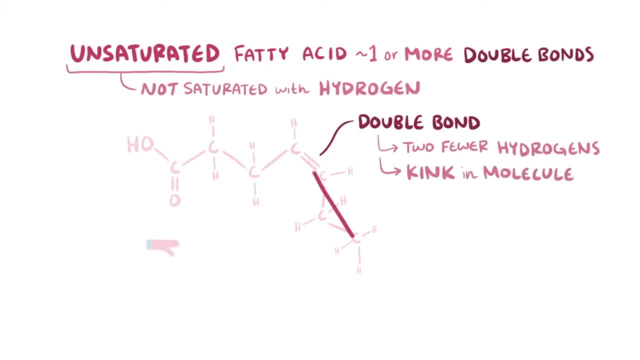 Also, a double bond causes a kink in the molecule, So the triglycerides don't pack together as nicely as saturated fatty acids. As a result, unsaturated fats are usually liquid at room temperature. Unsaturated fatty acids can be further classified according to the number of their double bonds. 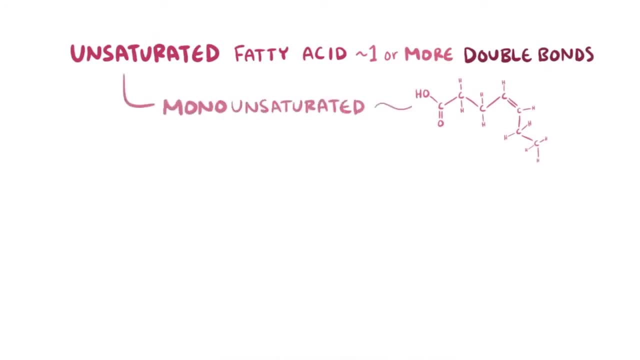 Monounsaturated fatty acids are unsaturated fatty acids with just one double bond. Polyunsaturated fatty acids have two or more double bonds. Also, they can be classified according to their location as well, Since all these hydrogens can get kind of crazy looking. 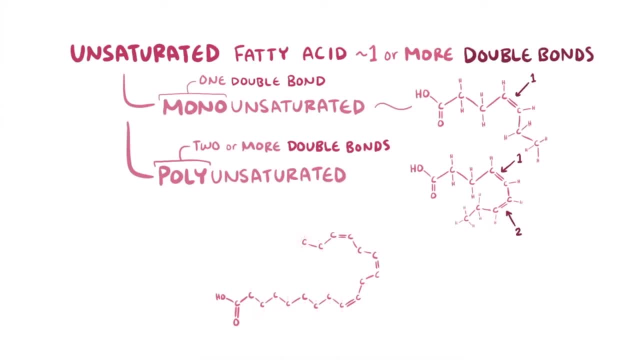 we'll just take a look. We'll just take them away for now. So another name for the methyl end is the omega end, And then we can count the number of carbons until the first double bond, Since this one is three. it would be an omega-3 fatty acid. 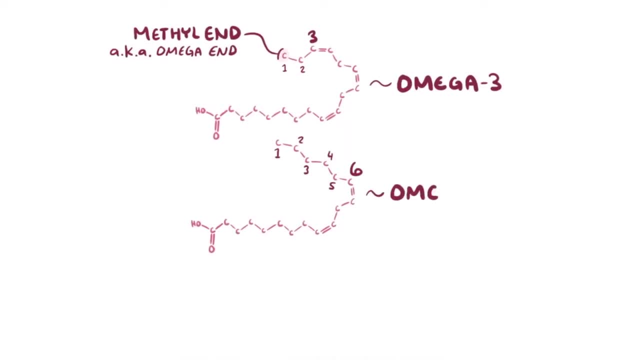 If the double bond is six carbons from the end, it's an omega-6.. And if it's nine carbons from the end, it's called omega-9.. Now, to make things even easier when looking at these molecules, I'm just going to show the bonds. 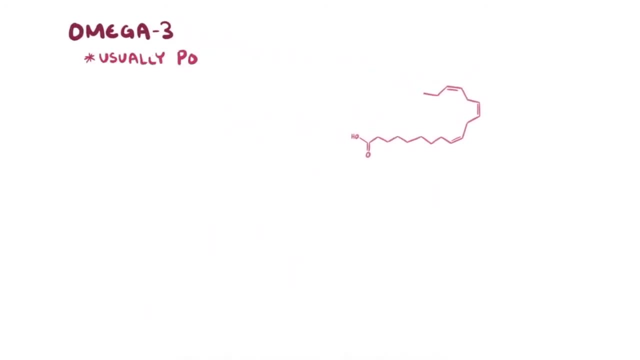 Alright. so omega-3s are usually polyunsaturated fatty acids and include alpha-linolenic acid or ALA, eicosapentaenoic acid or EPA, and docosahexaenoic acid, or DHA. 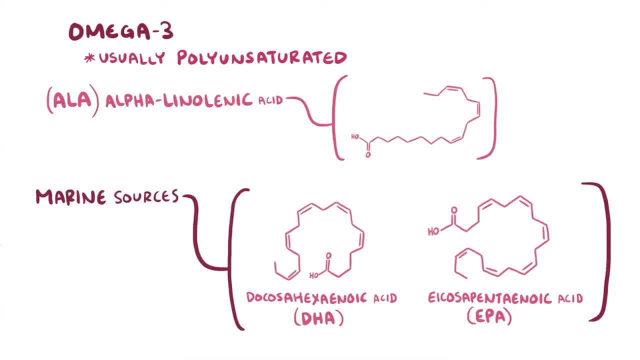 EPA and DHA are marine sources of omega-3s. They're produced by microalgae and end up in the tissues of fish like anchovies, mackerel salmon and sardines. Omega-3 is found in plants like flaxseed walnuts and canola and soybean oils. 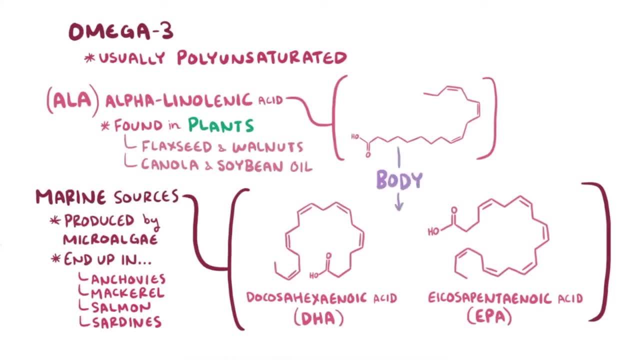 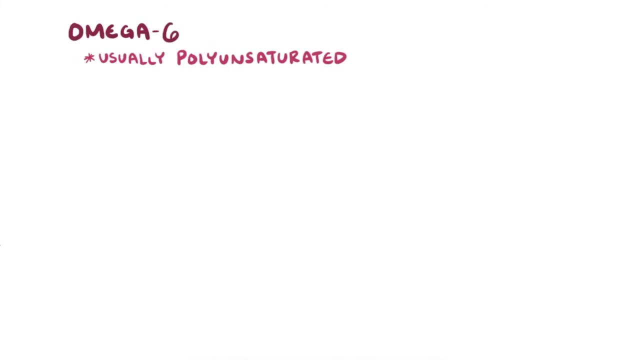 Our bodies can convert ALA into EPA and DHA, but it's an inefficient process that yields only small quantities, And that's why dietary recommendations include foods that have EPA and DHA. Omega-6 fatty acids are also usually polyunsaturated. 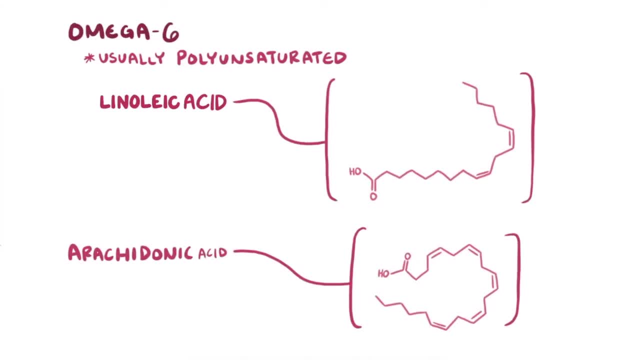 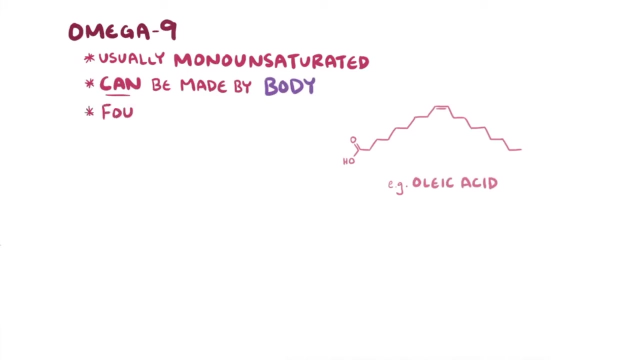 and include linoleic acid and arachidonic acid. Omega-9 fatty acids are typically monounsaturated fatty acids- example would be oleic acid- and these can be made by the human body. Foods like canola. 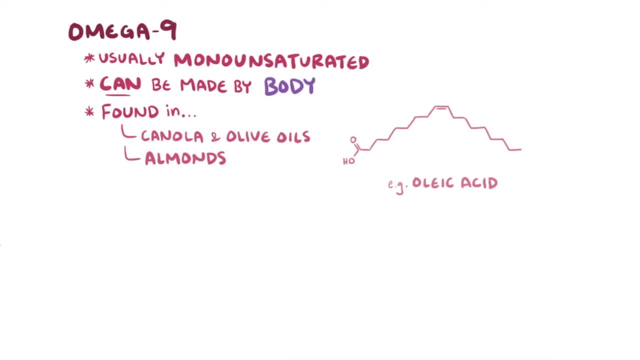 and olive oil, as well as almonds, contain omega-9s. Although some foods might have more of one type of fat than another, the truth is that all foods are made up of a blend of fatty acids. When you eat a food like peanut butter, 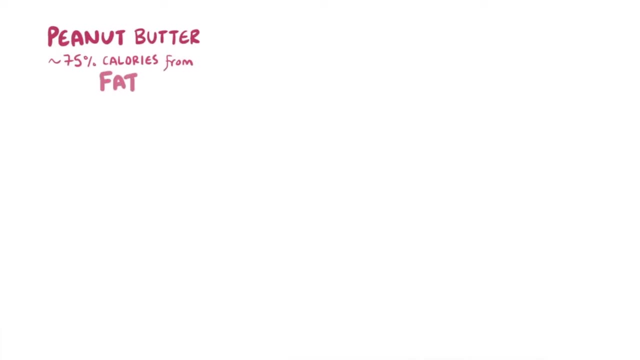 which has about 75% of its calories from fat. the body goes through a set of steps to digest and absorb the fatty acids. First of all, triglycerides are hydrophobic, so they form large globules of fat, like what you see when you pour oil in water. Enzymes called lipases 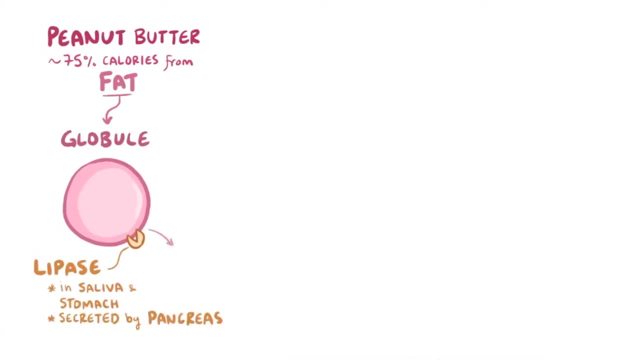 in the saliva stomach and secreted by the pancreas, can break down triglycerides into free fatty acids and monoglycerides. But working on the surface of a globule is inefficient. so to speed things up, bile salts produced by the liver break the large fat droplet into. 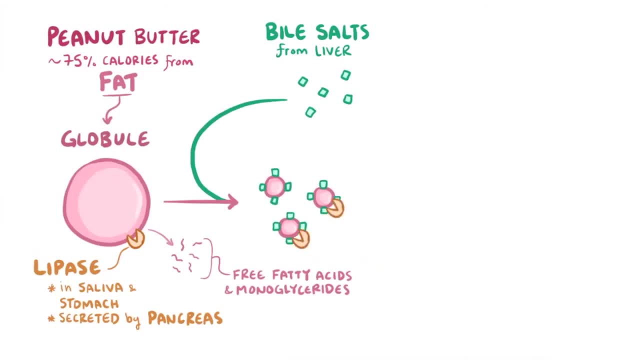 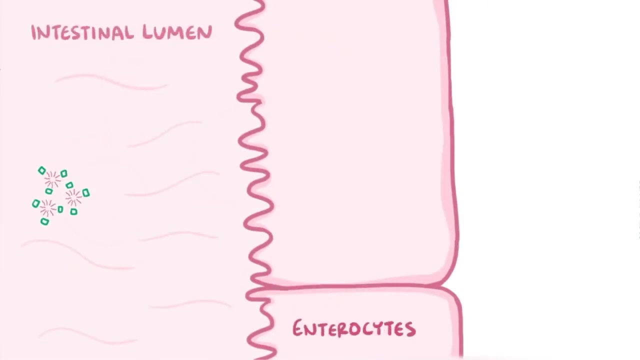 smaller droplets. Once the triglycerides are broken down into monoglycerides and free fatty acids, these self-assemble into mixed micelles which have a hydrophobic interior and a hydrophilic or water-loving exterior. The micelles glide through the watery environment of the intestinal lumen and reach the enterocytes. 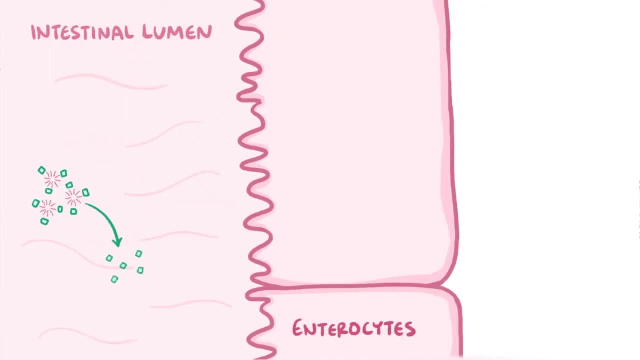 in the intestinal wall. When they get to the enterocytes, the micelles release the fatty acids and monoglycerides, which of course leads to the ingestion of fat, which leads to an increased levels of glycine. How many of these bioplastics are found in the lipases? 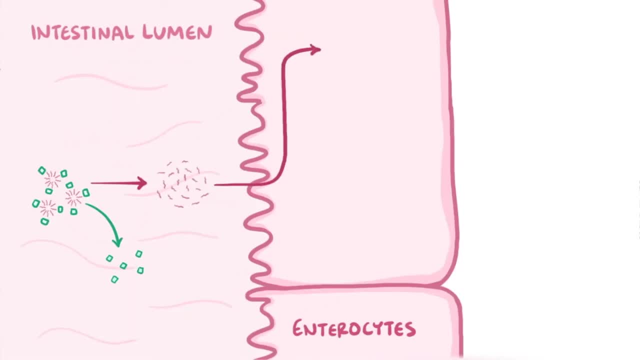 7,000.. which diffuse into the enterocyte. Inside the enterocyte, the fatty acids and monoglycerides reassemble into triglycerides and these get packed into a larger structure called a chylomicron. The chylomicron has lipids and proteins, so it's a lipoprotein. 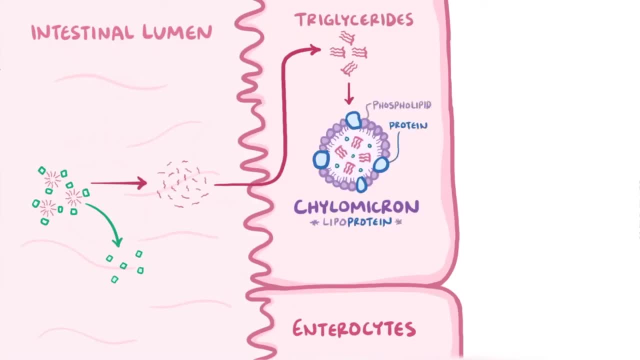 It has an outer membrane with phospholipids and proteins and a hydrophobic core that has triglycerides, cholesterol and fat-soluble vitamins A, D, E and K. The chylomicron then leaves the enterocyte, but it's too large to get into the endothelial. 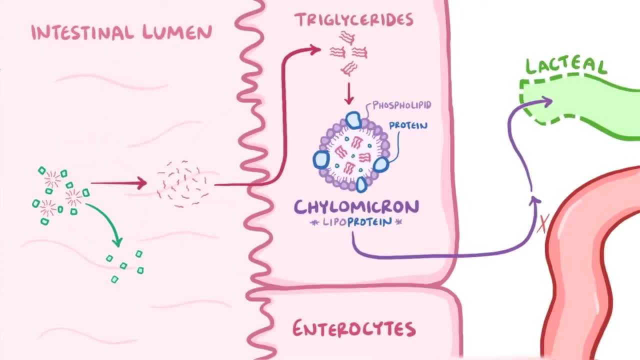 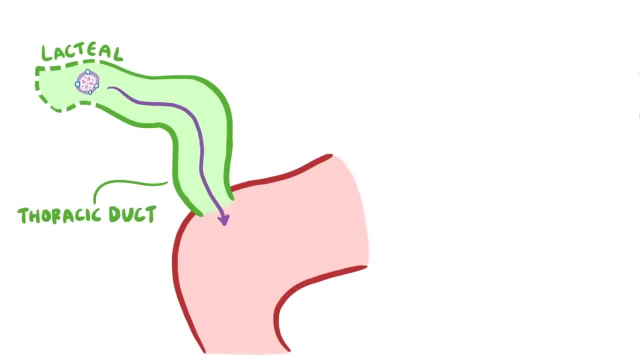 cells. so instead it enters a nearby lymphatic capillary called a lacteal. From there the chylomicron floats in the lymph and flows into the thoracic duct and then gets dumped into the blood, essentially bypassing the portal vein. 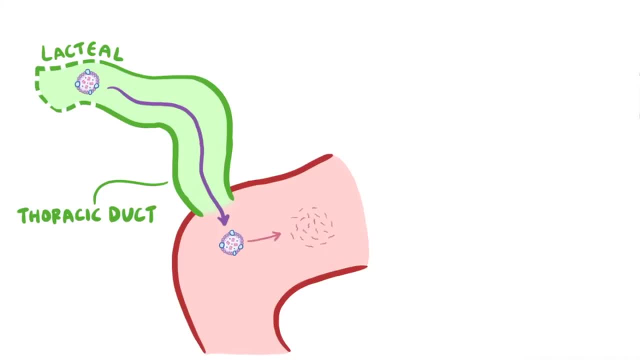 Once in the blood, the chylomicron releases fatty acids and monoglycerides in peripheral tissues like muscle, which use them for energy, as well as adipose tissue which can store them. After delivering the triglycerides, the chylomicron shrinks in size and eventually gets engulfed. 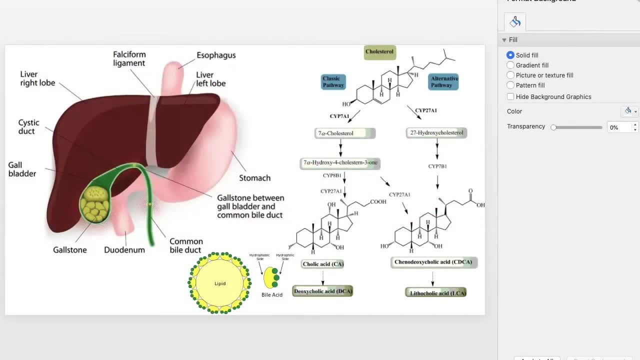 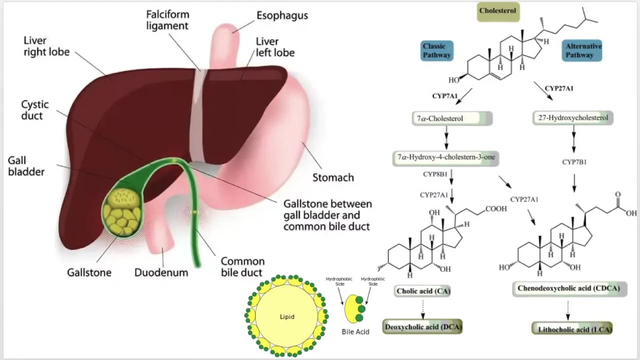 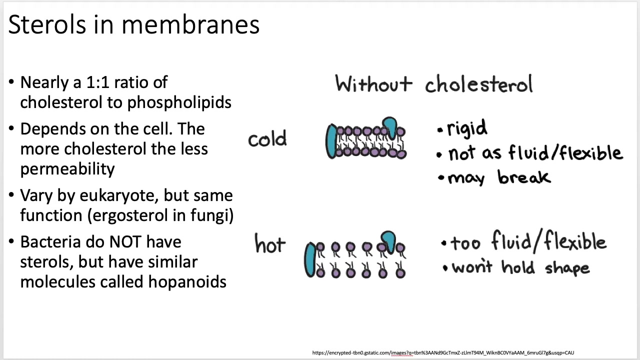 by the liver. This is a very common problem in the body. The last thing I want to talk about is actual membranes and membrane structure. This is something I like to talk about when I talk about lipids, because they're so intrinsically. 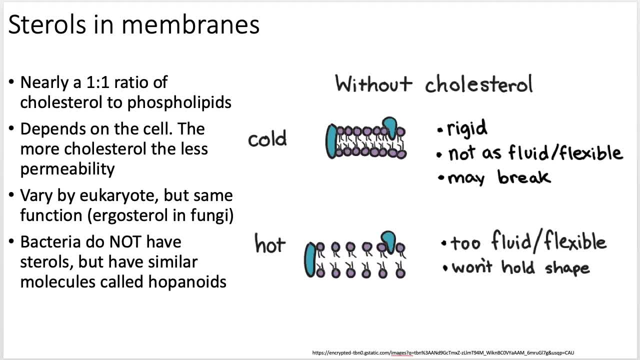 tied The idea of having a phospholipid and a phospholipid bilayer and they just come up a lot, so we need to talk about that. Off of that, we're actually going to talk about the function of membranes as well. 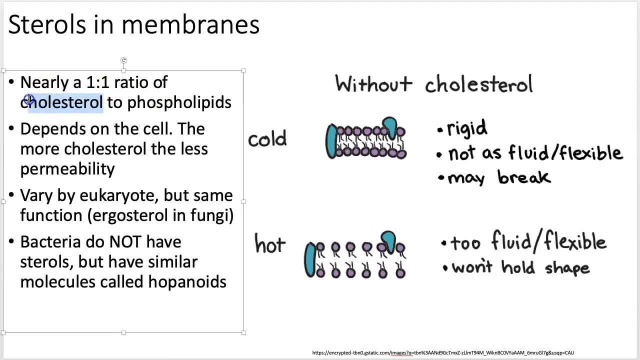 Now sterols and membranes. Cholesterol is the one that's mainly in humans. Other creatures have different kinds of sterols, so ergosterol, and funguses. Plants have a bunch of different sterols, Bacteria have hopanoids, which basically say the exact same purpose. 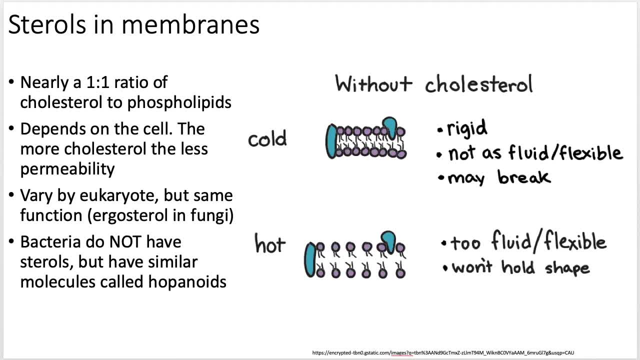 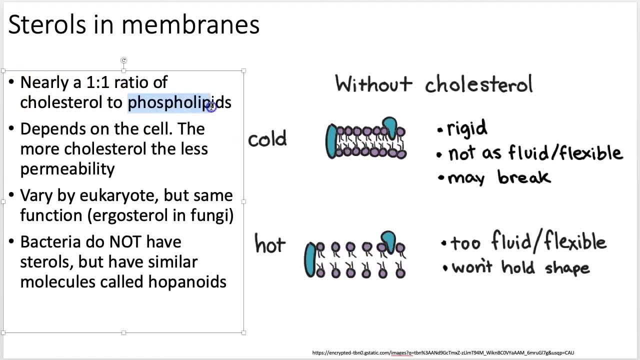 It depends on the cell, But phospholipids kind of explain the actual structure of it a little bit better, so that's why we make you learn that. But it is more of a one to one ratio, honestly, And the function of adding your cholesterols or whatever sterol you're using, into the 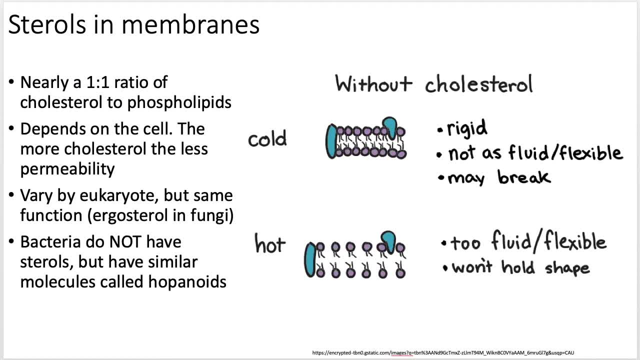 actual membrane is. it serves a couple purposes, but basically it makes it more structurally sound when you have adjustments in temperature, So if your phospholipids are really, really cold. so this is assuming that there is no cholesterol there. 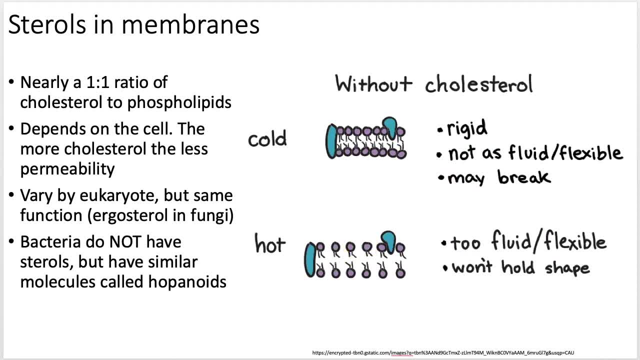 So maybe you don't have any cholesterol, Maybe you have a lot of fat in your diet or your body is having a lot of trouble generating fat, Maybe you have some kind of metabolic disorder, or maybe you're anorexic or whatever. 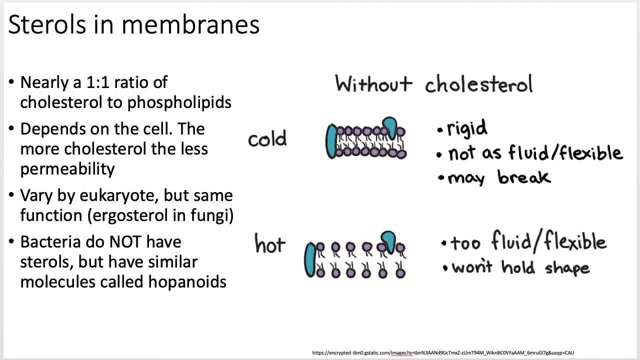 And it's. I'm not trying to downplay that, but if you're not getting enough fats in your diet and if you don't have enough nutrition in your diet, your lipid bilayers are going to fail, And if your lipid bilayers fail, you die. 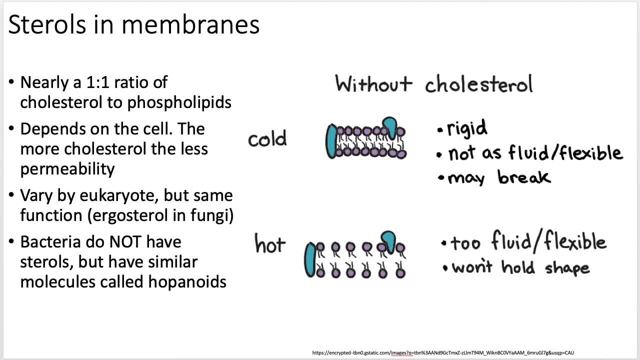 And so that's one of the first things that can start to go. But it's what your body's going to sacrifice to make too. So if you don't have cholesterol, if it gets really cold, you can imagine All the phospholipids. they stop vibrating as much, because that's what cold is right. 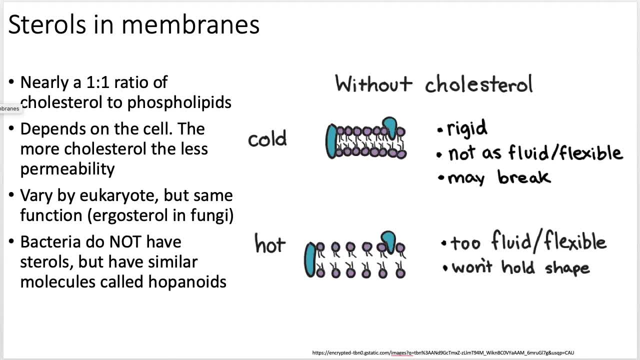 And it's the lack of vibration And it gets really rigid and it can shatter because it's so cold, It's kind of frozen. Now if it gets too hot as well, then they can sort of fall apart. And so what cholesterol does is it sort of bridges the gap between those two things. 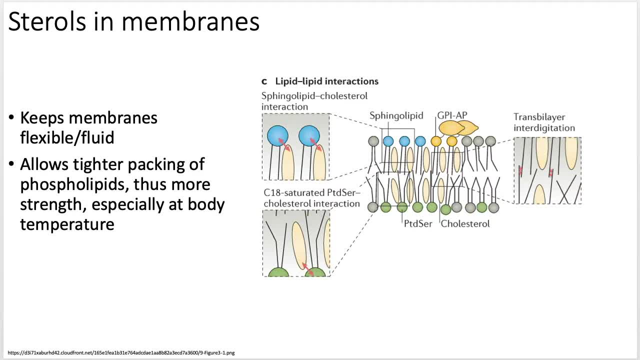 I have a graph in a second that's going to kind of show that a little bit better. I got this from a paper. It's really good You can go on there and look this paper up. They're going to apply fluidity and flexibility to the phospholipid bilayers. okay. 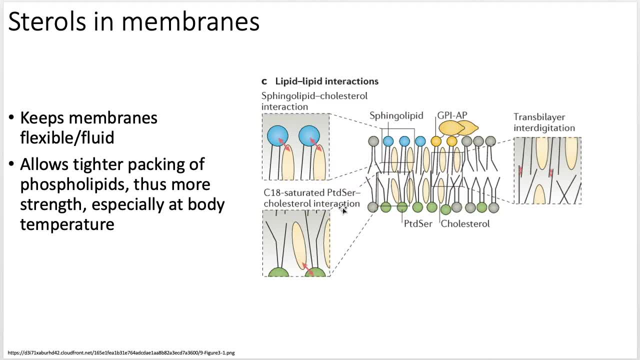 Okay. So it lets you pack them a little bit tighter and increases your strength And your body's really warm, right? So in humans and most mammals, we don't have to worry about getting too cold, right, Because we'll sacrifice energy to maintain our body heat. 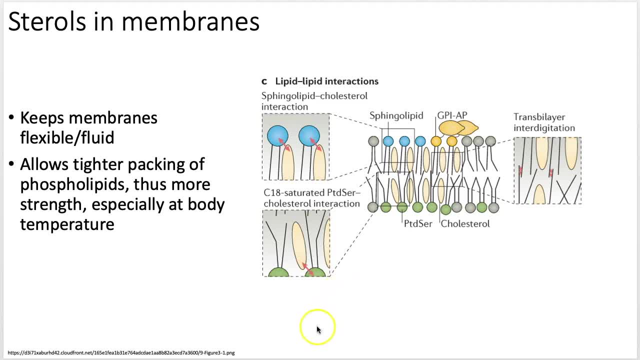 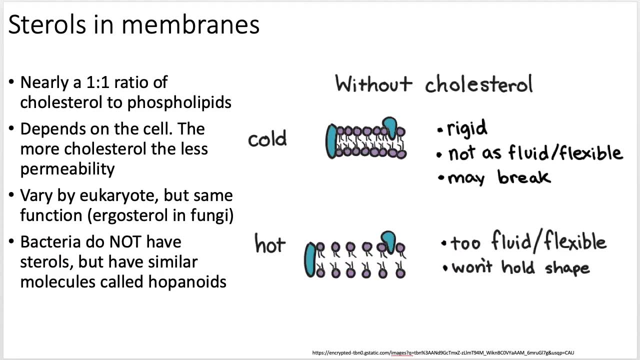 Not all creatures do that, but we do, And so we're generally dealing with warmth right, And so what can happen if we're too hot and we don't have enough cholesterol is that it gets too fluid. Your phospholipids won't hold their shape. 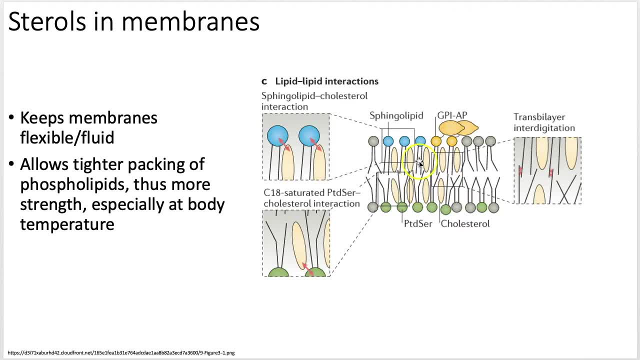 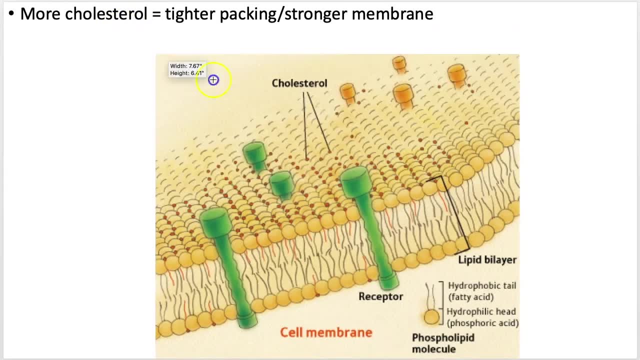 And so we're basically going to use our cholesterol. Cholesterol is to sort of hold. those act as the glue to hold the membranes together. And I have a picture here. I like this one. I know the quality is a little bit lower. 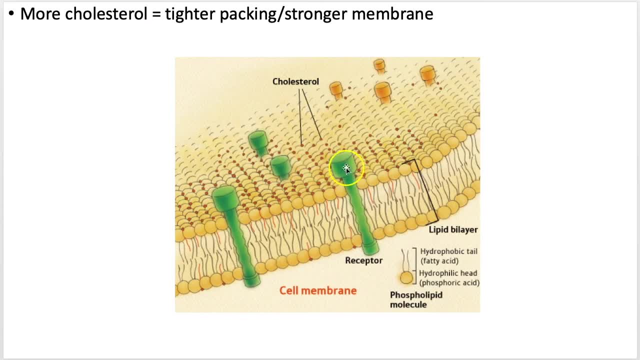 Some of the picture qualities for some of these just aren't great, but I like them. I don't know It. just I like this one a lot because it really demonstrates how much cholesterol there is. The red ones are cholesterol, How much cholesterol there is per phospholipid. 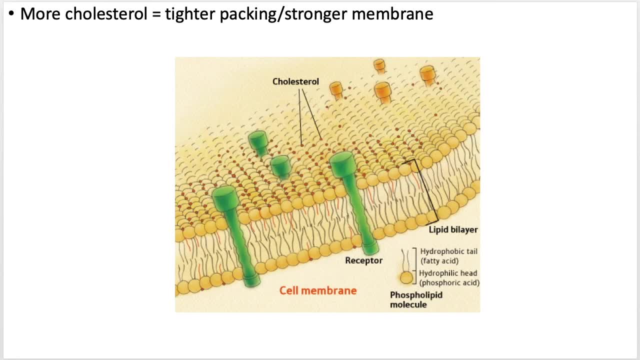 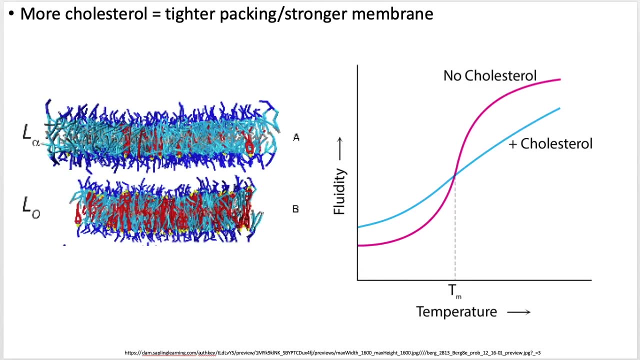 I mean, it's like a one to one, if not higher, ratio of cholesterol to phospholipid, So it's really really interesting. I like this one too, because it shows the receptors that are embedded on. That's what we're going to be talking about, but first let's finish talking about this. 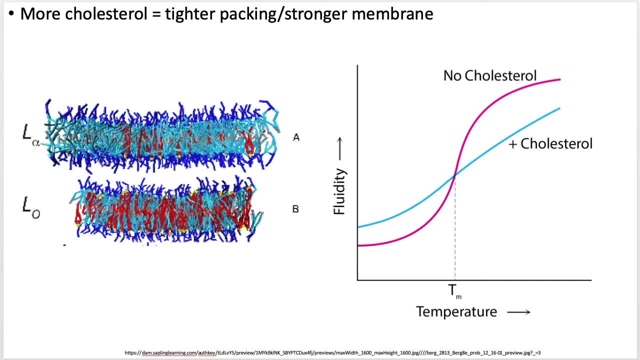 The more of the cholesterol you have, the tighter you can pack it and the stronger your membrane. Now, of course, there's a limit to that. You don't want. you don't want too much cholesterol in your phospholipids. 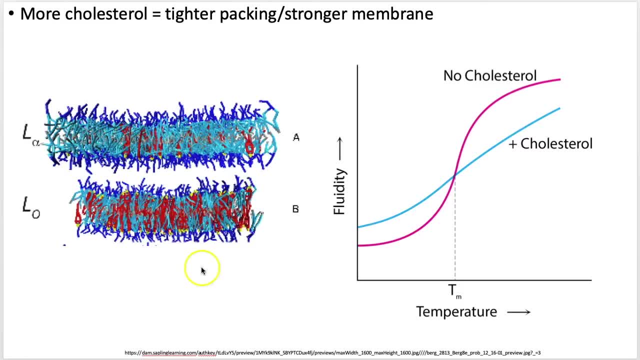 Hence why we're talking about. you know, actually being able to get rid of it, But biophysicists study this kind of structure And if you have cholesterol it really evens out. So in blue is the cholesterol here, And so as your temperature changes, 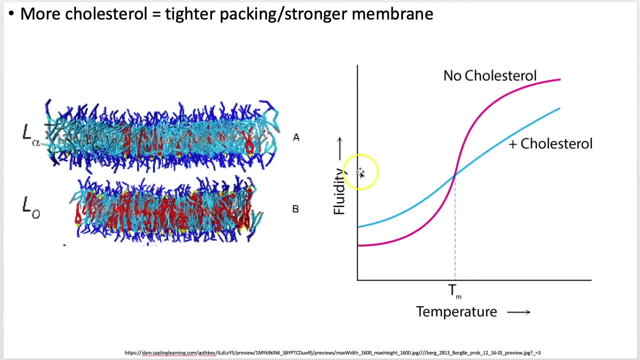 You can see the fluctuations in the actual fluidity, because you don't want your phospholipids to be too fluid- Right, That would be heat. So it can be too fluid, but you don't want it to be too stiff as well. 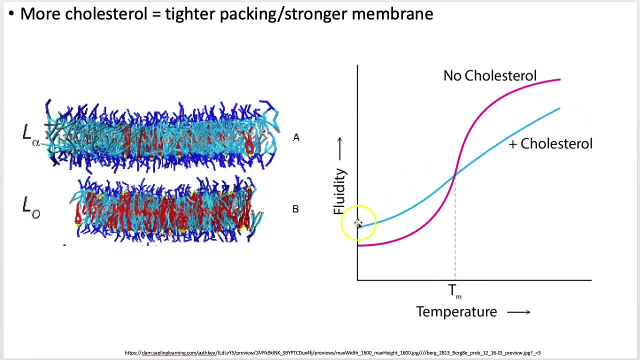 So you want that nice evenness And that's what cholesterol does at different temperatures. It just kind of flattens out the curve, because that's what's going on with COVID right now, But it just kind of narrows. It just makes it easier. 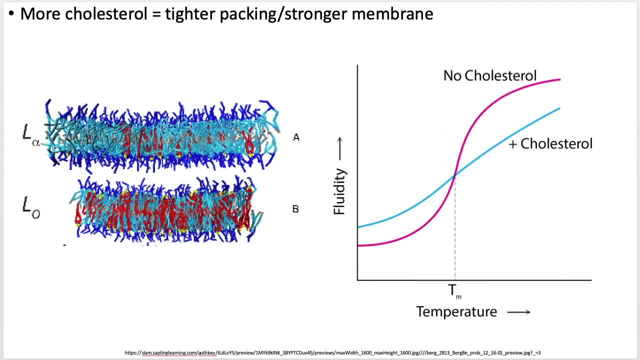 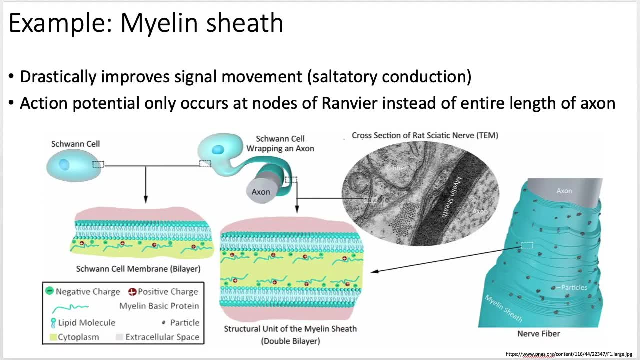 Okay, If you don't have cholesterol, you have these massive fluctuations And it can really change And it can really cause some damage. So that's bad. Damaged phospholipid virus- Bad. Let's do an example. So what kind of cells have a lot of these? 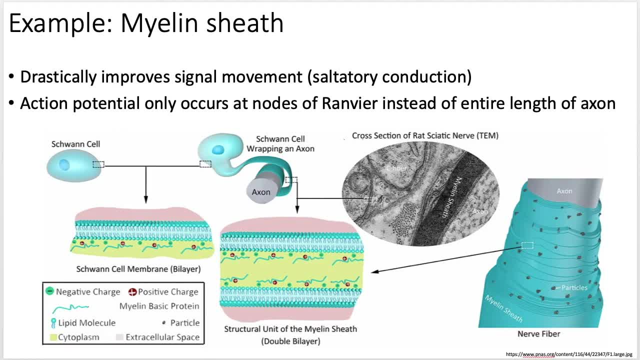 So your neurons need a myelin sheath. So you may have heard about this. if you've taken an anatomy and physiology course, You hear about your Schwann cells, which actually wrap up your axons. That's when you have the nodes of Ranvier, which is like the coolest term ever. 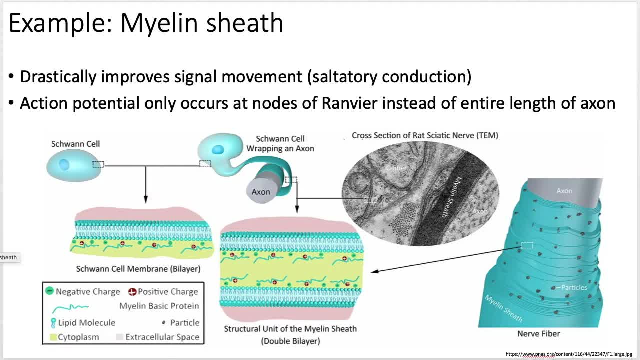 But basically you have that action potential Between positive and negative charge along your neuron, But you need to maintain that And in order to do that you have to have it nice and insulated, Just like a wire in your house or whatever I'm looking at. 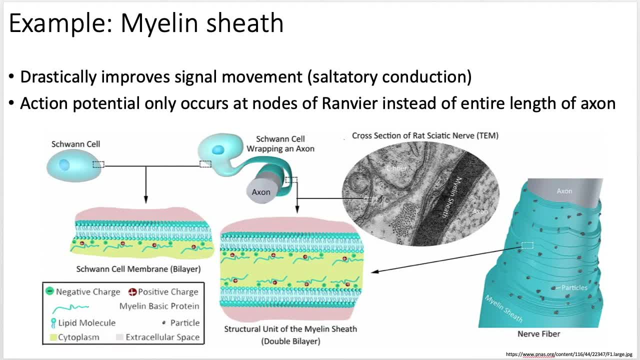 As if you guys can see me look at the outlet on my wall, And so you need to make sure that you keep it nice and insulated. Nice and insulated, And so that's what your myelin sheath's job is going to be. 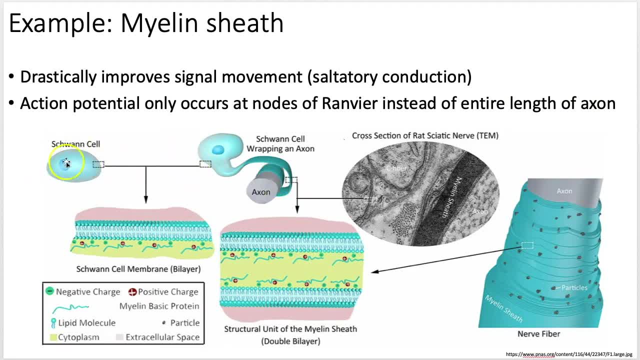 And the Schwann cells are really interesting. So they take their lipobylase. They look like a red, They look like a regular cell And look at that. They're going to stretch out and make It's still a lipobylase. 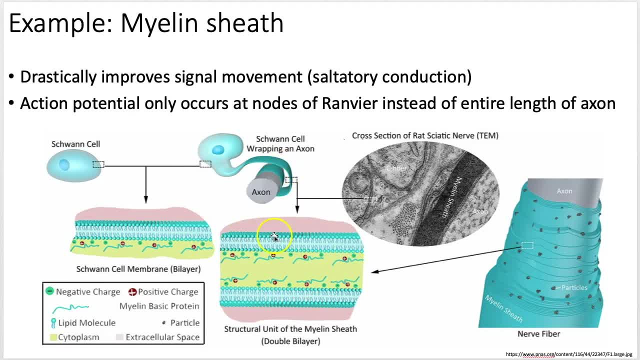 It's still two layers of cell, but it wraps around, So you end up with two lipobylases, So the rest of the cell is just crushed into this little area And it's really really cool And it wraps around over and over and over again. 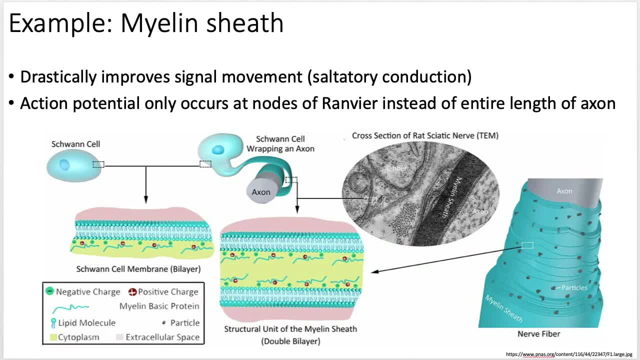 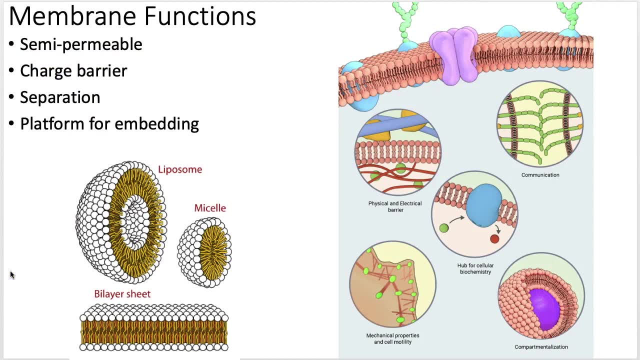 And it just really insulates that, which is really really cool. So insulation, that is one of the big functions. So a charge barrier is one of the membrane functions, But there are lots of other membrane functions that exist, Of course. 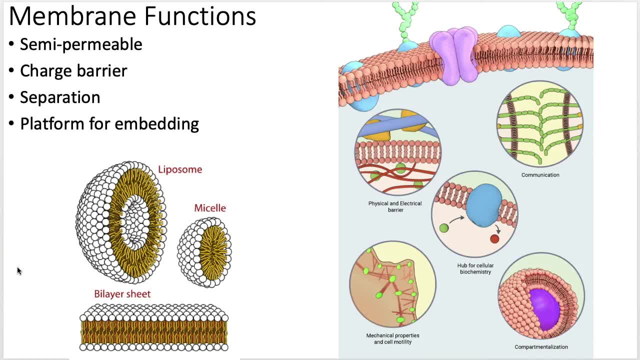 It's a semipermeable layer. You got to separate stuff. If you have a cell, you need compartments. It's just like your house: You need to have separate compartments. You don't have your bathroom and your kitchen and your bedroom all in the same room if 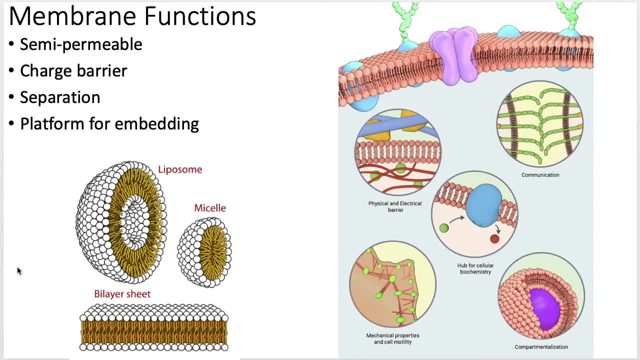 you can afford not to. I mean, of course, some people have that, But if you can avoid it, you want to, because you don't want where you poop to be right next to where you prep your food, right, And so you need some kind of separation. 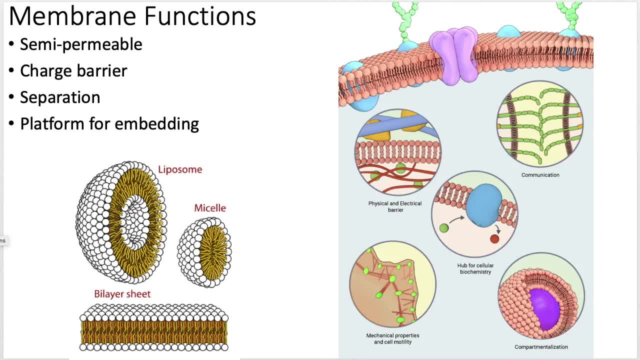 And cells are the same way, So if I need to do different things, I need to have separation. So, like your cells have a little trash can And with lots of really powerful enzymes that can cut stuff up, Well, I don't want those right next to, like my DNA or my ribosomes, because they're going. 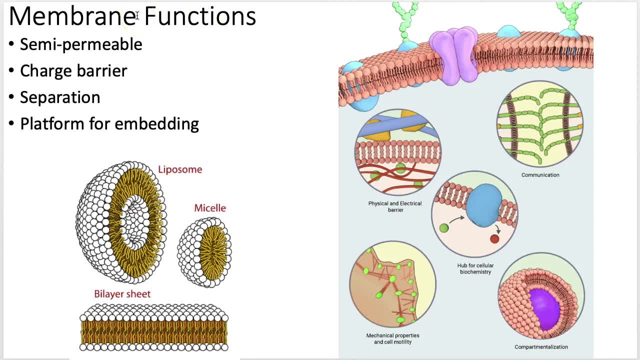 to cut those up, And so we separate them, And that's one of the main jobs of membranes. And they also act as nice little scaffold So we can attach things to them, We can stick proteins inside of them and do all kinds of fun stuff. 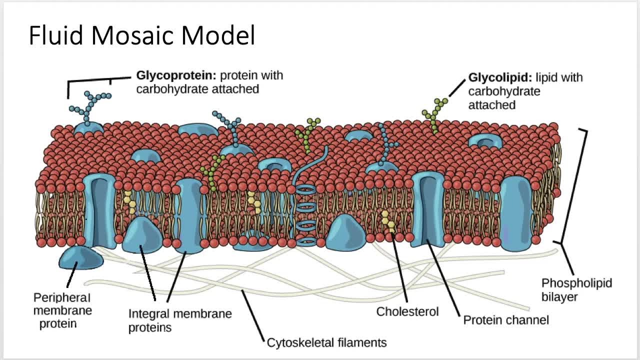 So, yeah, it's pretty fun. Now there are multiple models. The fluid mosaic model is the most commonly talked about. If you take cell biology, If you take cell biology, If you take it with me, then you will learn that there are other models and we talk a. 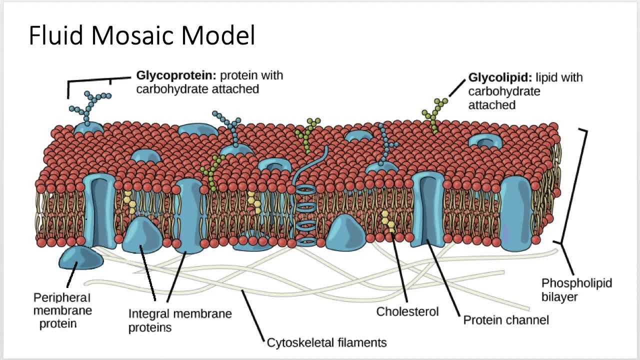 lot actually about membranes and membrane function, And so it's a kind of an extension of this actual talk that I'm giving right now. But the fluid mosaic model is generally the most accepted but it's more complex than what it is generally thought of. 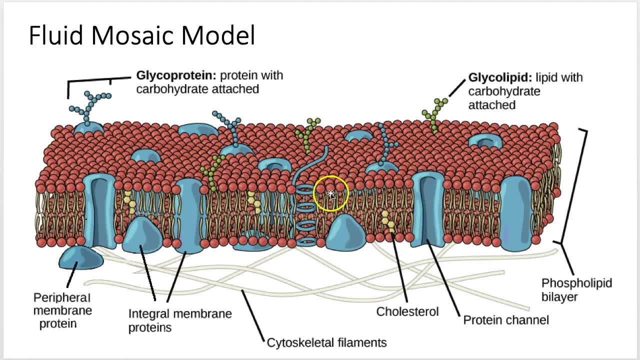 And so fluid mosaic just implies like. these are the way I see it is. these are like giant chunks of ice Or like if this was like a pool- I don't know A pool- And you threw as many beach balls as you could fit in there. 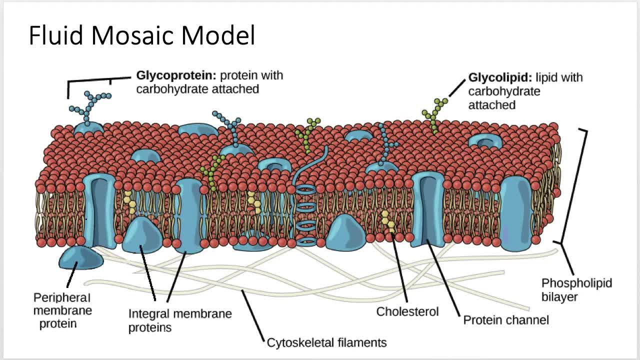 And then you have like a bigger, like I don't know a person or a giant inflatable thing. The inflatable thing can still move around the pool. It can kind of squeeze in between these beach balls, but you do have like some structure to it. 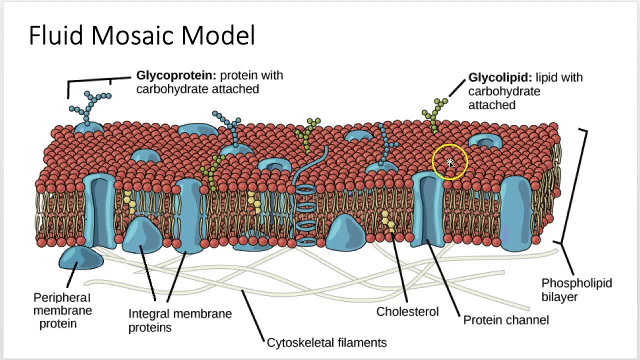 So the beach balls can move, but they are a level of structure And so that's basically the fluid mosaic models that things can move around. You can do all kinds of stuff to these proteins. Of course you can like oscillate them. 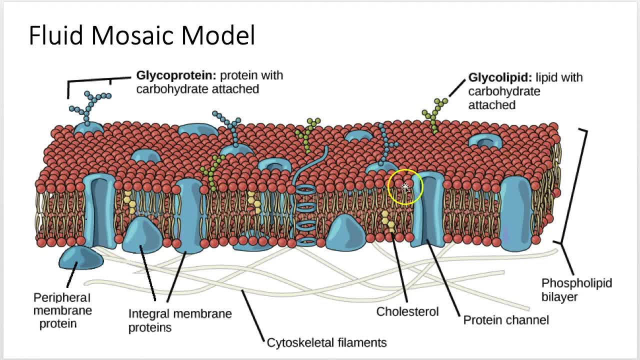 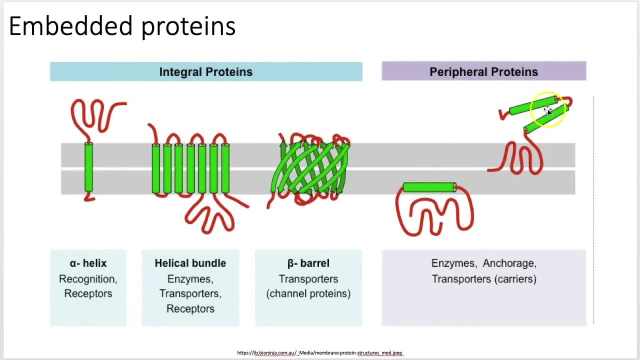 You can throw lipids on there, whatever, But the lipid bilayer itself is really, really cool and it's moving, It's actively doing stuff. You can stick proteins in it, They can be integrated, They can be peripheral, on the edges, though, you do usually have some kind of integral. 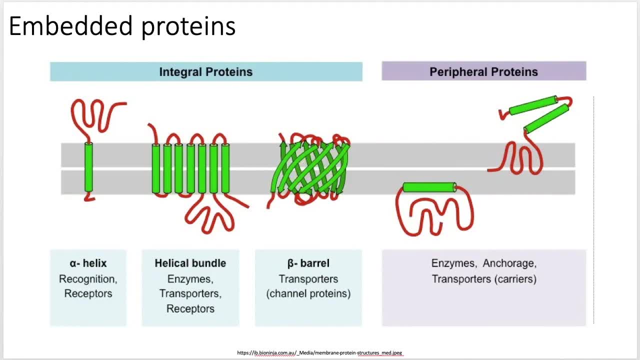 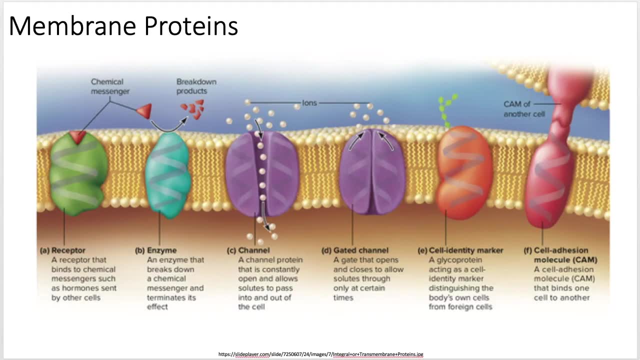 portion to it All kinds of stuff. I mean every receptor is going to be integrated, Every transporter or channel protein which I'm going to talk about, those, wow, that quality is terrible. Okay, It didn't look terrible earlier. 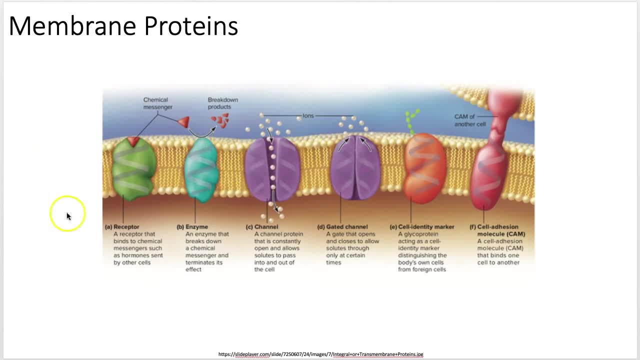 I'm so sorry. I'll just shrink it down and pretend that it doesn't look terrible, But you can have all kinds of stuff And classic biology exam questions are just asking like the different kinds of membranes and the different kinds of proteins, functions in membranes. 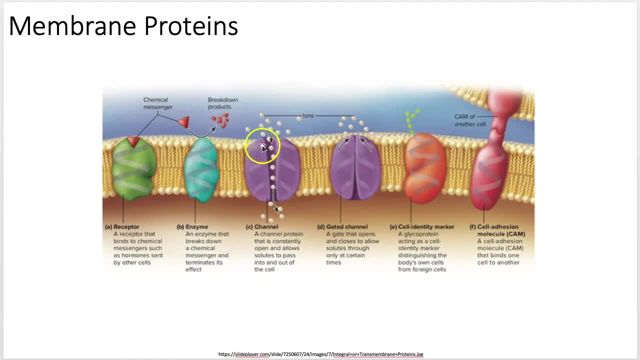 Are they going to act as a receptor? Are they going to act as a channel to let things in or put things back out? Can they talk to other cells? I mean viruses. use these right. The virus is going to have a ligand, or a ligand that's going to bind to a cell receptor. 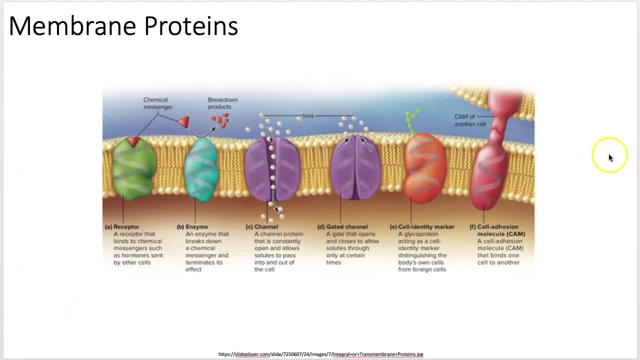 and it'll let the virus in. But that's all dependent on your phospholipid bilayer, or should we say cholesterol slash phospholipid bilayer? Yeah, It's really really important. As far as specifically what's happening, we need to talk about that. 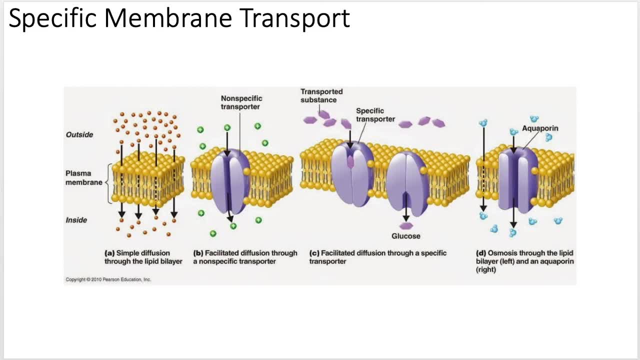 So there's different kinds of diffusion, right? So phospholipid bilayers are semipermeable. What does that mean? Well, some things can pass through and some things can't, So water is typically can just pass right through it. 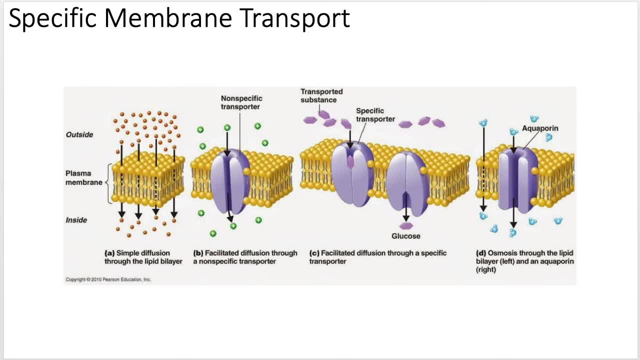 So it shouldn't just diffuse through. It's all about gradients, right? So if I have a bunch of something on one side and none of it on the other, it wants to get to the other side and I can take advantage of that. 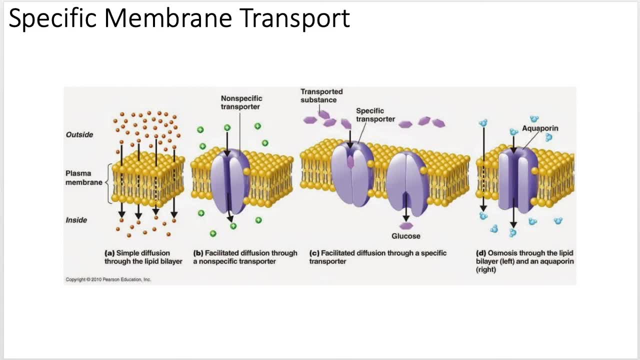 Which, when we talk about, like the electron transport chain, well charged molecules tend not to be able to pass through phospholipid bilayers because they have that big hydrophobic region right. So they're attracted to the hydrophilic regions where there's charges and they avoid the hydrophobic. 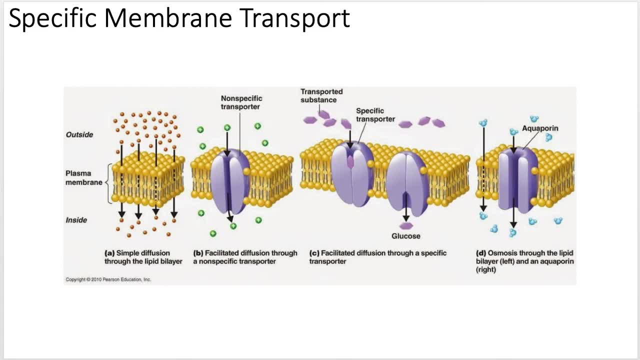 regions which can be really, really big, And so Hydrogen is on one side of a membrane and let them pass through and it acts as like a little water wheel and we can use that power And so that's so simple. diffusion is just if it can pass through. there's other molecules. 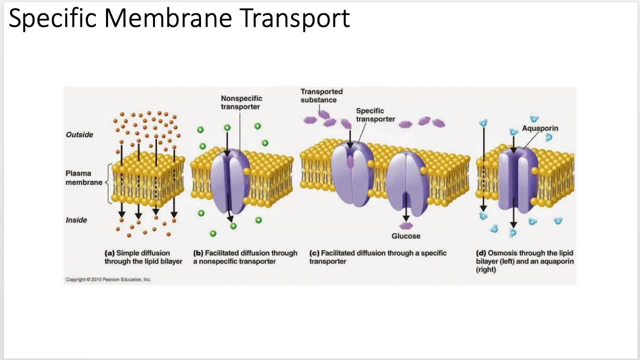 that can do that, Glucose being the other more common one- But sometimes you want a bunch of it to come through, in which case maybe I want a bunch of water to come in, or maybe I want a bunch of glucose to come in. 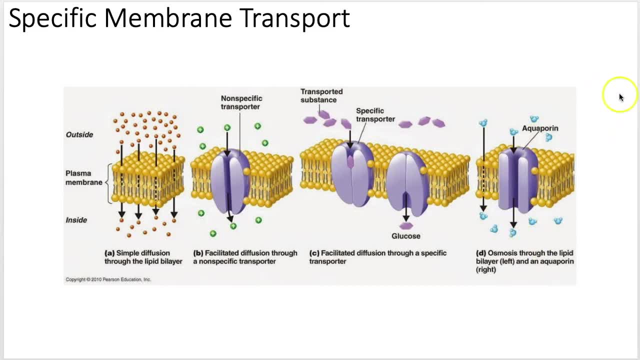 So I get a glucose transporter and that acts like this: where it allows like a giant thing- It's not aquaporin, but it lets like a giant amount come through faster than just simple diffusion- You can facilitate the diffusion. So you could have like: in this case we've got a non-specific transporter or you could. 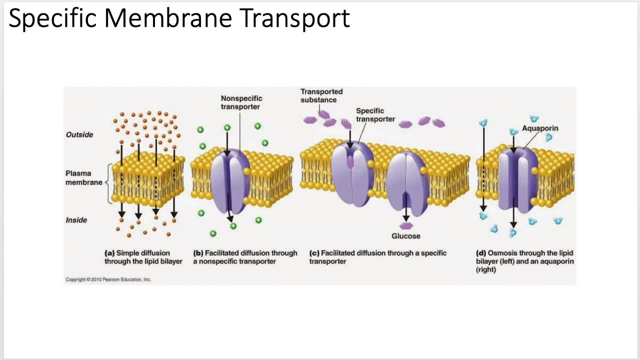 have a specific transporter. I mean, cells are so full of variety It's kind of awesome. But facilitated diffusion is just taking a protein channel and sticking it in the phospholipid bilayer so that something can happen That can be powered. 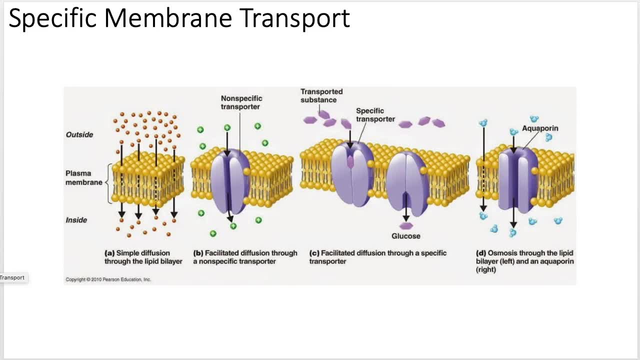 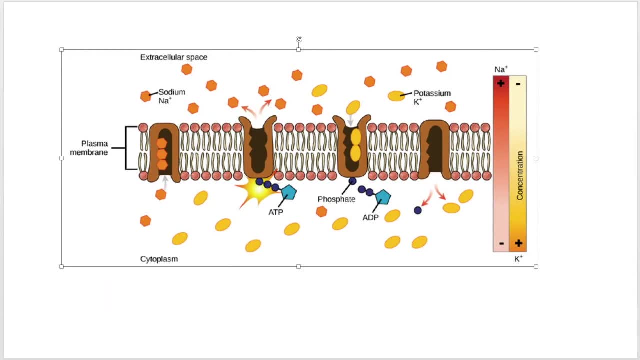 It can be unpowered. Usually, if you're powering it, that means that you want it to go against a gradient as opposed to not. Okay, Now, the phospholipid bilayer itself. I was talking about that. So when I spend energy with a specific transporter, that's usually if I'm trying to go against. 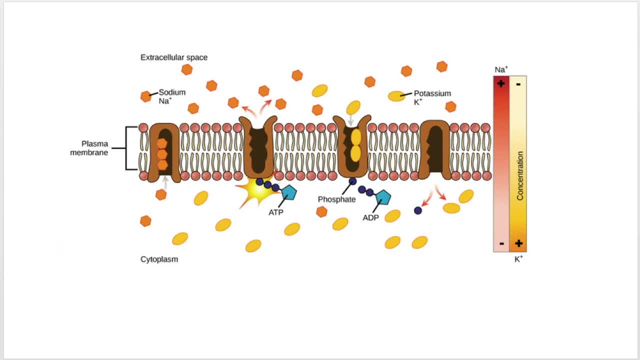 a gradient And that's where we see, like in neurons, when we have our sodium potassium pumps to put a bunch of sodium on one side and a bunch of potassium on the other, but the actual amounts of charges are different, So you end up with a more positive side and a more negative side. 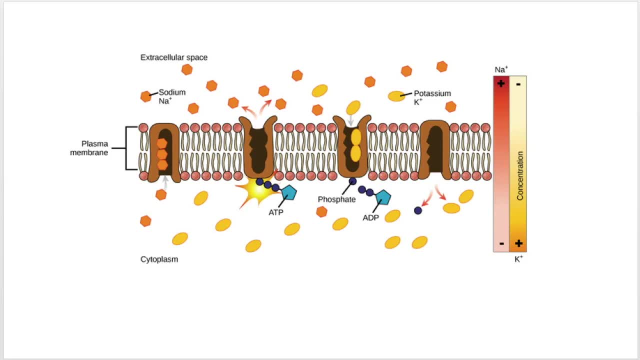 Okay, And then when you allow them to quickly switch, then that acts as a conduction mechanism and it allows the transport of information, basically, of which calcium is one of the very important molecules. at the end of that transmission, transport was the term I completely forgot. 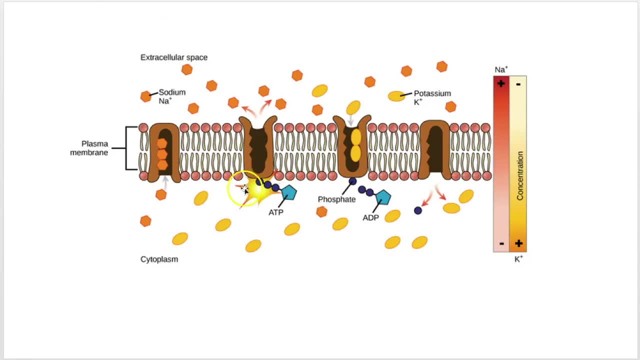 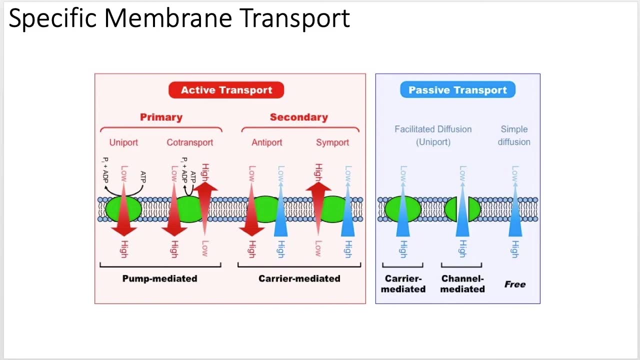 I don't know why, I'm just out of my mind. basically, if I'm going to spend ATP, then it's active transport. Now, there's a bunch of different kinds of this. You can dig real deep into it if you want to. 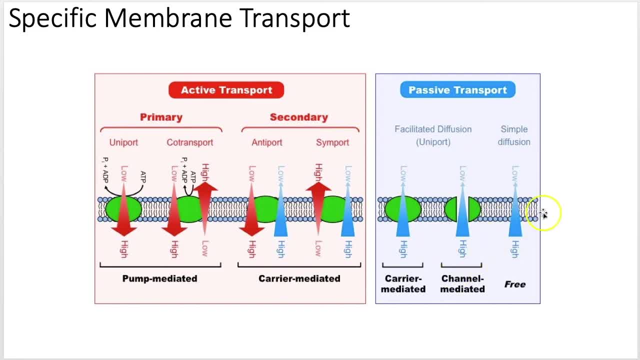 I mean, of course things are passive If they're just going from high to low, Okay. But if I want to go against a gradient, then I got to spend some money, right? So if I want to pump water, water will just flow downhill. 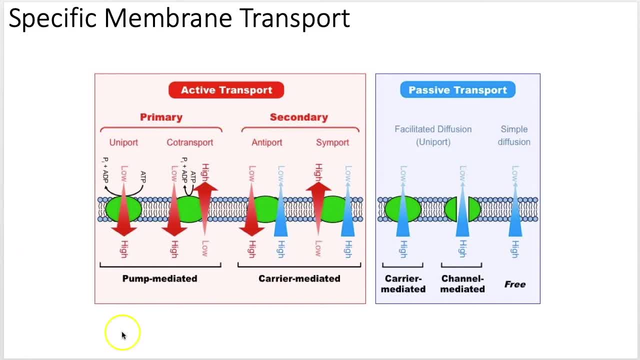 But if I wanted to go uphill I'm going to have to spend some energy And there's lots of different ways you can do that. You can go from high to low. You can go from low to high. Sometimes you can use like carrier mediated would be using something in conjunction. 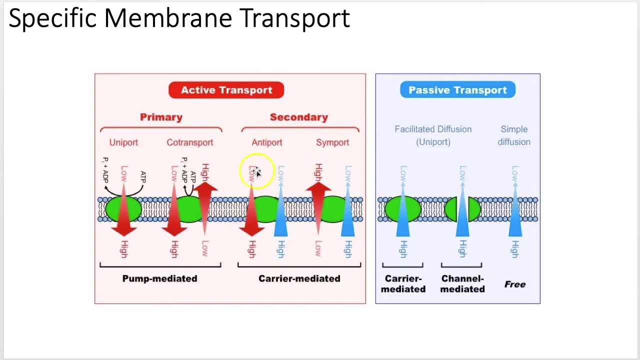 So like you allow something to go from high to low and that allows you to push something the other direction, But basically you're using something in conjunction. Usually, if we're talking about active transport, you're usually depending on primary which. 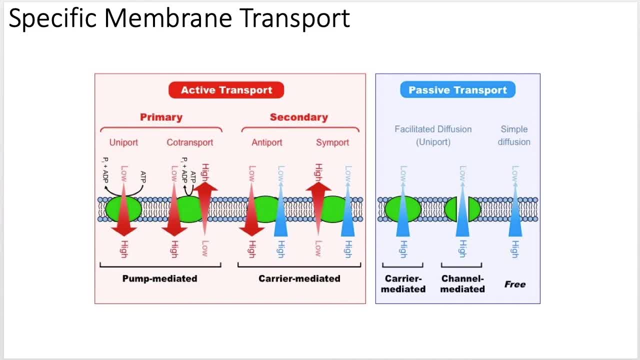 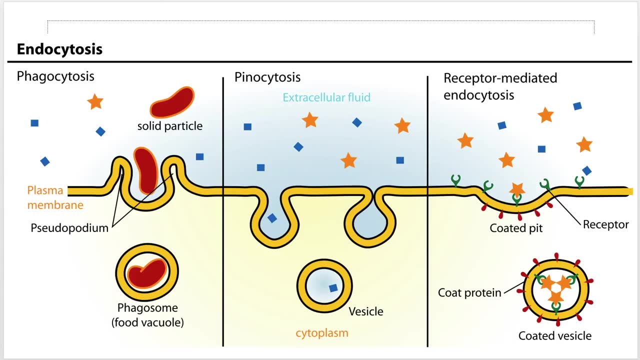 is using ATP to actually power your transporter. Lipid bilayers are super dynamic, Now. not only can they act as scaffolding to put proteins in or whatever, we can have a variety of ways of endocytic pathways or vesicle formation to actually move things around. 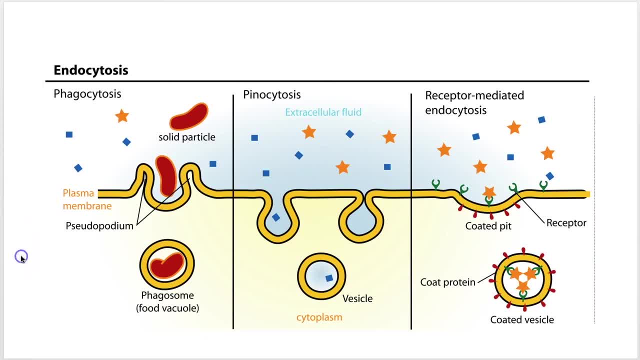 And so this gets talked about a lot- like phagocytosis. People talk about that a lot. There are subcategories of all of these. So this is an entire field of study of how all the different proteins associated with forming, like the pseudopods, the phagosomes, the vesicle formation, 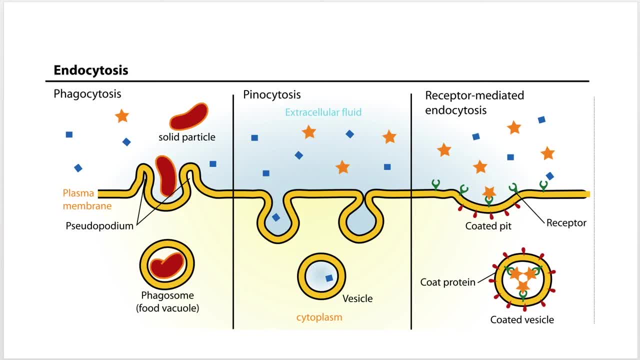 There's like clathrin-coated pits. There's just so many different things associated with this. If you take cell biology, we talk way more about this, But suffice to say your lipid bilayer is incredibly dynamic, which is really really. 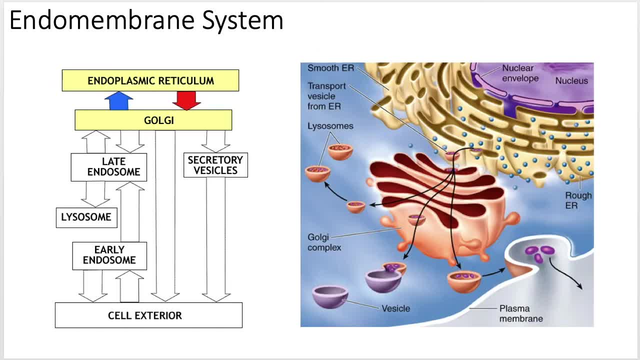 cool And that sort of comes off of the endomembrane system And so that's really cool. Yeah, I think one of the first lectures we had was talking about the endoplasmic reticulum and the Golgi apparatus and what do they do in vesicles. 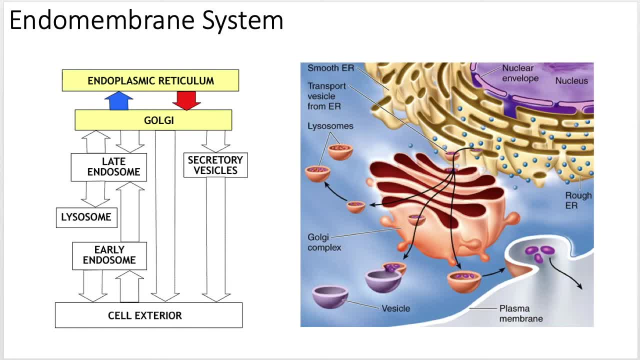 And so those are all lipid bilayers, And so that's kind of what I wanted to end on was just lipid bilayers are so important and they're so ubiquitous that we kind of give them short shrift. I've never used that term before. 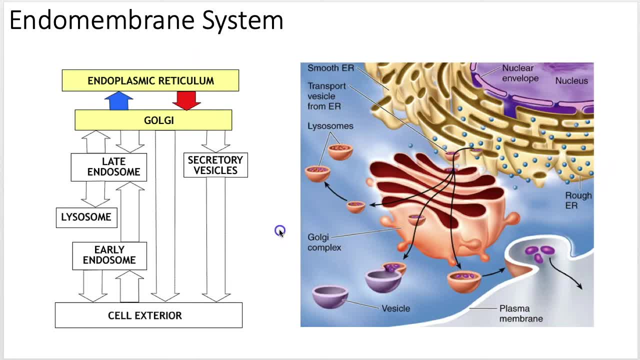 We just kind of forget about them, right, They're just the walls that hold us together, But it's so easy to forget how important those walls actually are And the jobs that they serve, right, And so they're really, really important. 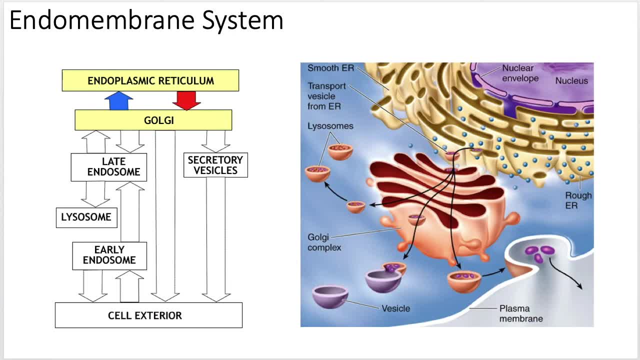 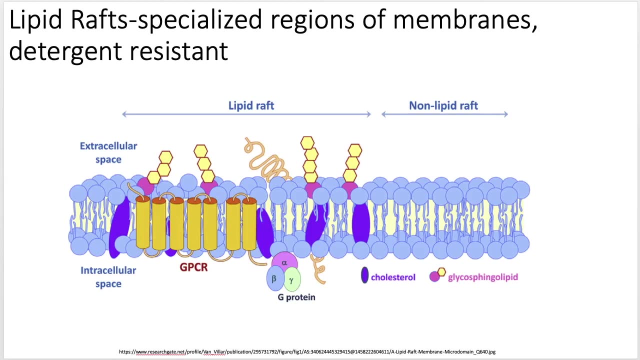 And so that's what I want you to take from that. You didn't think fossil bilayers and membranes and sterols and cholesterol and fatty acids were complicated enough. This very last thing I want to talk about is the idea of lipid raft, So it's a subset of research that goes into, like, the actual structure of fossil bilayers. 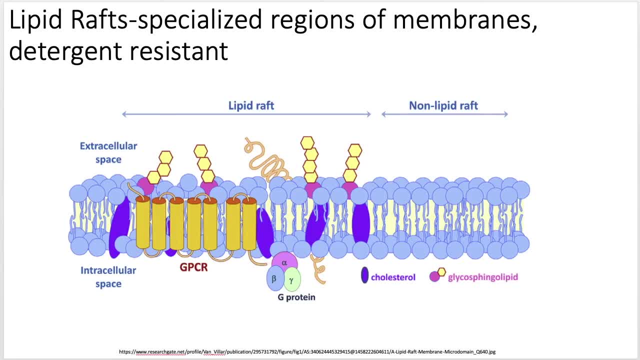 Once again, if you take cell biology, we'll talk about this in more detail. But basically what they noticed was you could take all the lipid bilayers out of a cell and you could throw a detergent at it, So like soap basically, And there were regions that were detergent resistant. 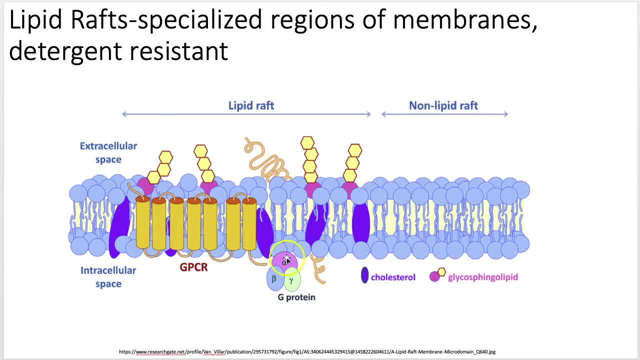 And so they took those and they were trying to figure out what is going on with these, And basically there were these lipid rafts, So they would be full of cholesterols and they'd be really, really dense, And that's where you would see these proteins actually get embedded. 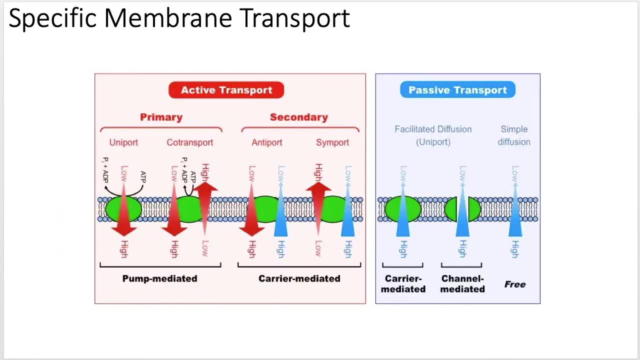 So it's not as simple of like: oh, I just threw the protein in there, You know, it's just sitting in there, It's stuck in there somewhere. Where's this one? Yeah, Just. oh, they're just kind of randomly in there. 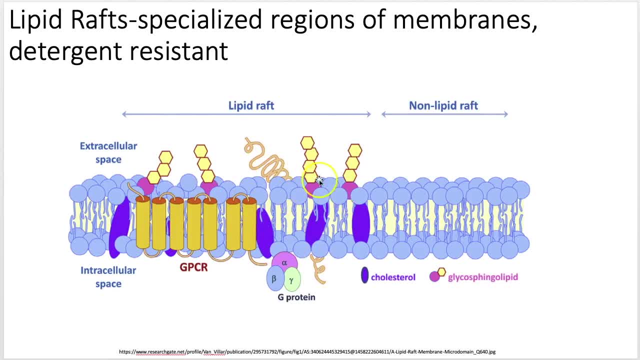 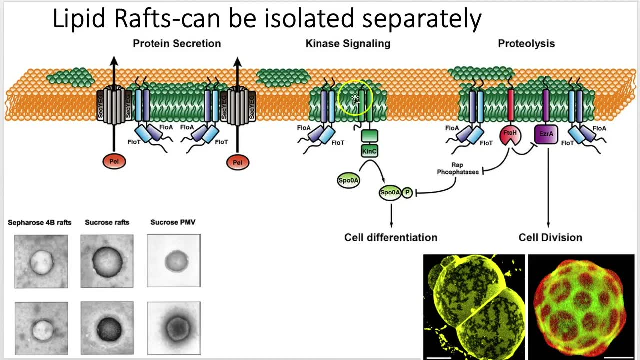 No, they're not Those fluid mosaics. they're actually really complicated. We call those lipid rafts, And what's really really cool is that you can isolate them and separate them out and actually find specific regions that are responsible for specific functions. 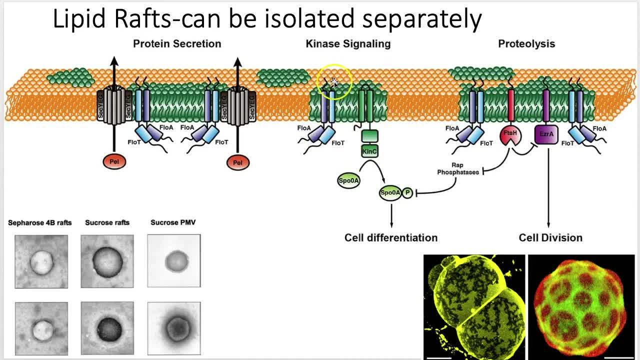 So you could have like a nice signaling kinase pathway that's associated with one lipid raft, or you could have a secretion area, And so it's just one more level of organization to a cell Where you can just see like: oh okay, like cells aren't just these random smatterings. 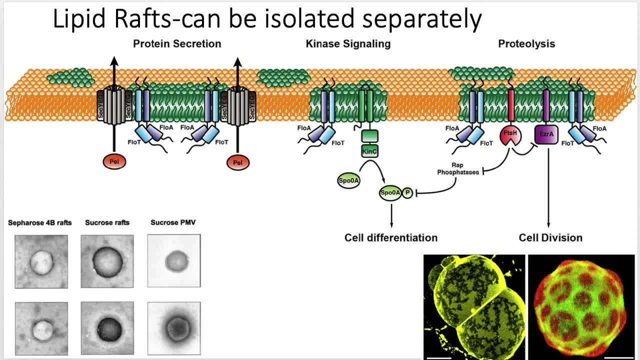 of proteins embedded in a fossil with a bilayer. okay, They are much more complicated than that. I want you to appreciate how complex a cell can actually be. Just think about, like, all the mechanisms that are involved in putting all these proteins and making sure that this region has the right amount of sterols, and it gets really complicated. 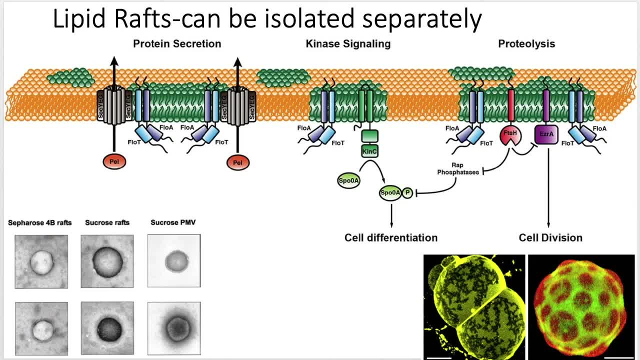 really fast, And I just want you to appreciate that, which I think you do.